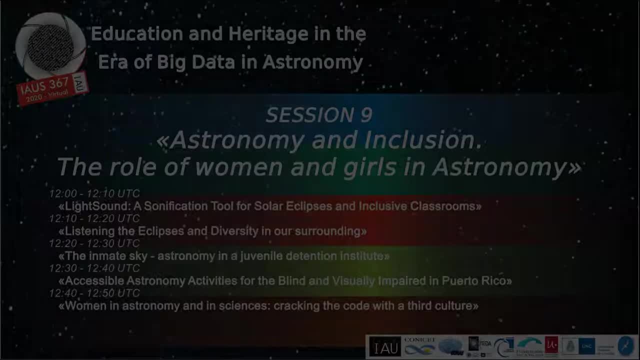 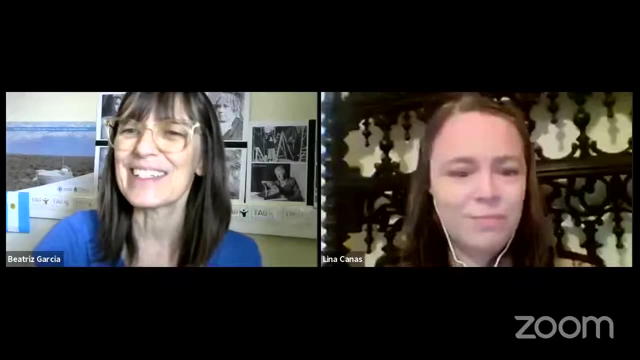 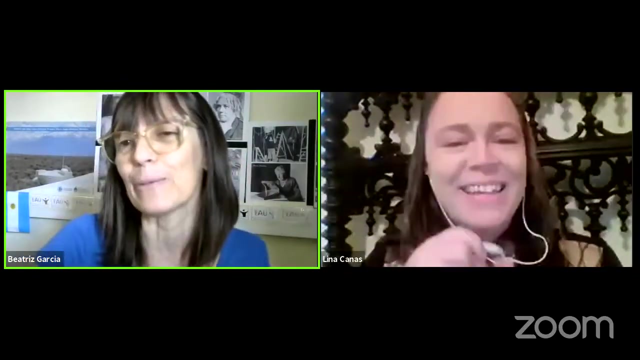 Now it's time to give the space to Lina Canas. She's here. She's the chair of the next session. Sorry, Lina, I gave you the time a bit late, but the topic was very interesting, Very interesting. Yes, Beatriz, thank you so much, Don't worry, It was well worth it. 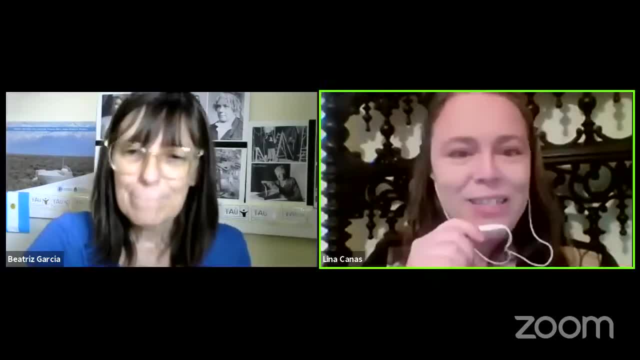 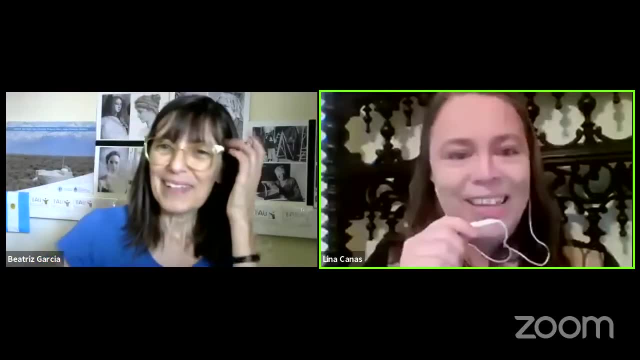 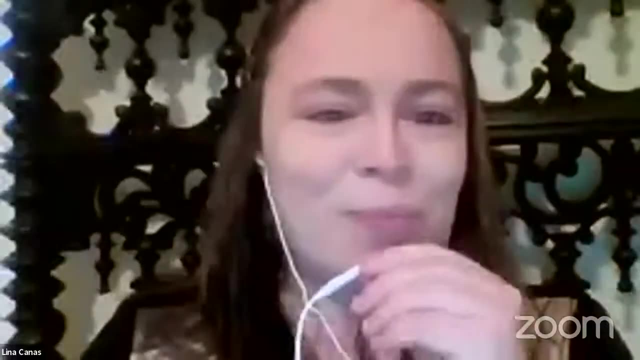 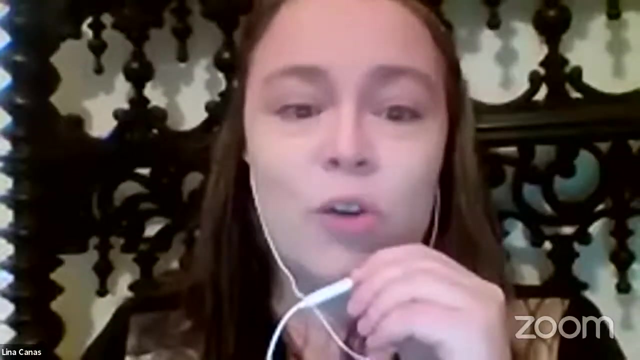 And thank you, Karen. It was an impressive presentation. And thank you, Beatriz, and to all organizers for the incredible symposium that we've been witnessing since Tuesday. The next hour is all yours. Thank you so much. So I wanted to welcome you all to the session nine on astronomy and inclusion: the role of women and girls in astronomy. 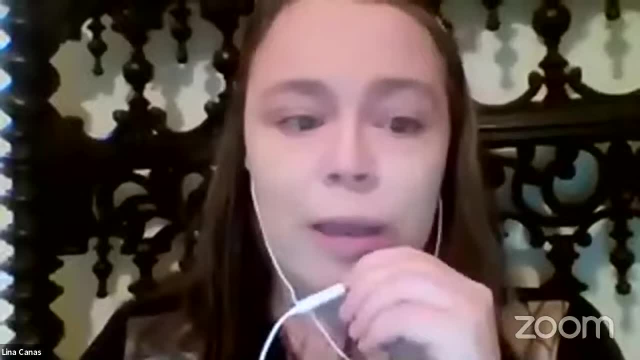 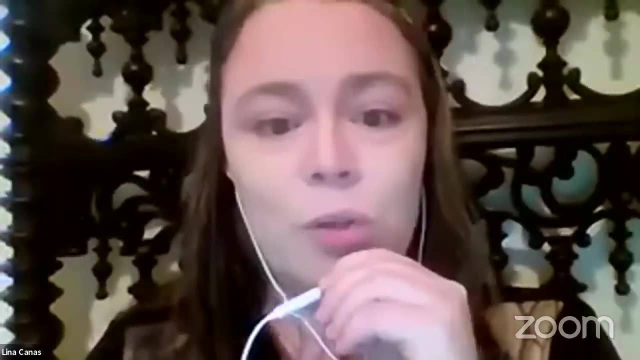 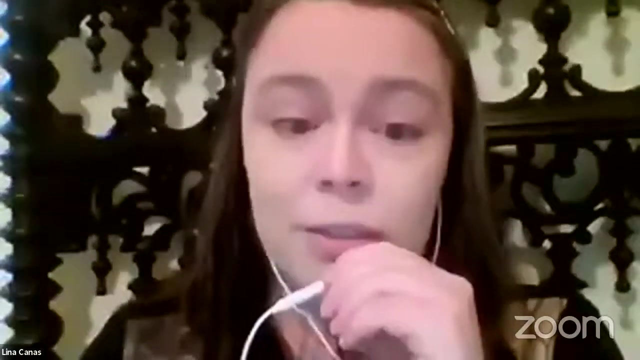 And for the next hour we will have the opportunity to hear very important works and very relevant to our community from our colleagues. Alison, from the US- I believe Alison is already with us, correct? I think she wasn't present at the rehearsal. 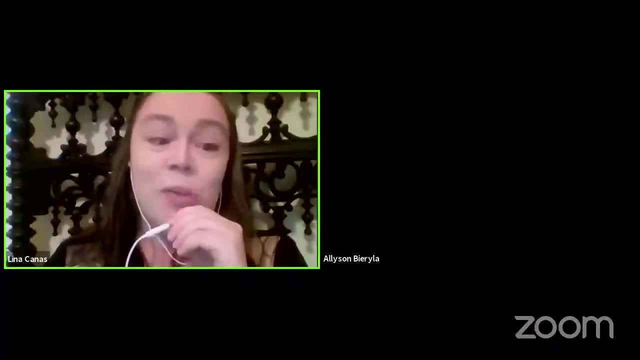 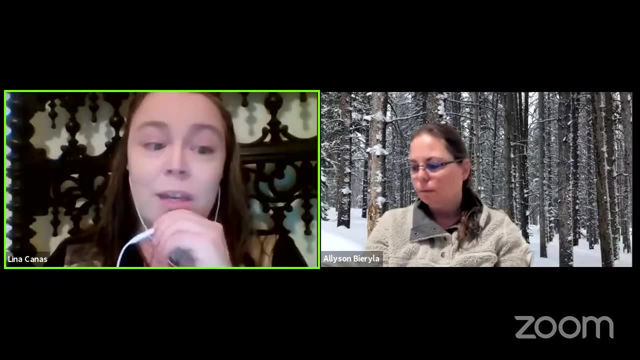 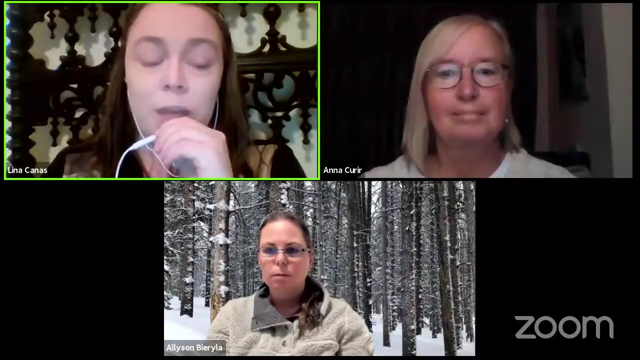 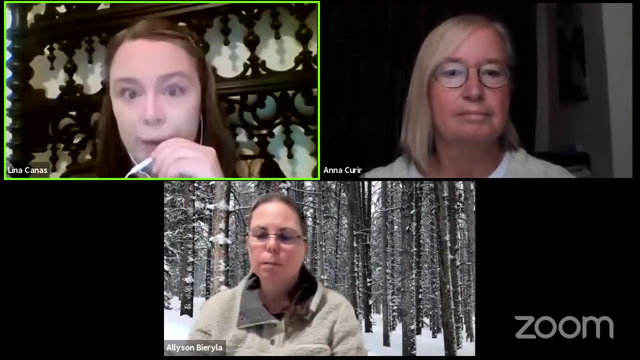 Okay, Hi Alison, And then we will have Paulina, that is reaching us from Chile, Then Silvia from Italy, Gloria from Puerto Rico and Anna Currir from Italy. Each speaker will have 10 minutes and I will notify you when two minutes remain from the end of your talk and at the end of your talk. 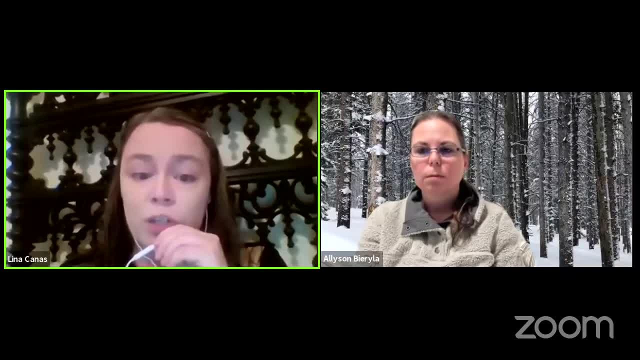 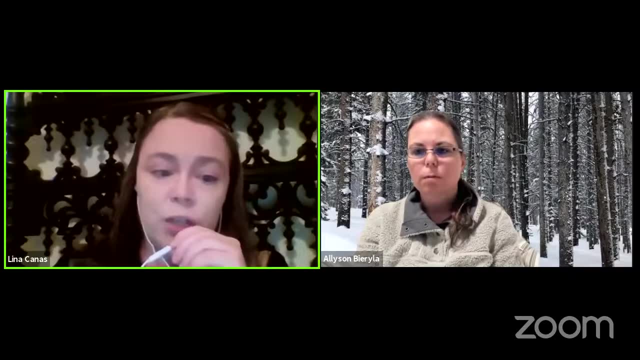 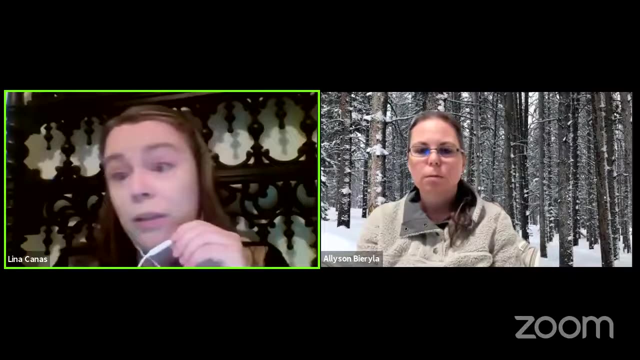 On the end of the five talks, we will have some time for questions from the participants and from all of you, From all the panelists. please place your questions, your comments, in the chat and the Q&A option. So, without further ado, I want to call Alison. 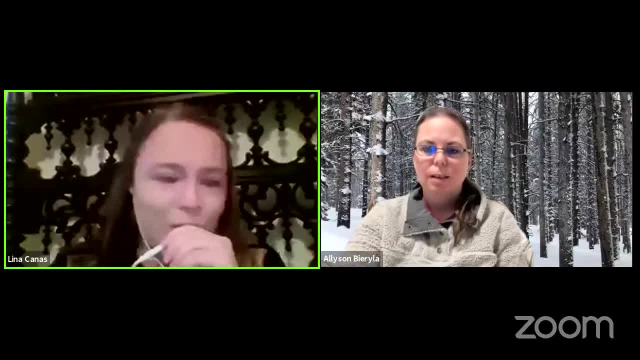 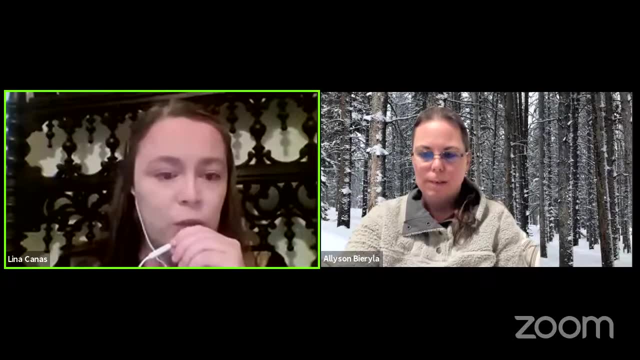 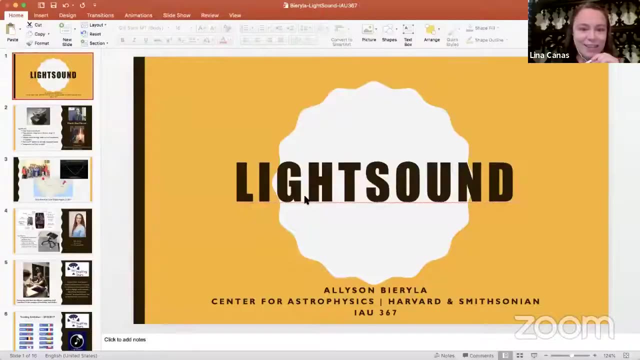 Hi, Alison, Can you turn on- okay, you already have turned on your camera- and also could you share your screen, if that's possible? Yes, Okay, Thank you, Thank you, Okay, Just to test. Okay, perfect. 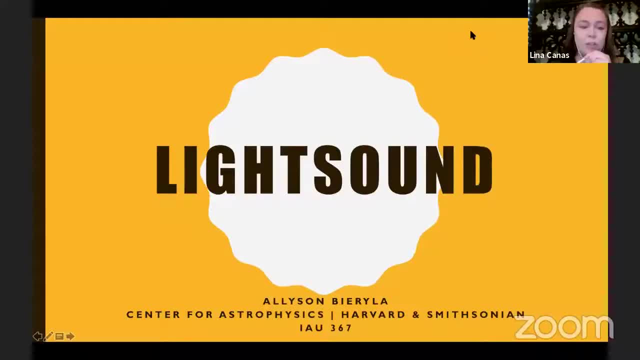 So Alison from Harvard University, USA, and she will present Light Sound, a sonification tool for solar eclipses and inclusive classrooms. Alison, Thank you, Thank you, Great. Yeah, I'm very excited to be here. It's very early on the East Coast of the United States, but I'm happy to be here with everyone. 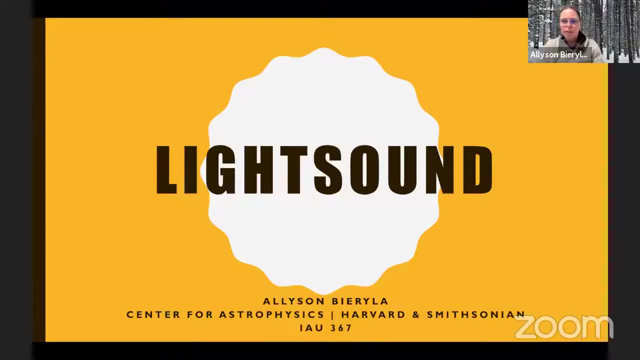 Thank you to Lina, Beatrice and all the organizers for allowing me to speak today. As Lina said, I'm my name is Alison Barilla, I'm from the Center for Astrophysics at Harvard and Smithsonian, and I'm excited to talk about the Light Sound project that I've been working on for a number of years. 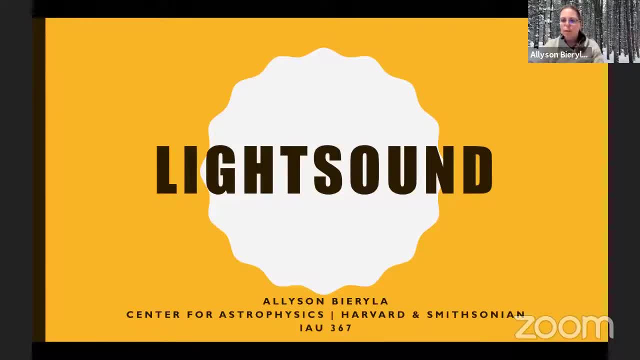 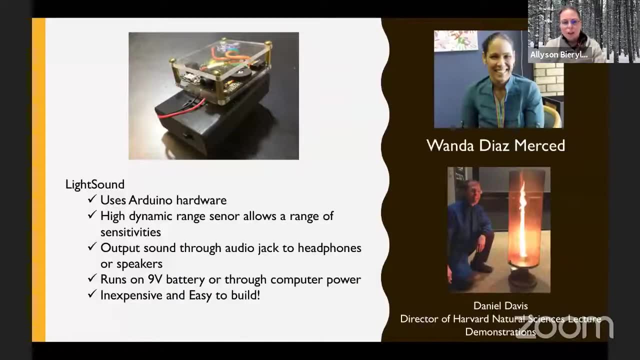 I think I'll try to give a little bit of background about what Light Sound is and kind of what we've done over the past few years and just look toward the future. So I guess, in a nutshell, Light Sound is a sonification device that we developed as an accessibility tool for the blind and visually impaired to as a way to experience a solar eclipse. 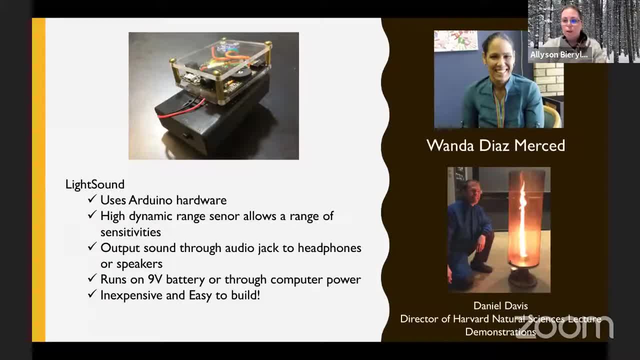 This project and idea kind of came about with our dear, my dear friend and collaborator, Wanda Diaz-Merced, which many of you probably know. Wanda herself is a blind astronomer And she uses sonification as a way to experience solar eclipses. 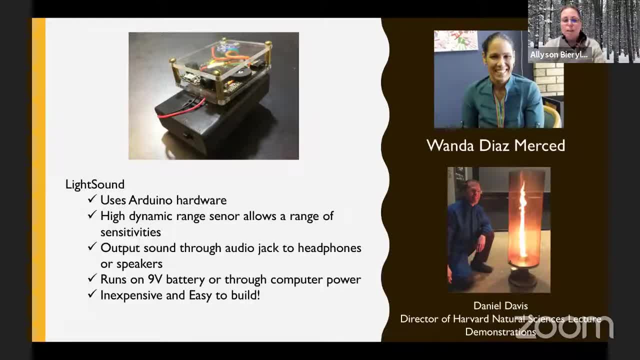 And she uses sonification as a way to experience solar eclipses. And she uses sonification as a way to experience solar eclipses And she uses sonification as a way to do her research. She was at the CFA, the Center for Astrophysics, in 2017 when we kind of came up with this idea and started to develop it. 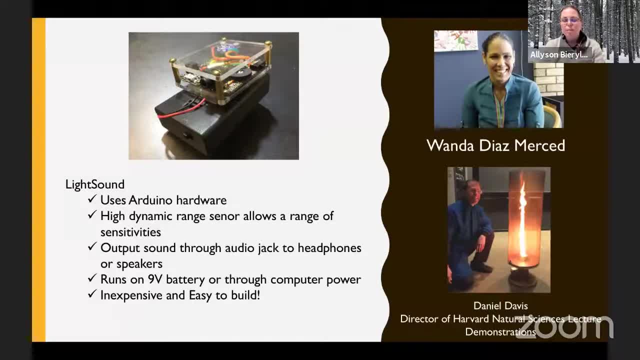 And it was during the Great American North American solar eclipse, And we were discussing ways that we could make the event more inclusive. Wanda was getting ready to head to South Africa to work for the IAU and was going to be working with students that are blind and visually impaired. 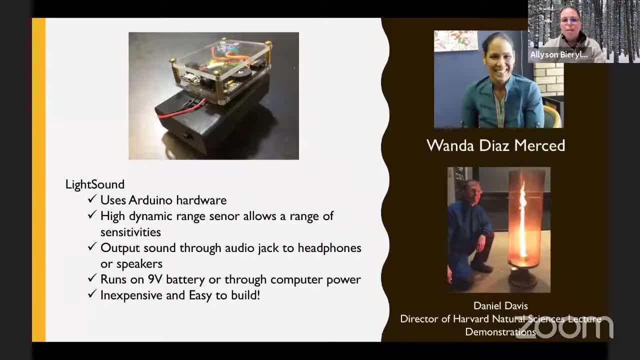 and the whole world was kind of hyped up about this eclipse, and and her students as well, and so we were trying to think of ways that that we can include them, and so in our development stage we were. the main idea here was to make the tool accessible to as many people as possible, so we 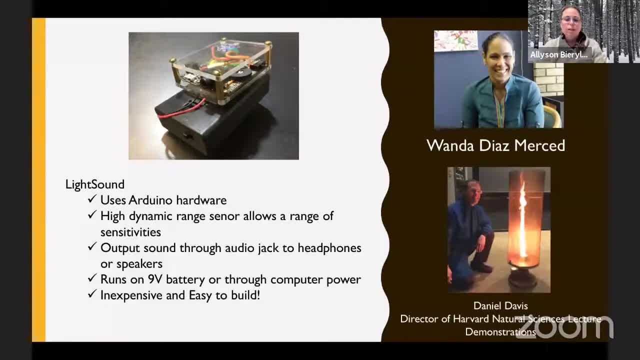 really wanted it to be low cost, easy to reproduce, and so that was our kind of in the back of our mind all all along. so we had this idea and we brought Daniel Davis, who's pictured here as well, into the mix. he's a. he's a the director of lecture demos at Harvard and he's really good at 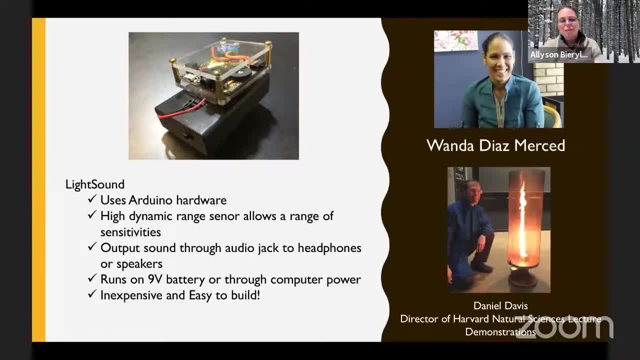 making things appear physically. so we we went to him and he helped develop this, this first prototype. so this is the first version of the light sound and, as I said, it's it's a sonification tool. so the idea is to convert light to sound, and so it's pretty simple in concept. but I'll kind of just walk through the 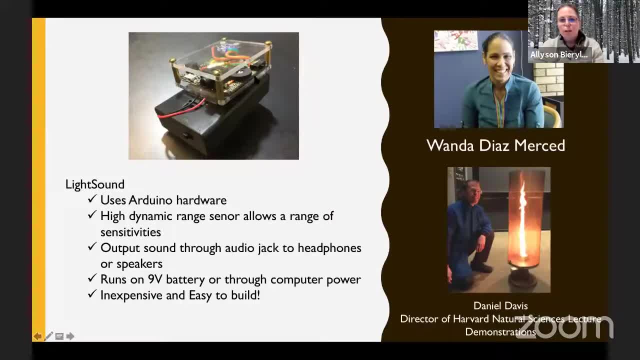 the parts here. this board here is an Arduino board. it's a microcontroller, so you can think of it as a small computer where you can upload a simple program to it. you can also attach different components to it. so this is the microcontroller board we have over here. this. 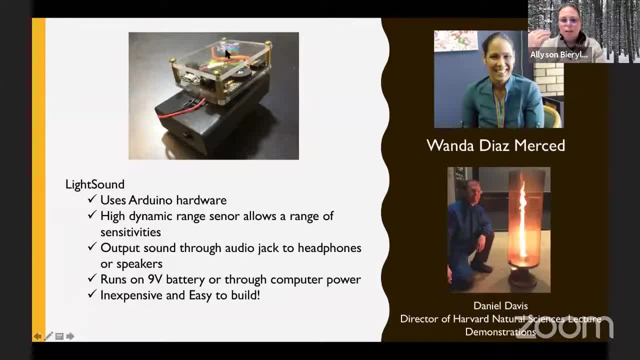 high dynamic range light sensor so it can accept very bright light, also works in very low light situations and, as many of you probably know, also the. a total eclipse is something similar to about the brightness of a full moon, so we need something full, full sunlight and also low light like a full moon. there's also 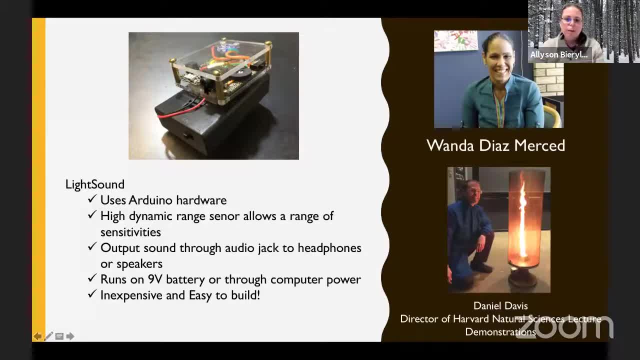 an audio output here, so this is your speaker output. you can attach the headphones, you can attach the speakers. we have a port here that goes to a computer, so you can also charge the device that way, or you can connect to a computer, if you have one, and collect data. 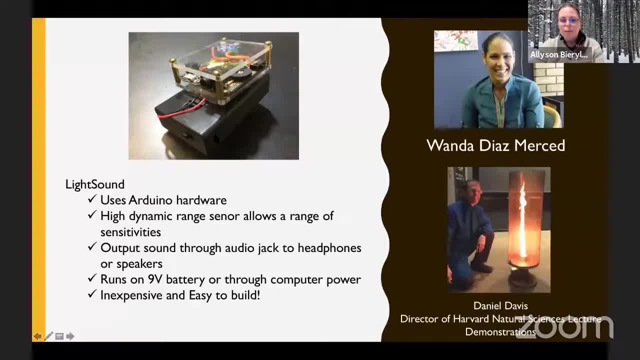 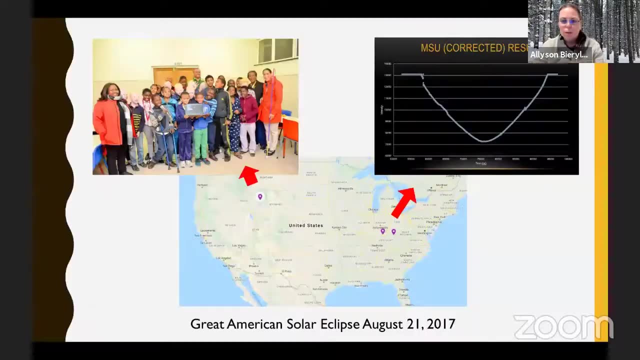 now it's not required that you have a computer. we also have a battery pack that runs on a nine volt. so that's the idea: bright light is mapped to to a high sound, high pitch, and then low light to a lower pitch. so we had our, our prototype. so in 2017 I was going to be here. 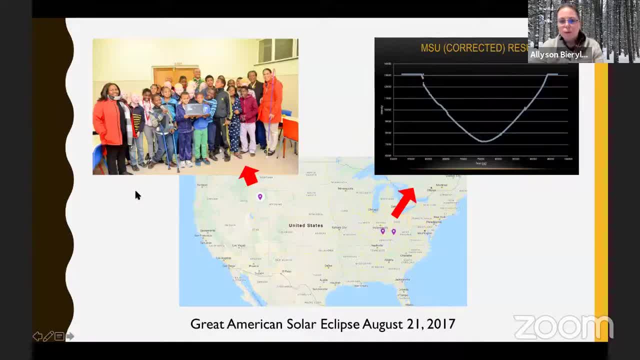 I was going to start the day two days before the parks and whole Wyoming um Wanda's- pictured here with her students, south Africa. so I um streamed the event on YouTube and Wanda and her students were able to listen in as as did others around the world, and we also had two devices in Kentucky. 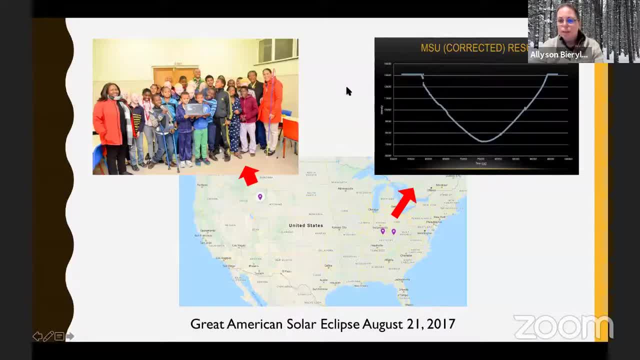 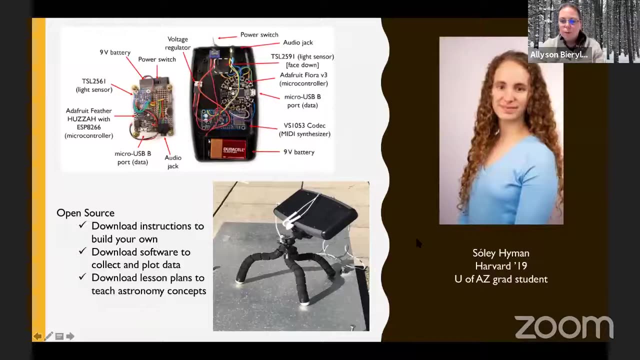 this is data that was collected from Moorhead State University, so it was a great success. we had our prototype and and things worked, so that was very exciting. there's a lot to improve on, So in 2018, Soleil Hyman joined our group. She was a Harvard. 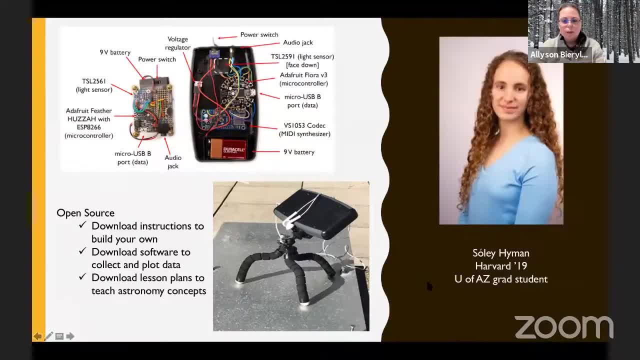 undergraduate at the time. She's now a University of Arizona graduate student and she really helped a lot with this project. She worked on the redesign of the light sound device. So here's the first version picture on the left and then we have the more updated version here on the right. So a couple. 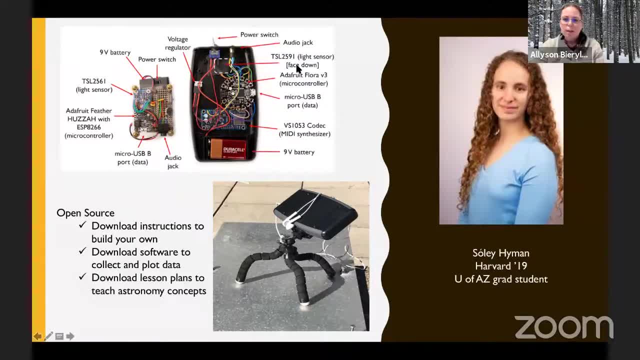 key changes were made. We have a new light sensor now, so it's just a slightly better light sensor that we found, So it helped with the dynamic range a little bit. We have a new microcontroller board that works with MIDI technology, So we have this MIDI synthesizer here, So the 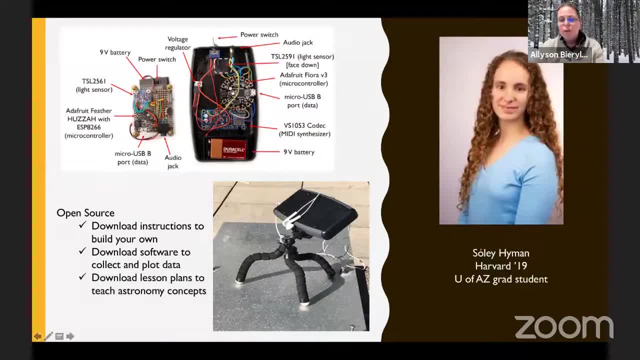 key part here is we really wanted to improve the quality of the sound and to do that with MIDI. you can attach different instruments to different sounds and it really helps the sound profile quite a bit. Also note that Soleil while she studies astronomy. 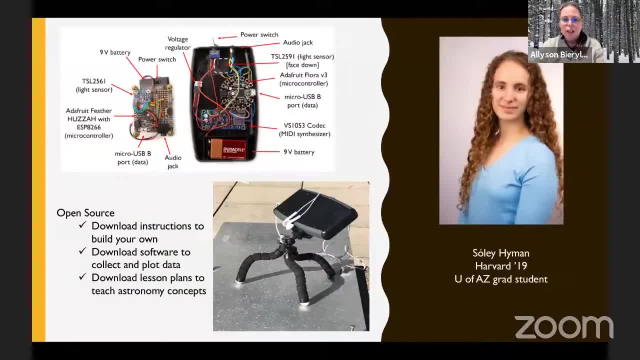 and physics. she is also a musician, so that helped a lot. And then, of course, you can see, here we have a nice custom case which just enclosed everything nicely. So Soleil also worked on really documenting the data. We really want everything to be open source because, as we said, we want to. 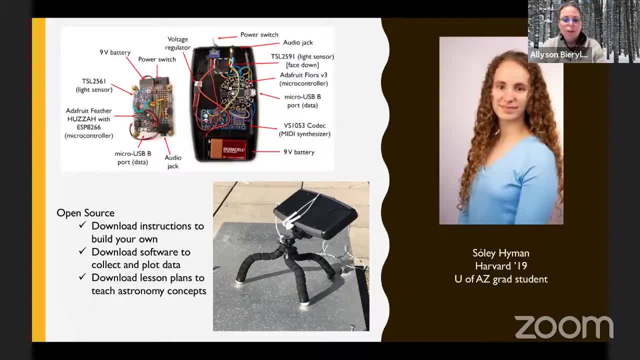 make this as accessible to as many people as possible. So we have all the instructions on how to build all the components, you know, diagrams on how to wire things, how to upload the data to the device, As well as just the code that runs it. So they also developed. 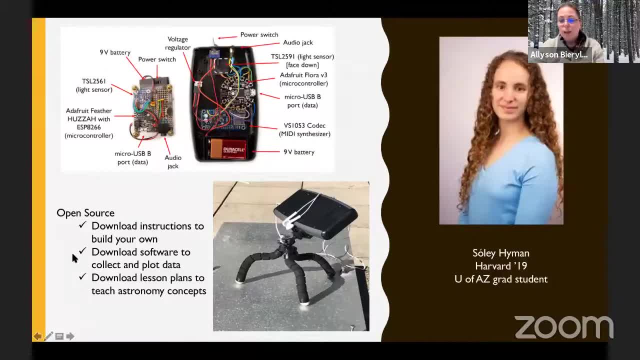 a couple Python scripts that allow you to collect and plot data easily, And that was really nice. And then we started working on some lesson plans, So we wanted to adapt this to classroom and outreach programs as well, Not just solar Eclipses. Some of you probably know about the Inspir Fucking. 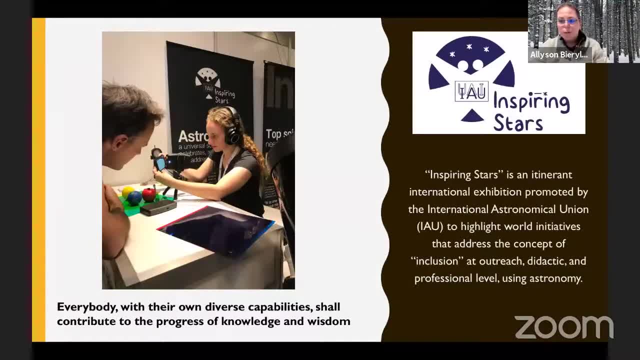 Actress protocol at the beginning of this presentation. but what I want to nada spilled the deceptive 列, a small focus here. So today I want to Start architecture here a little bit. April 1st's And this is the. so we have all the databases and codes that we wrote here in the description below, And then we want to develop a newsletter that시면 a little bit as grey, predominant in terms of the calling of almost 70 after day timings and definitions. We created some�s to take some data in relation to earth and the red filet science, so we wanted to rough andhando. 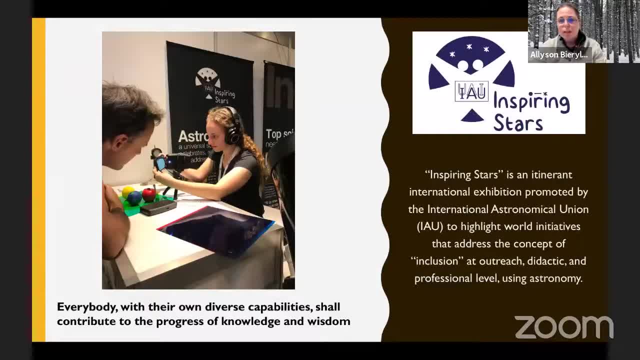 The Inspiring Stars exhibit. we were really excited to be part of this And this is a picture here at the Vienna IAU meeting. This is just Soleil demonstrating the device. We were happy so. Inspiring Stars is an international traveling exhibit that highlights some inclusion and accessibility tools. 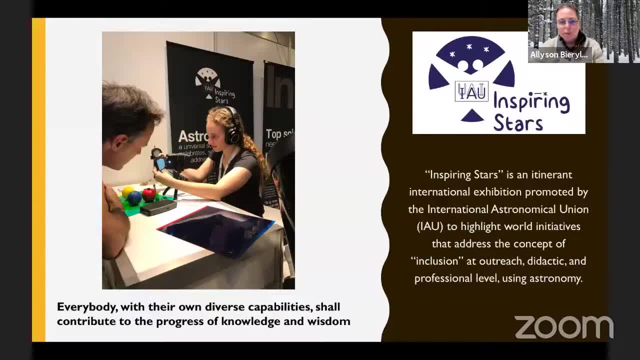 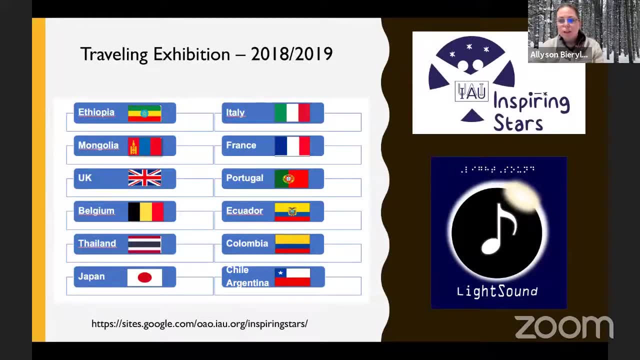 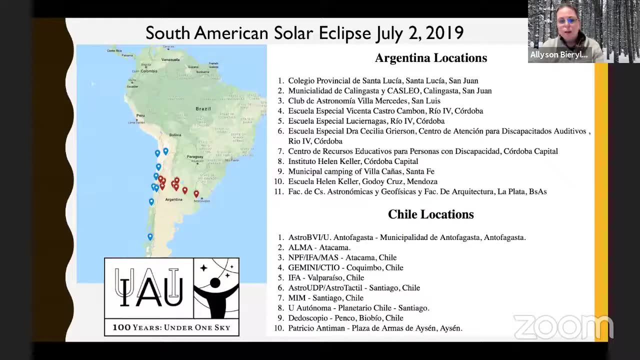 We're one of the devices and tools in that exhibit, so we're very excited to be part of that. The exhibit traveled to many countries throughout 2018 and 2019.. And then in 2019, we were given an IAU grant to build and distribute 20 of these devices for the South American solar eclipse. 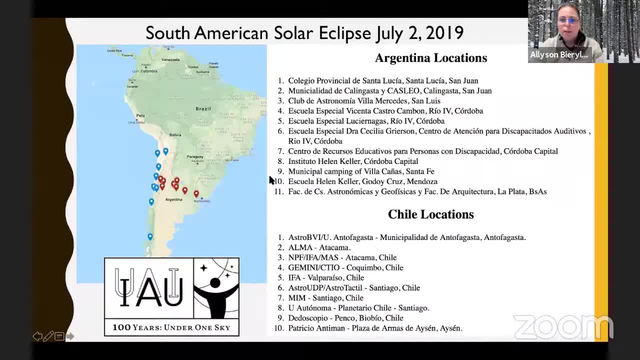 So Beatriz Garcia and her group led the effort to build in Argentina, And so they built and distributed the devices here across the path. And then Soleil and I built and sent the devices for the Chilean locations, And Erika Lab and Paulina, who's going to be speaking next, were key collaborators in those areas. 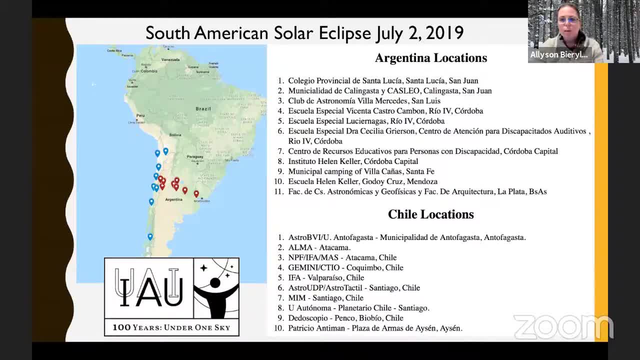 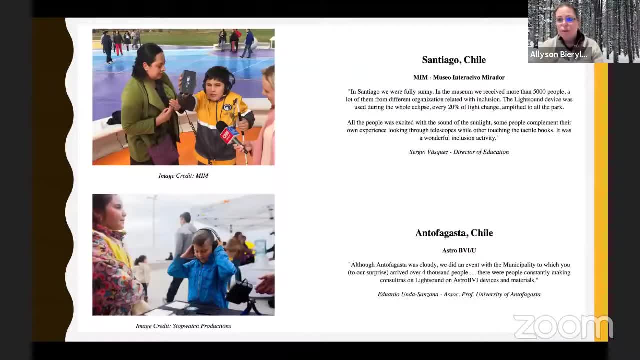 And Paulina is going to talk a little bit more about the actual South American eclipses and some of the development that went on in Chile, And I was just thrilled. Unfortunately I didn't get to physically go there. I was hoping to be with you this week. 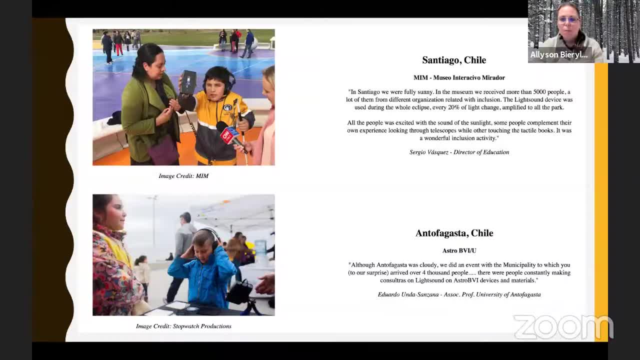 But I didn't. I was just thrilled. Unfortunately, I didn't get to physically go there. I was hoping to be with you this week, But um Covid right. But, mmm, I was just thrilled to see some of the photos and hear some of the reaction from people that were at these events. come back. 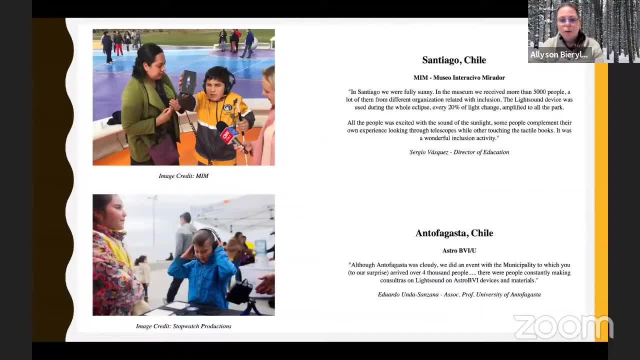 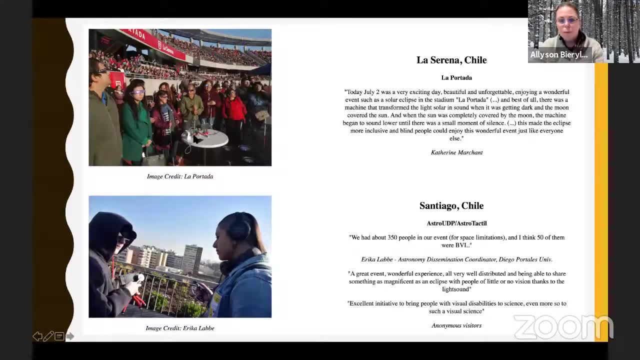 It was. it's really rewarding project. I'll note that one of the things – this picture especially – I think, shows it. You know, there's many, many thousands of people in this picture, But there's one light sound device here on the table and it's connected to a speaker. 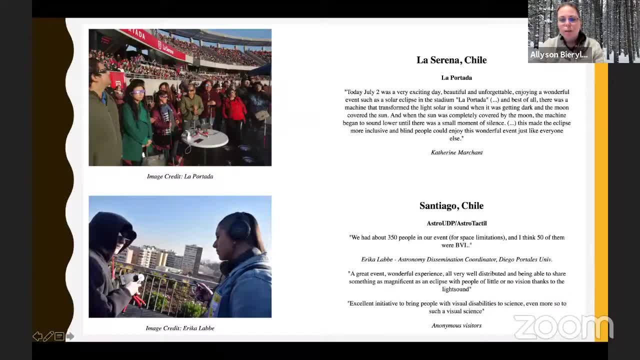 And, And, and. so the device costs about $70 to build and the impact from that one device can impact many, many people. So that's- Sorry, Alison, two minutes, Thank you, thank you. So that's the key here is just you're able to impact. 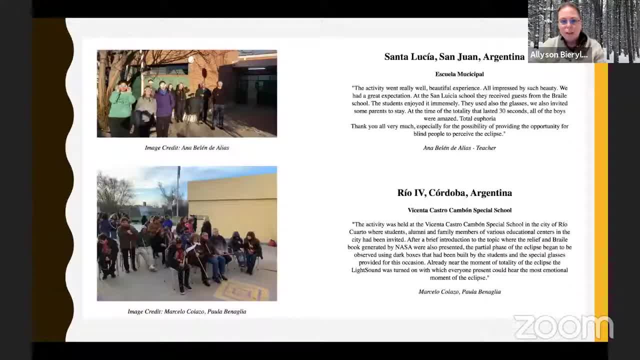 many people with one device. One other thing is that we were able to translate all the documentation to Spanish as part of this project, So that's what we hope going forward: that we can work on even more translation to other languages. I'll just point out here in 2019,. 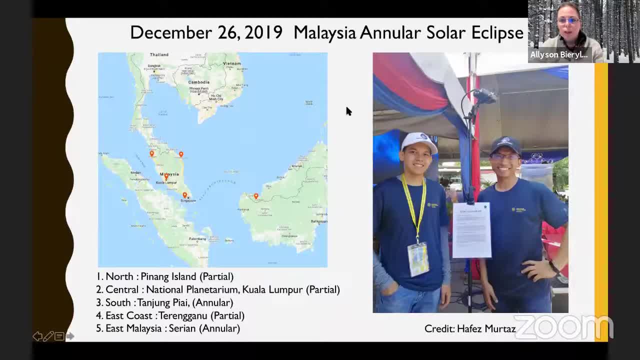 there was another. there was an annular eclipse in Malaysia and a group led by Hafei Murtaz built five devices across Malaysia. I wasn't directly part of this, but they were in contact all along the way and it was a successful event. 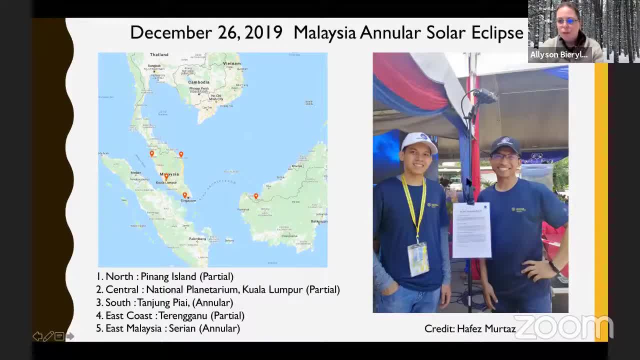 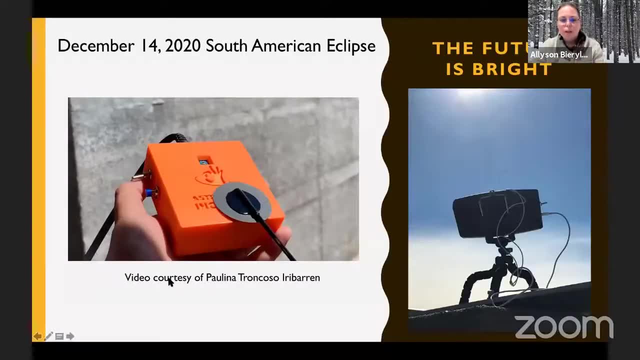 They used the documentation that we provided and you can see here again. one device connected to a speaker can impact and that make a entire event accessible. So I just want to play you a quick sound clip. So this device is the same device I've been talking about. 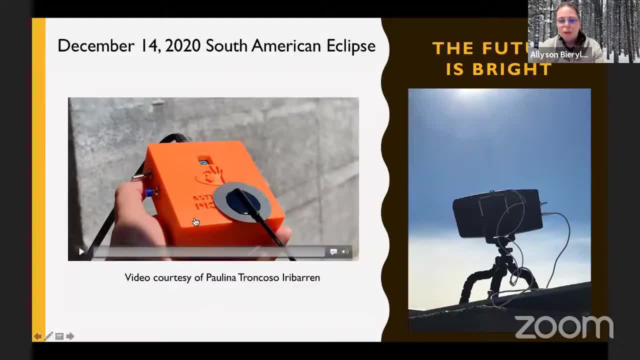 but this is a video courtesy of Paulina and they have their own custom cases that they make, So I'll- hopefully you can hear this. I'm going to turn up my sound, So this is the high pitch flute level, And then this is the simulation of the eclipse. 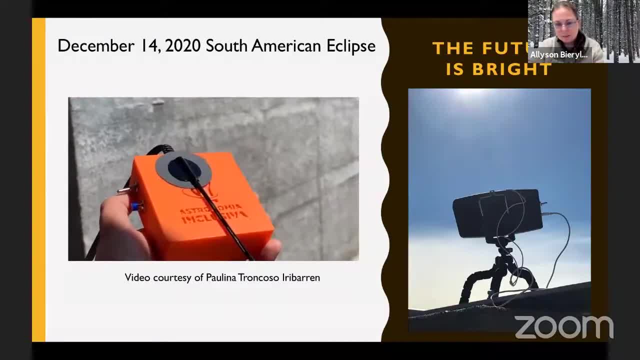 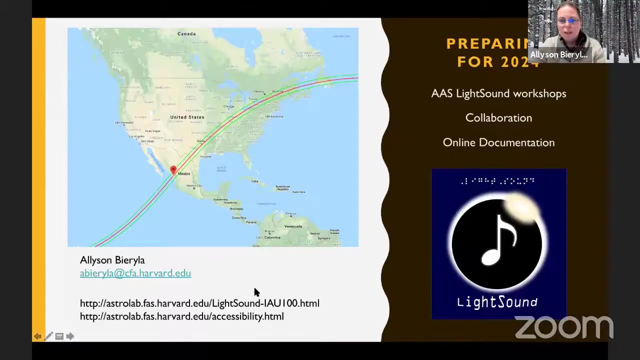 At the low level it gets like very low. you could hear the, the change. obviously an eclipse takes, takes time, so this is a sped up version, but just to give you an idea of what the sound is like. um, and so really i just you know, we're starting to think about 2024 in the in in north america. so the eclipse last time went. 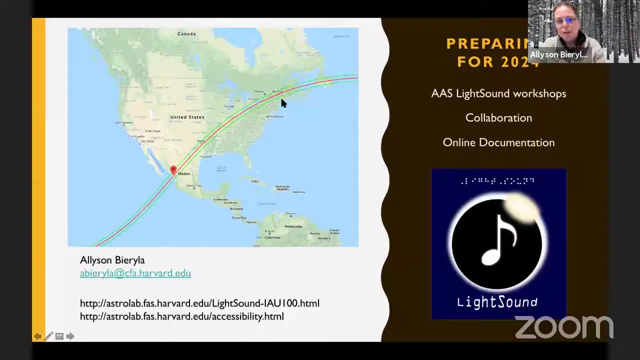 from like northwest down, and here we're going, you know, up, uh. so i don't know where i'll be along this path, but i'm definitely thinking about it. uh, weather is going to be a key, um. so here's the, the links down here and my email to get documentation and reach out. but we've developed a workshop, a 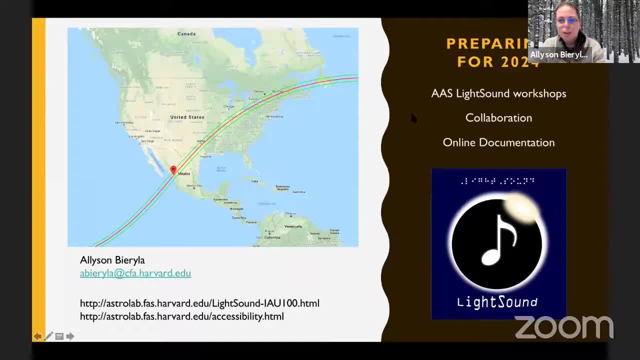 two-day workshop that we debuted at the american astronomical society meeting in hawaii last january and it's to build and just build and use the device. and we hope to run more of these workshops at the double ass, other other conferences, um to get word out and to to collaborate with others, because, uh, we can't. 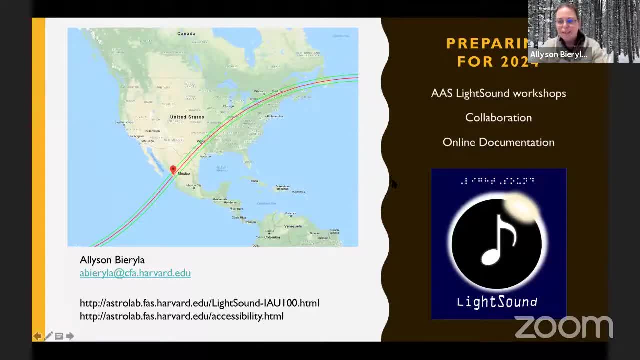 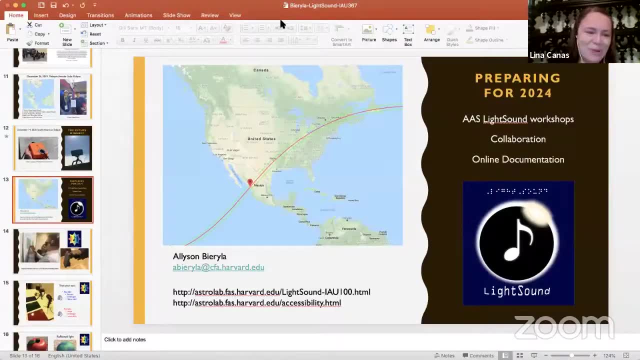 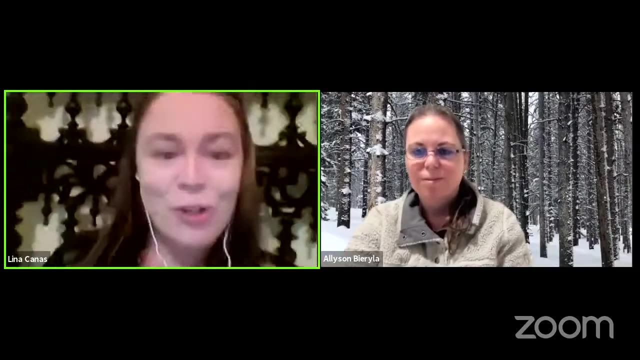 do it alone. so, um, thank you for listening and, uh, thank you so much, allison. yep, no problem, thank you so much. it's always a pleasure to hear more about lights on accomplishments, and it's also a pleasure to be able to collaborate with you, and we are fortunate to have you in a direct collaboration with so many with inspiring stars. 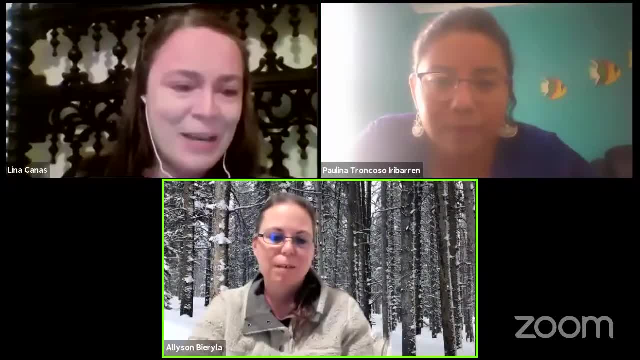 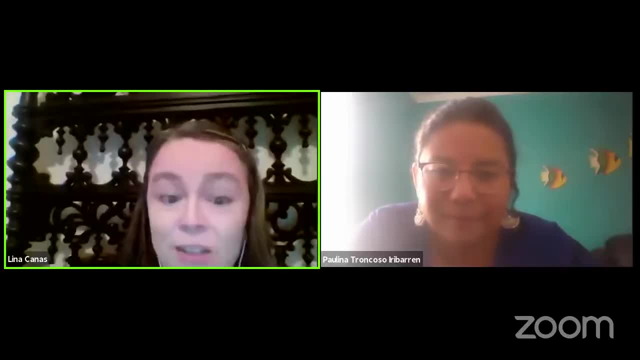 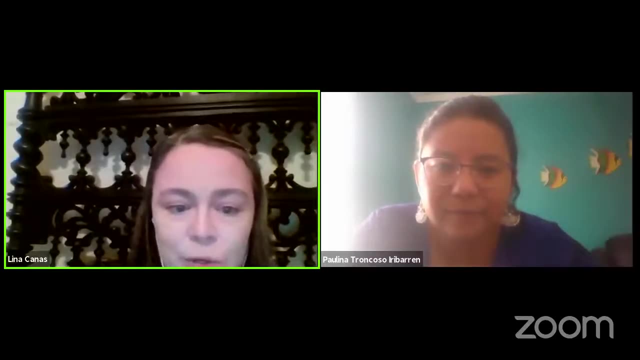 and other projects around the world. thank you, allison, thank you, um, and now i would like to call paulina, paulina troncoso uh, from the universidad central de chile, um, and she will talk about listening the eclipses and diversity in our surrounding. paulina, thank you so much for. 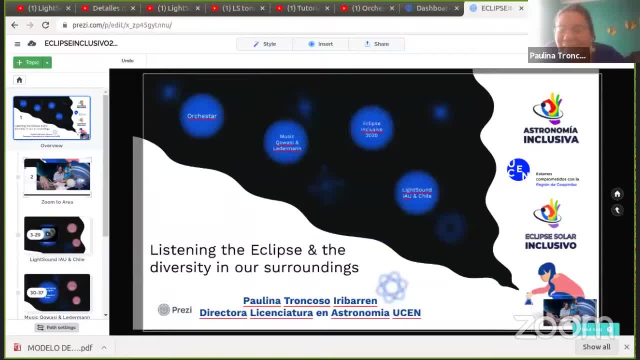 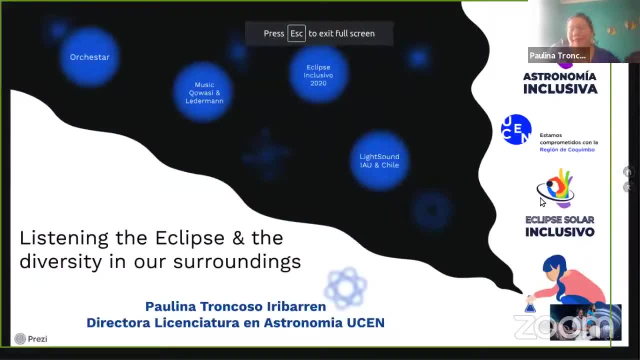 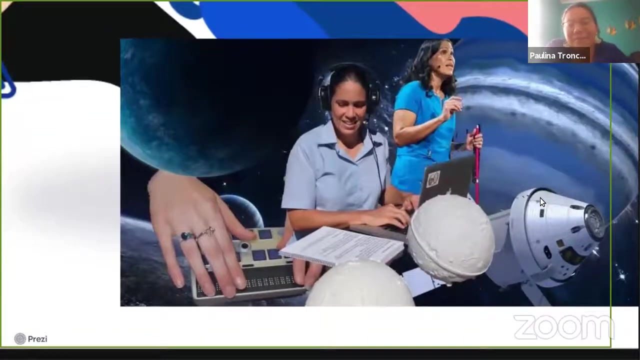 being with us. hello, hello, uh. can you see my presentation? yes, we can see your presentation, yes. so yeah, as i listen, say we were like sort of a boost with all this motivation for with the light sound, and we decided to start building it here. so this experiment that we are doing here, i would say, at least for me, is driven and motivated for. 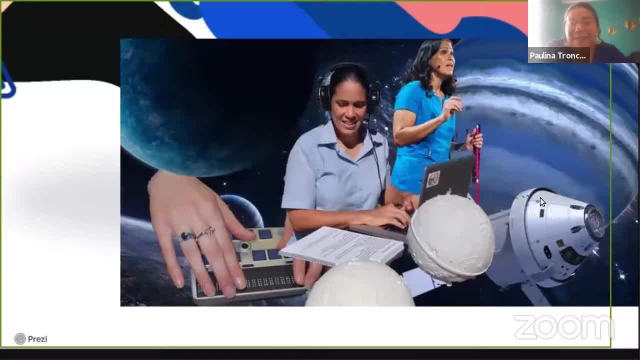 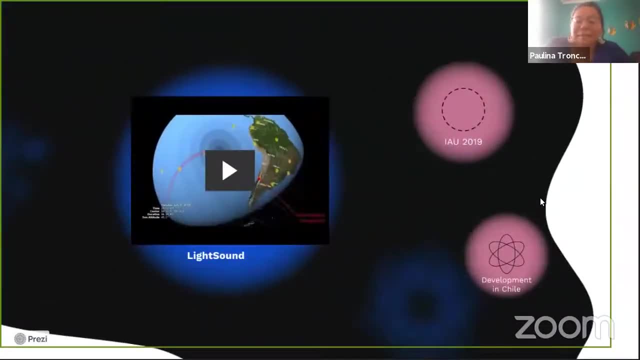 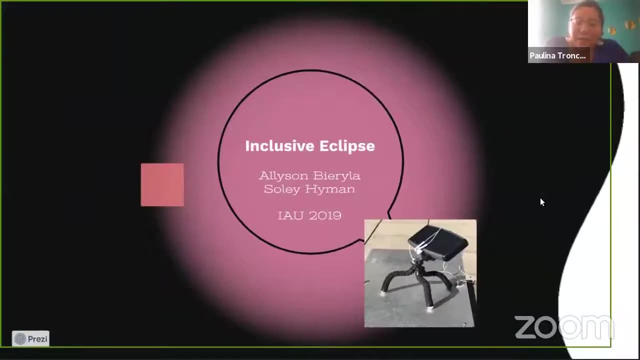 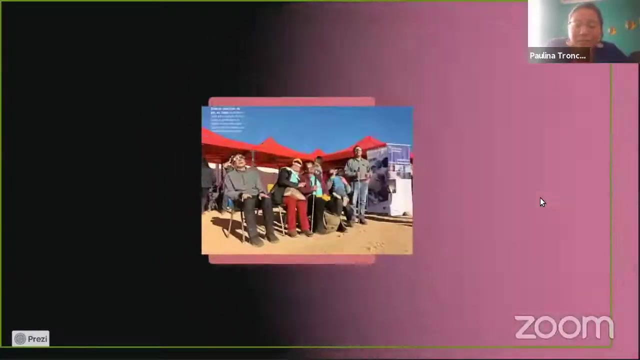 my dear friend wanda, when she brought the first devices here in 2018 and later. while this was a little bit of a change in her life, she was, let's say, changing when changing because she motivated even more people when we had this record of the eclipse and, as allison say, they ship us 12 devices. 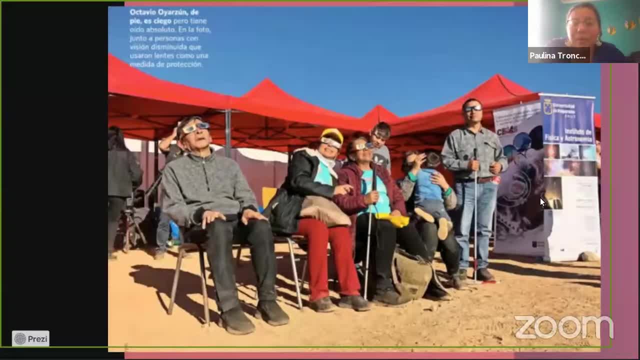 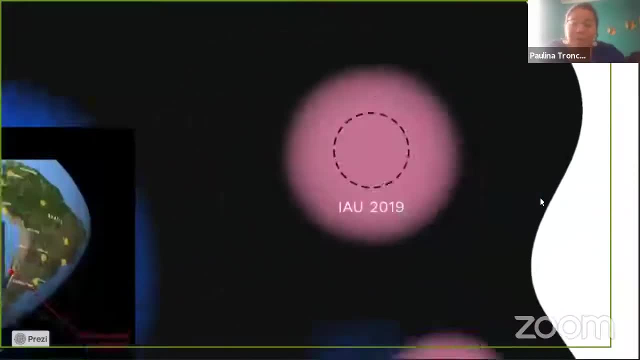 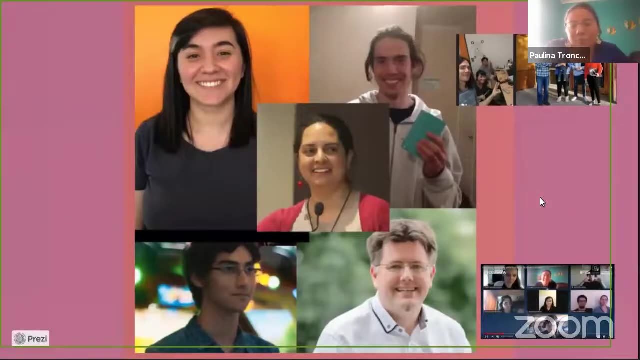 along chile and we were able to enjoy it in an inclusive way for first time- the eclipse here in chile- and we got a lot of people involved. the point here was that we started working with the main group, these five persons that are in the middle, a little bit before the the eclipse, because, uh, with 12 devices, let's say we were short because 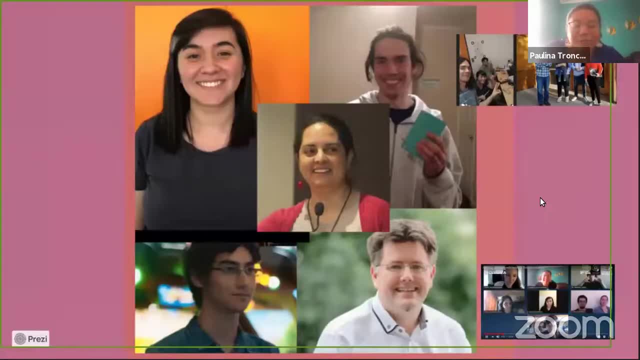 everyone wanted to have it. we circulate information in social networks that we will transmit the, the, the sound of eclipse, and the media was just reacting like very active and they started routing to us and the the two kids, javier and carlos, that you see on top. 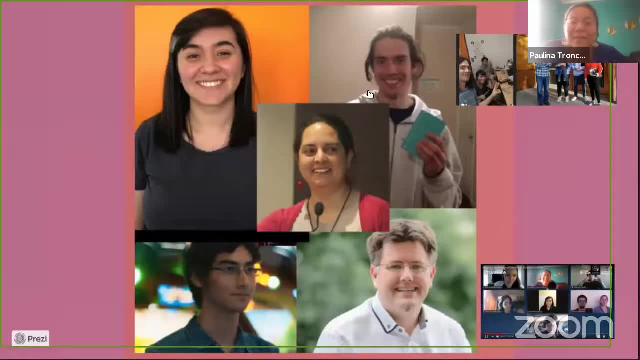 were my students and this moment and and they started playing how to do it. also, henry, the student of erica. and well, here's my husband, he's an astro engineering and we started, like as a family, all of us trying to how, to see how we can reproduce it and follow the instruction that 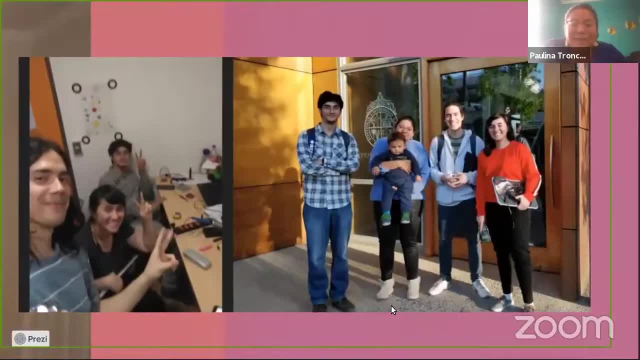 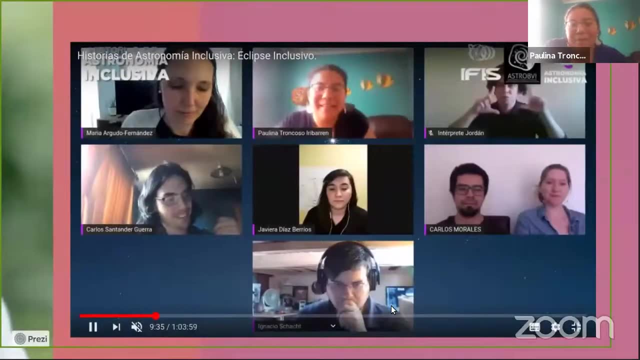 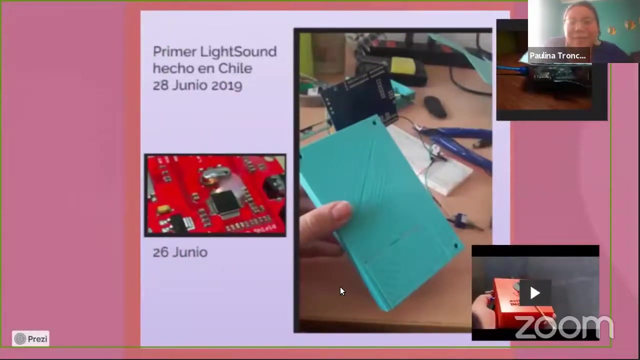 alison just gave, and we had very nice uh evenings playing various things. and finally, this year this team even grew up a bit more, with these two persons here that are in temuco also building light sounds, and ignacio that was also joining the, the core team. so, uh, i have to say we succeed on the 28th of june of last year's- few days really. 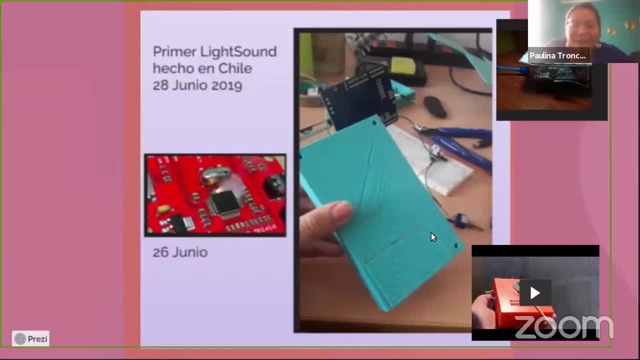 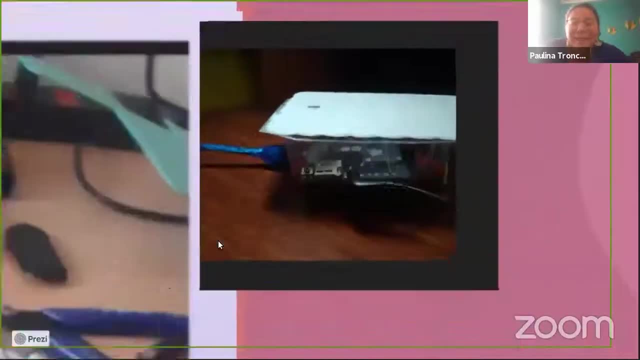 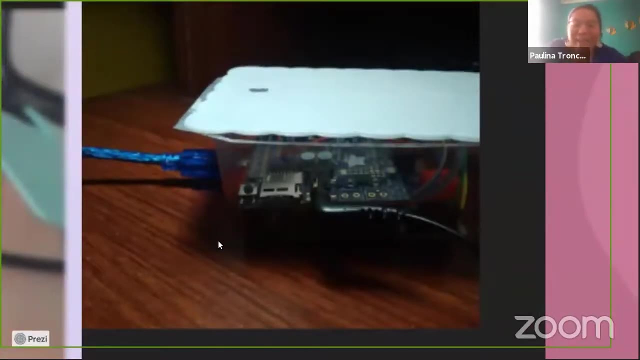 before the eclipse, with this case that we create this science case. but on the 26th we were at this level just burning things, and the first case that we had was this one. we could not find the same case that alison had, and we did not have a way how to acquire someone. 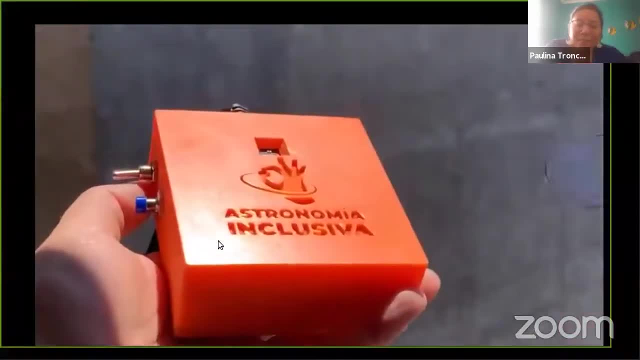 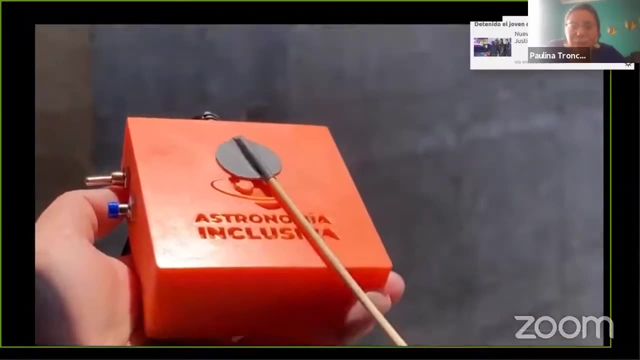 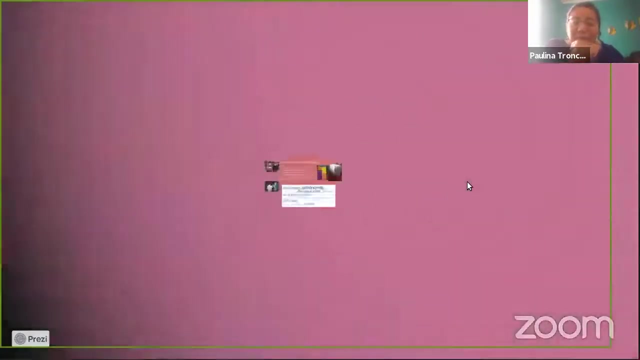 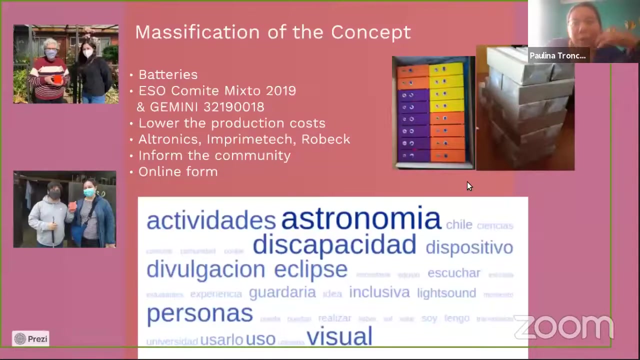 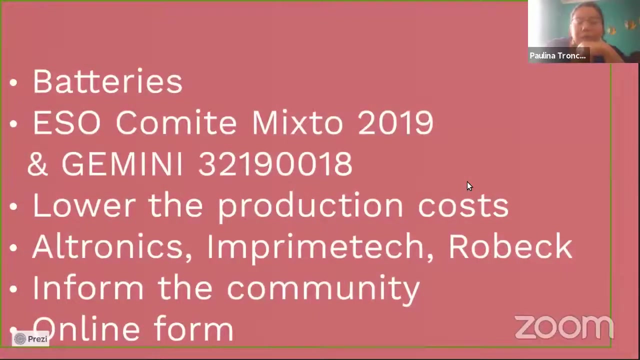 here. so we bring one in 3d and well, this video i will not play, because exactly what just alison showed to you and we were going with this development. so we say, what do we do for next year? and we, we point to the massification of this concept and we say: how can we do it? so the first thing that we 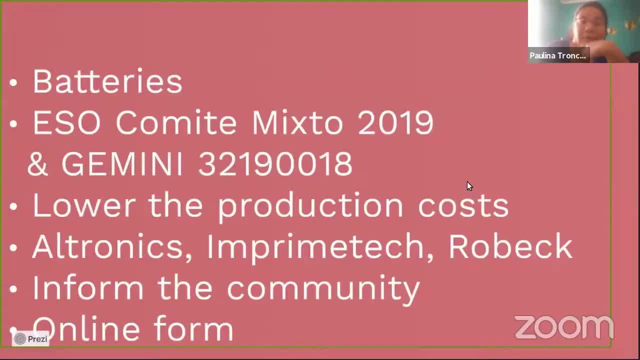 did? we say, okay, we want to reuse the battery of the laptops to fit the devices. so, and how do we plan to do this? we start collecting the bad batteries from the people who wanted to donate it to the project. we applied to two funds and we got both very happy about it. and with this money, we say okay. 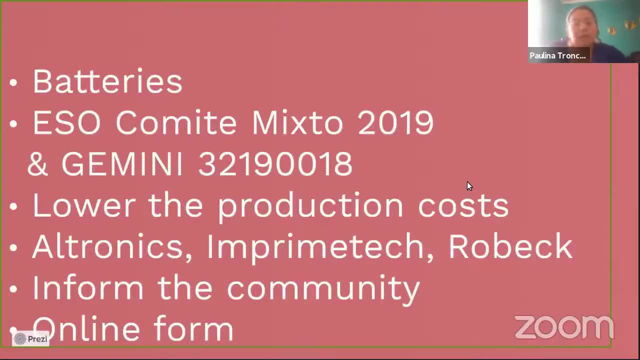 how do we lower the production cost so that we can um distribute as many devices as we want? and- and this was also motivated for a different reason to the one that allison said- i had, like this uh idea that the people who could not see could just take the device, for example, to a 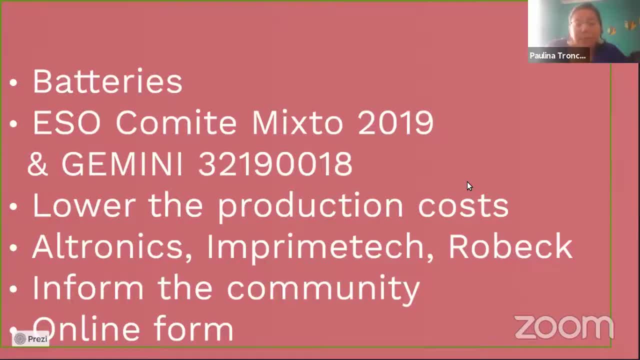 national park and listen the the clips with his, with their families, like in a closed environment. so not necessarily that because you you had some you you cannot see, you had to share it with the rest of the people. so this was like the one of the aims. but 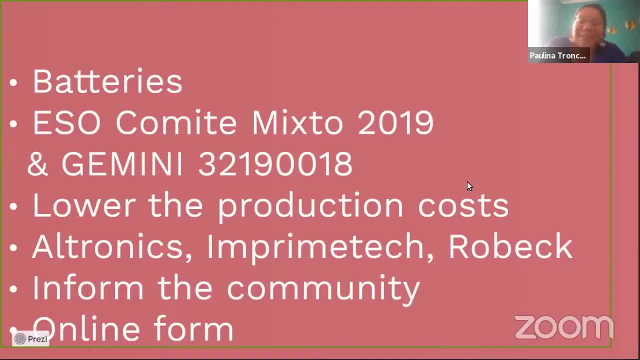 with the covet it is, let's say it changed a lot. so we are ending up with the transmission and all these things. so we rely in three chilean companies who brought us very nicely all the supplies, electronic supplies, the cases that you see and also the acrylic plates that we, we created. so 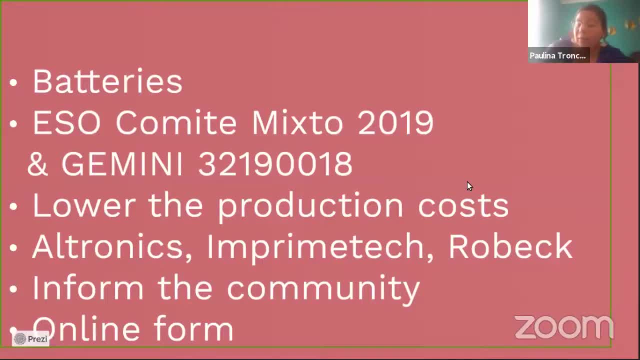 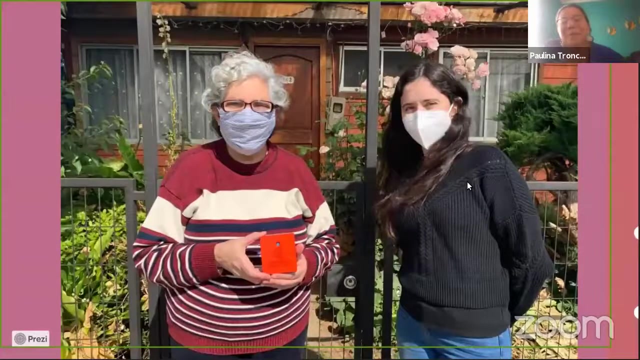 that you can see the electronic inside and we can motivate young people to say, yeah, why not? there are only three plates inside some wires. why i cannot do it? and with this we inform the the community and we submit an online form that we got so many requests and we started with the distribution. these are: this was our idea. i really 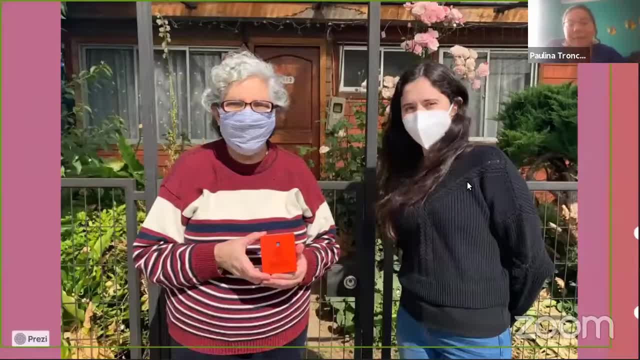 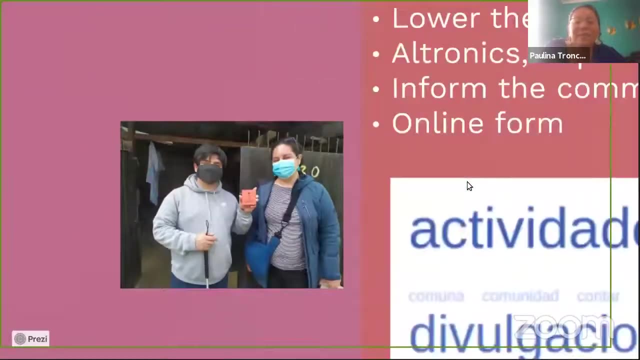 like to show this picture because we wanted to keep this light sound in in person. in the south she's leading the transmission of the eclipse on monday, resilience transmission. and this is erica. well, you know her also doing another device, but most of them were going like this, in boxes with 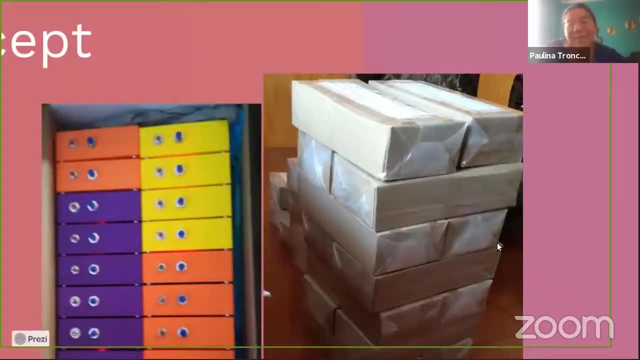 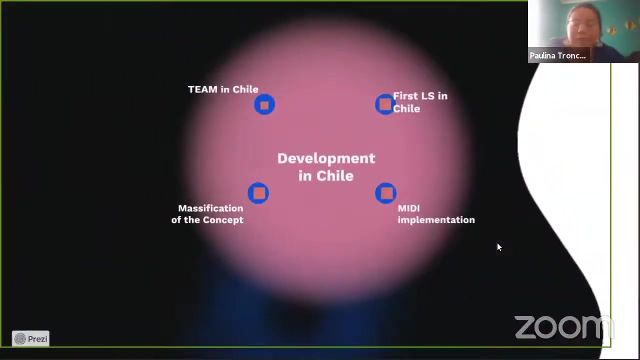 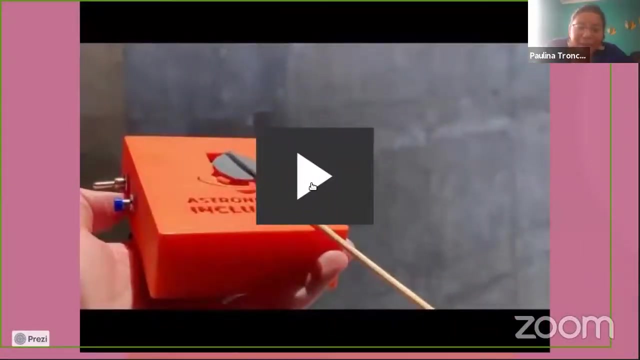 another kid from the years of the doscopio is a finger telescope is the name of this group and they sent a tactile kit for the people 140 and we put some light sounds in for certain people who wanted to share the signal. so we were playing with the electronic. that allison say and here 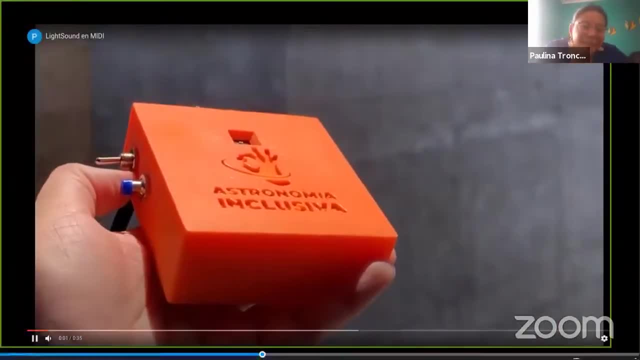 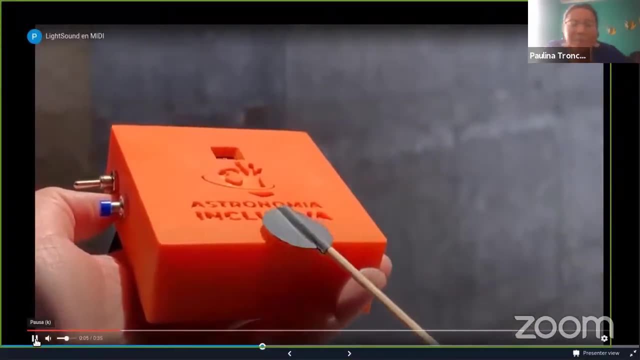 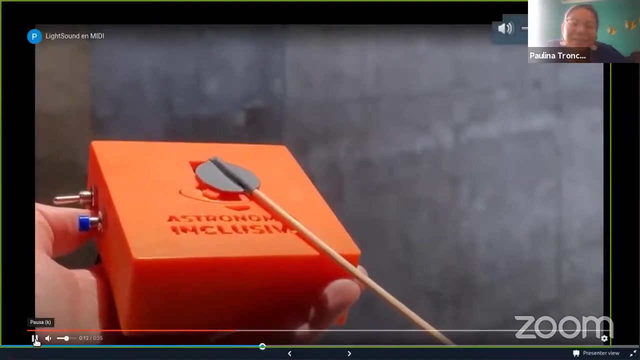 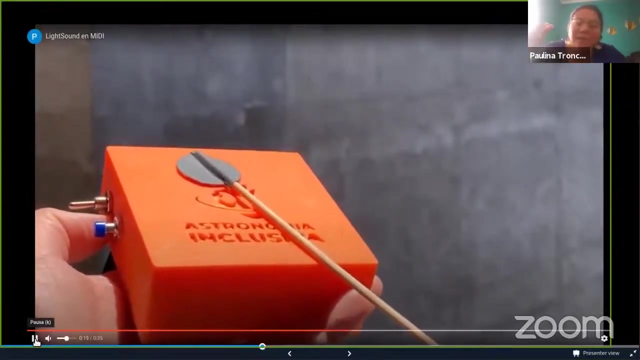 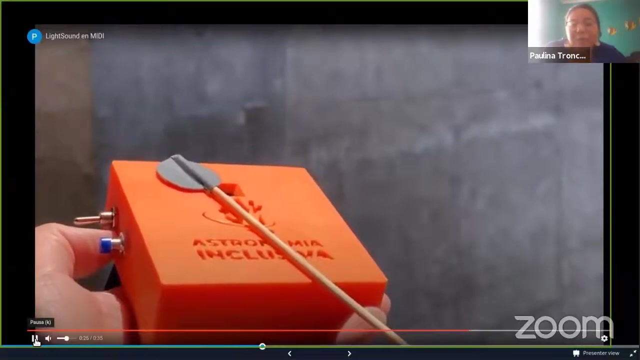 there is a. it's a different video because we implement music. so here is the device sounding and here is erica placing a fake moon. and when the moon, when, when the light is covered, the instruments are just switching off, and when the light is coming back, the instruments are included. 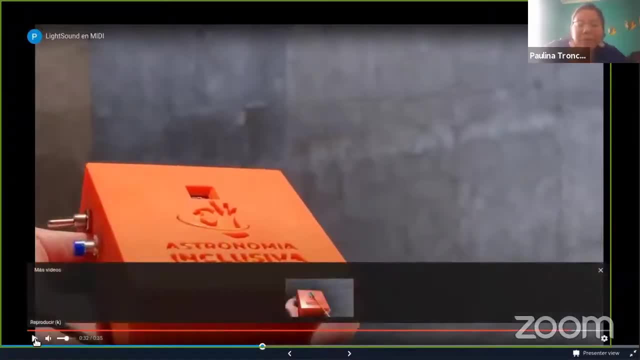 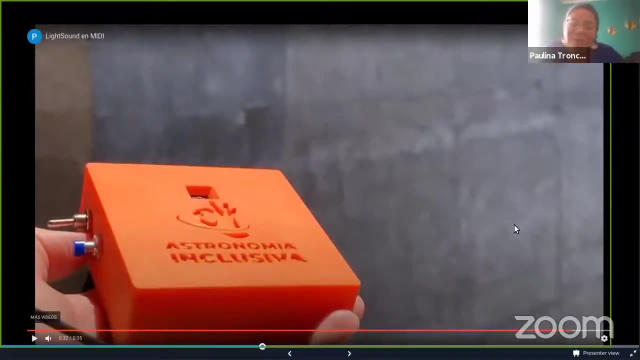 so our intention was that this personal use, that the people could start implementing their own most loved midi song in the devices. and i have to say on this we are a little bit late in the process. we are a little bit late on training the, the community. it's not an easy task, so we wanted to. 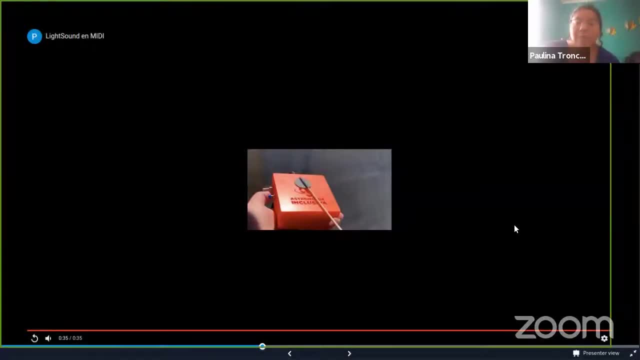 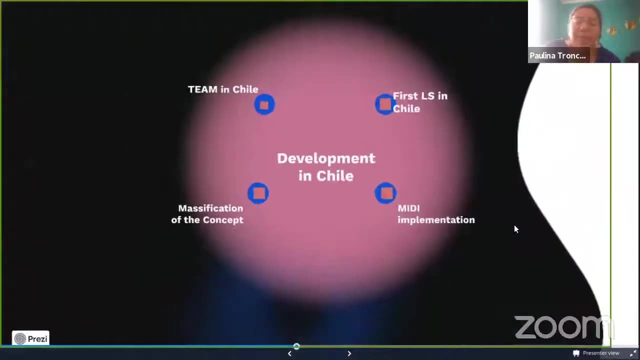 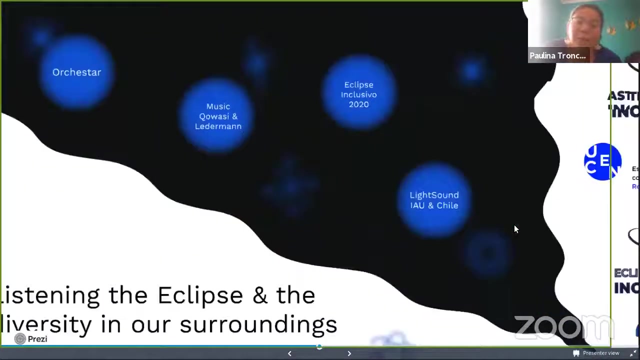 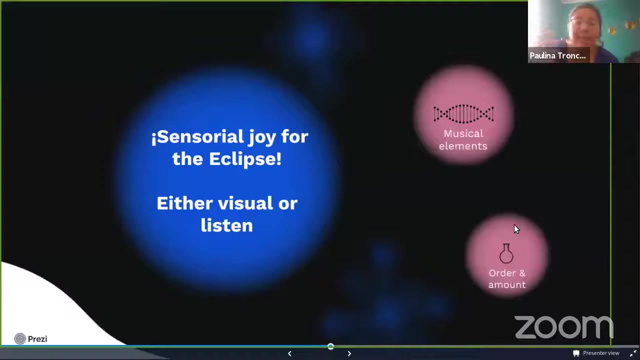 implement a melody, as i say, for the eclipse, except for our transmission. and we were a bit complicated with this because we start speaking with some musicians that are this, uh, rodrigo kowasi, igor lederman, to create a special, let's say, song, to give us sensorial joy, also for eclipse, but, uh, something that we can. 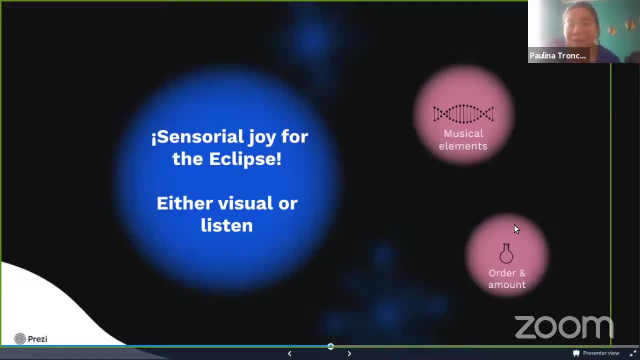 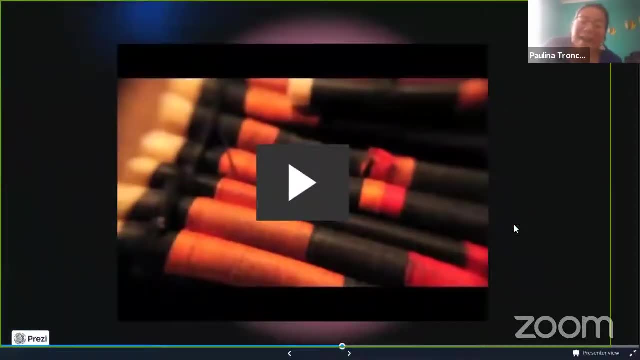 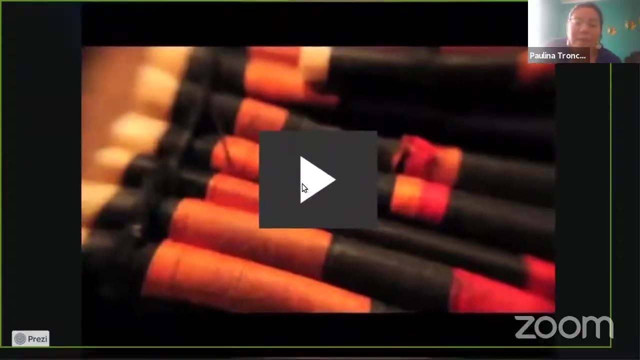 listen and, of course, if we are liking them one day and we don't have clouds, let's see- we will try or like and and the music that we started to implement, i, i choose this, these people, because they are playing this. let's say ethno, ethno. 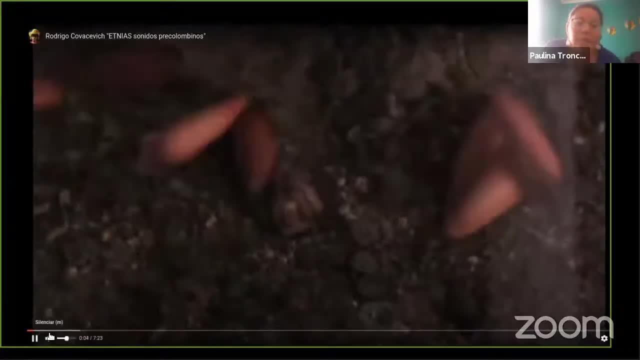 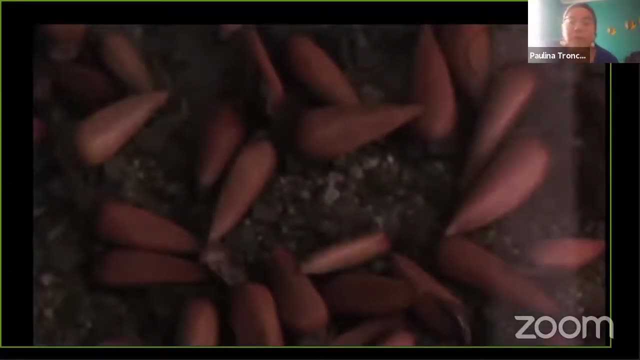 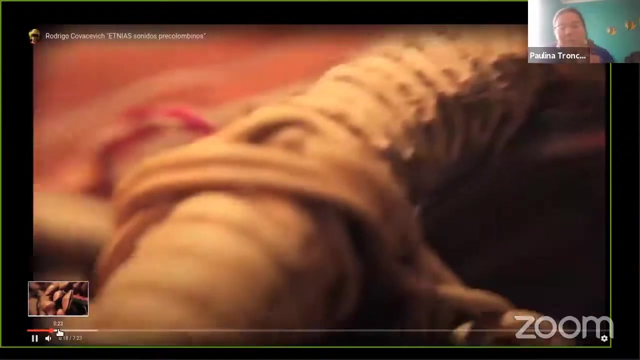 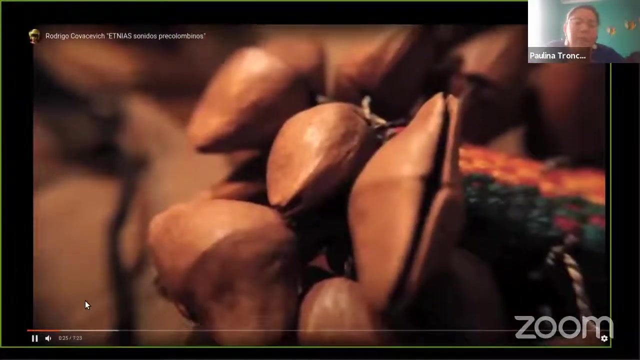 music, with some instruments that are related to to astronomy, to ancestral cultures or latin american in general, not only to the south of chile, and he's playing instruments that there are a written on. we're drawing the stones, but we don't have it now anymore and he's trying to reproduce this, the sound of this instrument. 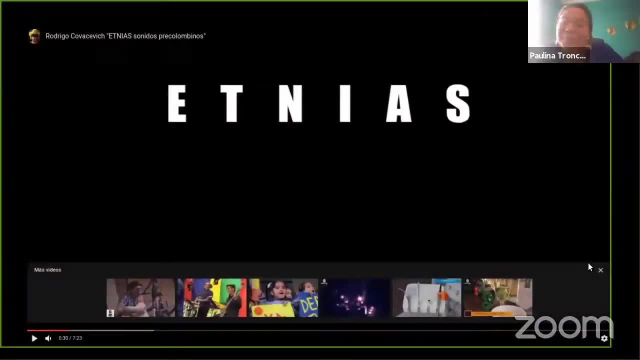 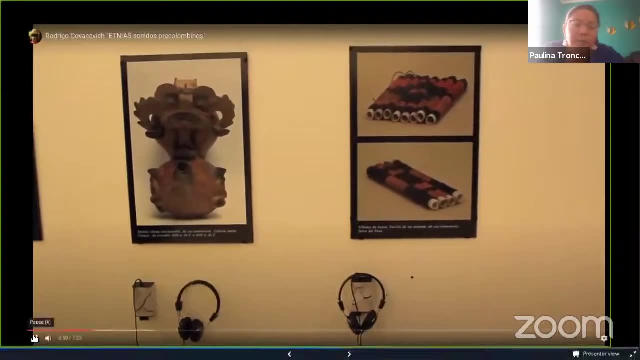 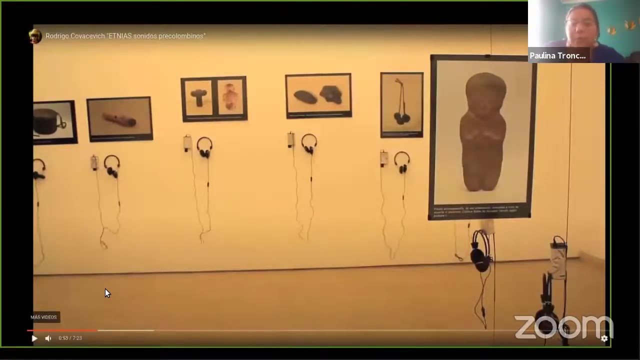 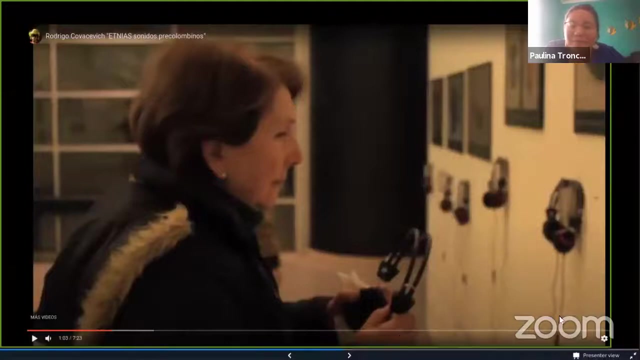 sorry, paulina, two minutes, okay, thank you. and and he's trying to to do this with all these instruments. so here is a. he's showing this in a museum and we were working, uh, together to to create something, let's say experiment. i i would call it a musical experiment mixture with science. 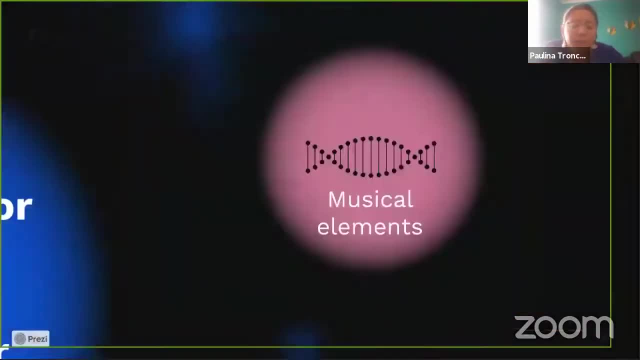 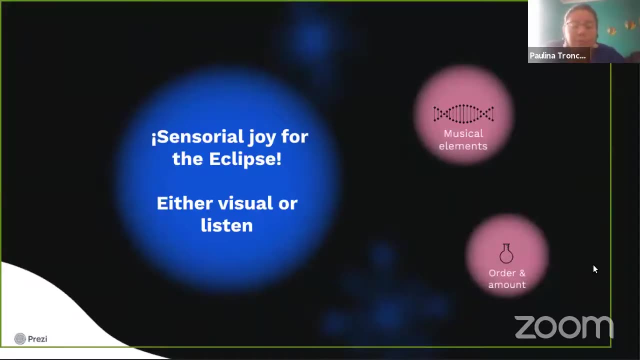 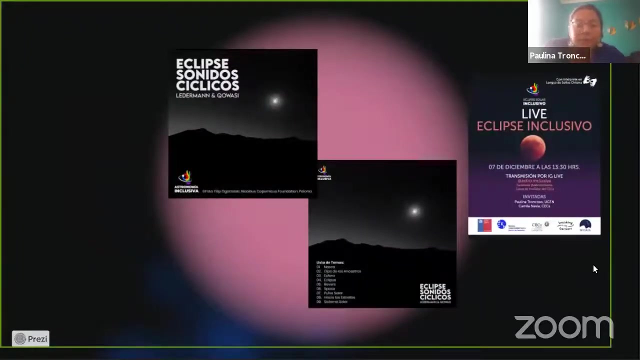 and, and what we did here at the end was to take, uh, this way, put a lab here to give an order and the amount of music that we want to put on it. so we started working, as i say, for the midis and we lower the cost of the light sound to 20 dollars with the place that. 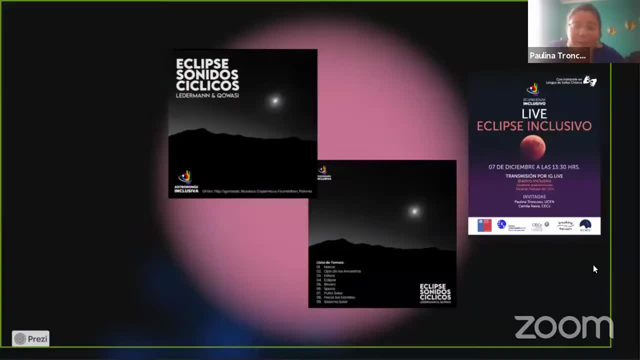 we, we bought here like more than 100, but if we wanted to go to the quality of this music in mp3 we had to go to, to the raspberry basically, and this was really rising the coast and we could not ship it everywhere. so we say, okay, we are also in kobe time, so let's do a transmission with this nice. 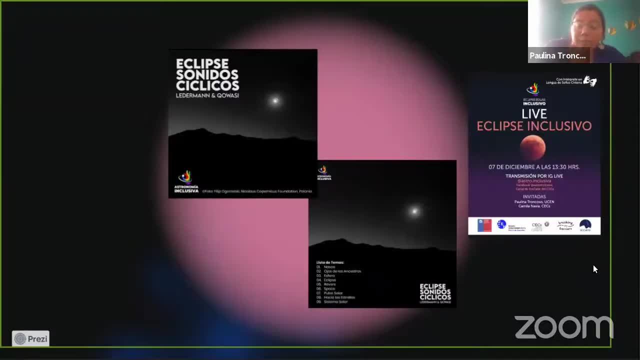 music, and the musicians were so motivated that at the end they created a full disc that is called a cyclic sounds of the eclipse, based on this music that I will not play now because I don't want to give you the spoiler, and we will transmit this on on Monday. sorry, here is wrong the date. 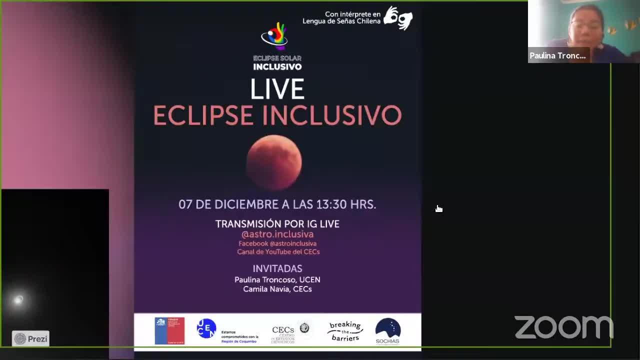 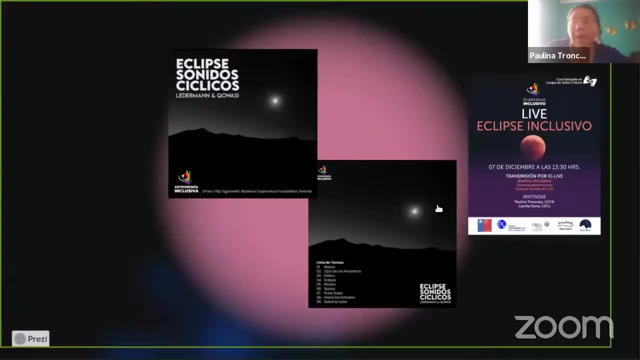 and we will speak the first. we will transmit the first half with the direct sound of the light sound, and when the totality arrives, we will have a surprise with this really nice music, and the music that we will play this day is not the full disc. it's a mixture of different songs that 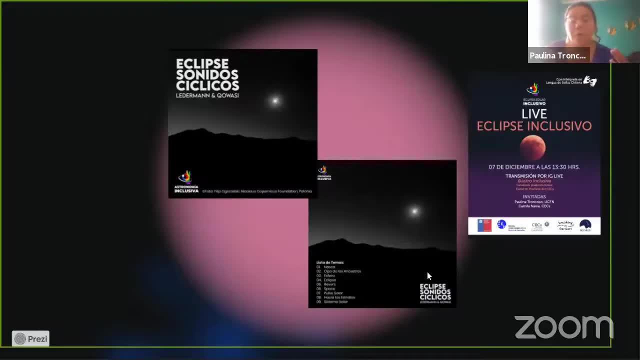 we believe. well, we, when we- I say we, I include also Carlos, a visually impaired person, who helped us to- to track, let's say you, our perception of this music and, and we will play with amount of times, the orders of the different songs to give, like the idea of the eclipse during this transmission. so I just want. 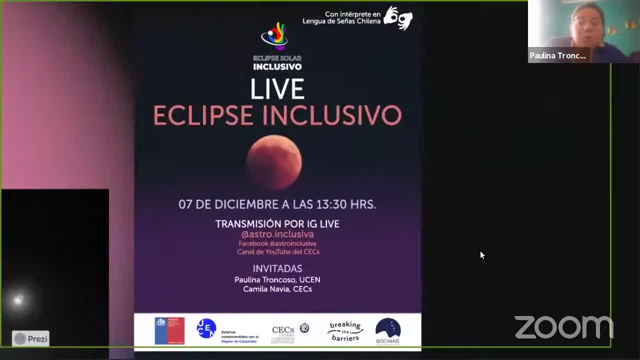 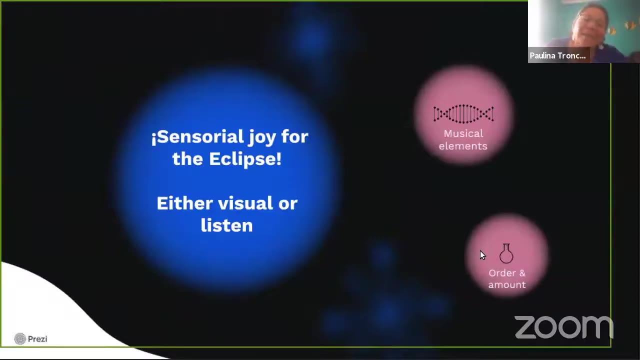 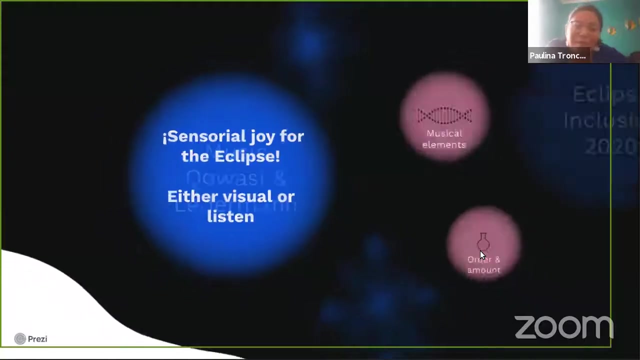 to let invite you for this transmission to to follow it on next Monday. it will be really, let's say, different. it will be in Spanish. I'm sorry, but the music is without any any language, with the idea of giving this sensorial joy. so here I think I have to stop. 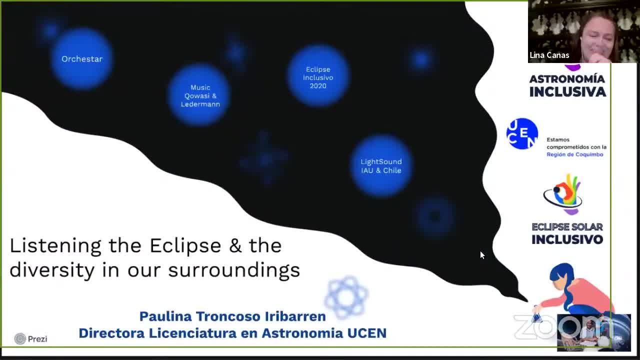 thank you so much, Paulina. this was so interesting and indeed it's incredible when we all collaborate and everyone can add on and add up to to the projects. thank you so much for sharing with us and with luck with the transmission for for Monday. I would like to thank all of you for coming on time. 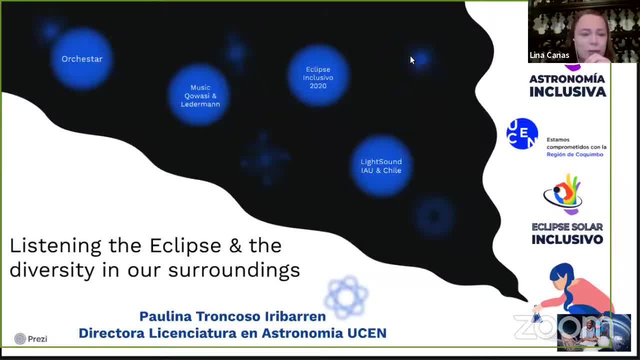 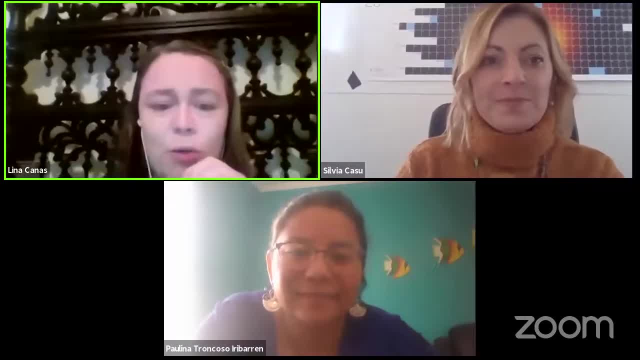 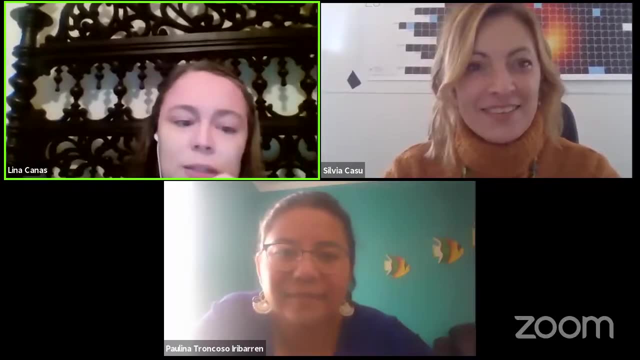 I would like to call my next colleague, Silvia Casu, for Instituto Nazionale d'Astrofisica d'Osservatorio Astronomico di Calgari, Italy, and she will talk about the Inmate Sky- Astronomy in a Juvenile Detention Institute. 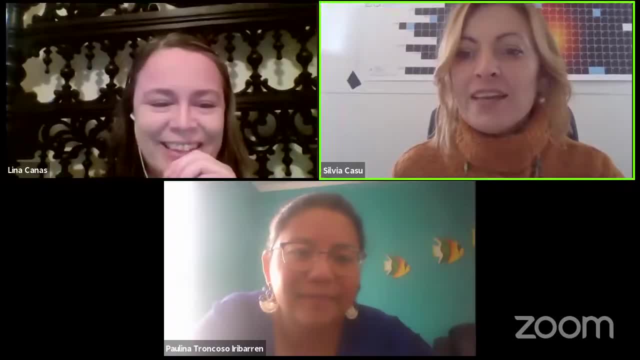 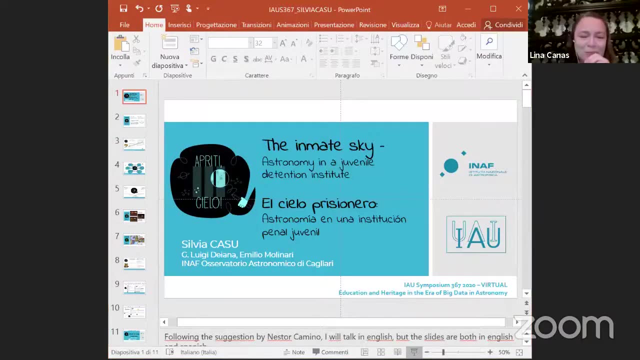 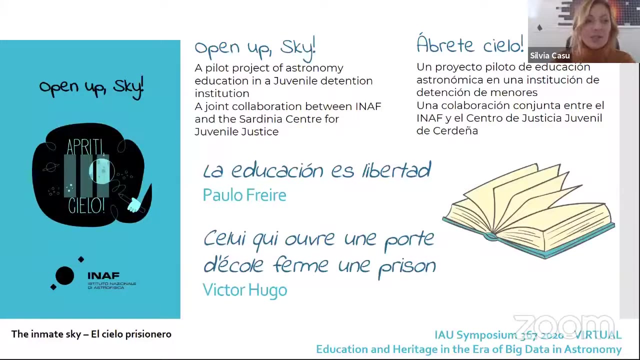 Silvia, the floor is yours. Okay, can you see my slides? Yes, we can. Thank you, Silvia. Perfect, So good morning to everybody. First of all, let me say thanks to the organizer to give me the opportunity to be here today. 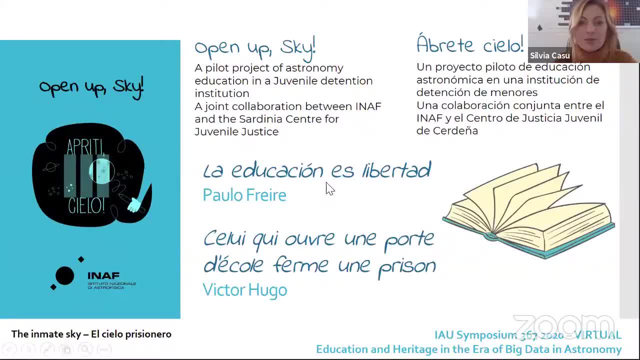 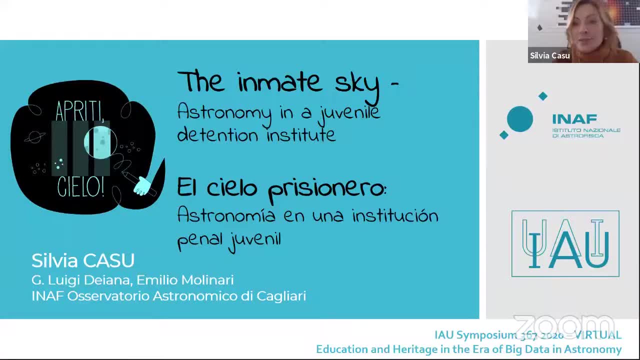 to talk about this particular project, which is called Apreticello. I cannot speak Spanish but, following the suggestion of- I would have done better if I spoke here the very first day- my slide will be in both in English and in hit Spanish. 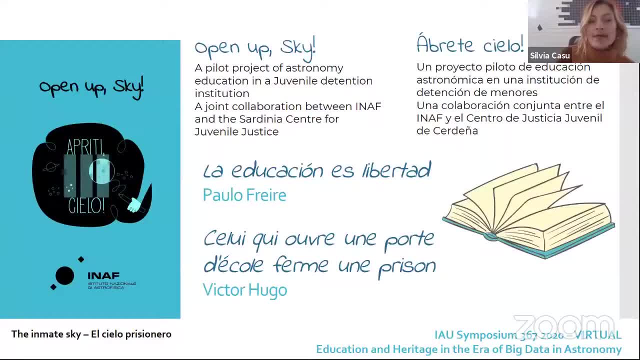 So the project Open Up Sky- Apreticello, Aprete i Sielo is a pilot project of astronomy education in a juvenile detection institution, based on a formal agreement between my own institute, the Italian Instituto Nazionale di Astronomia, and my work place. So if I don't get the opportunity to share the subject for now, that all will go into my own time. We are at two times told where we are going to be here next year. Thank you a lot. Thank you All right. 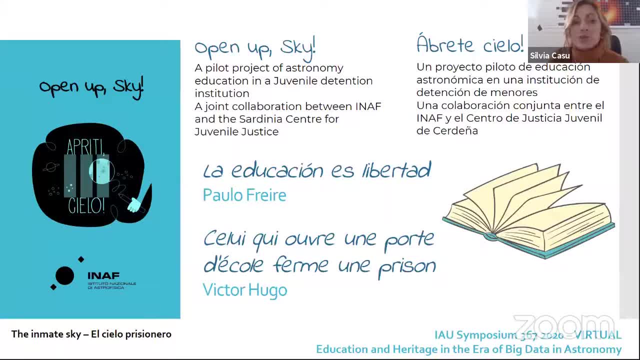 Bye, Bye, bye. Thus see you next year By Bye, Bye. Thank you for joining me. Our agenda today: Astrophysica and the Sardinia Center for Juvenile Justice. Well, talking about astronomy inside the jail. 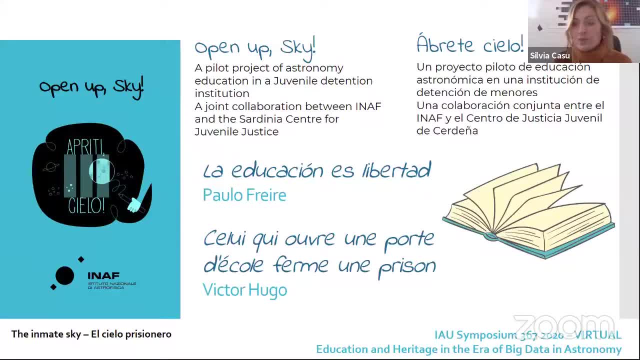 could be perceived as a bit paradoxical, because I'm sure that for most people, the word astronomy evokes the images of open, dark skies, perfect, infinite spaces, beauty and probably or definitely, the idea of an ultimate freedom. So why we should talk about astronomy to people who 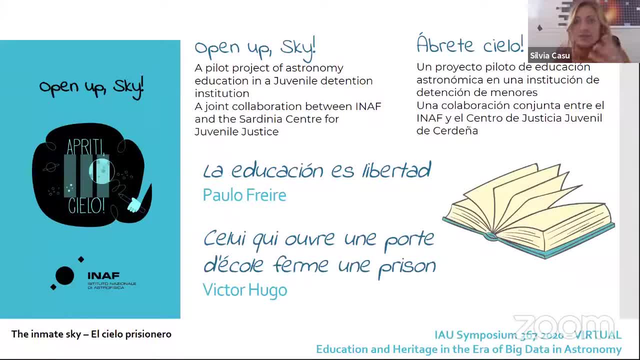 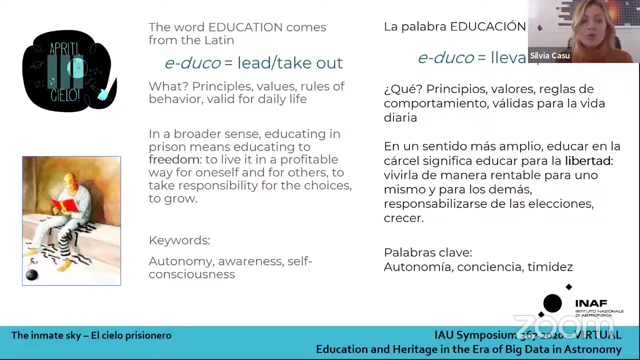 live in a distressing situation, locked in a well-confined space, deprived for a short or long period of their own freedom. Well, if we think about it, the word education, the real meaning of education, well, the word comes from the Latin word. 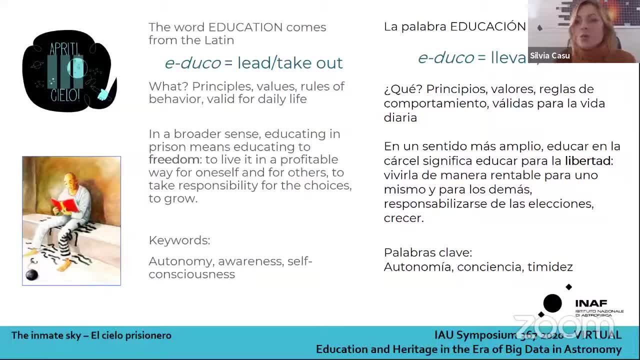 which means lead. take out What is education. So education means lead out principles, values, rules of behavior which are valid for the daily life inside the juvenile institution, but also in the external life, where Inmates will come back once the sentence is over. 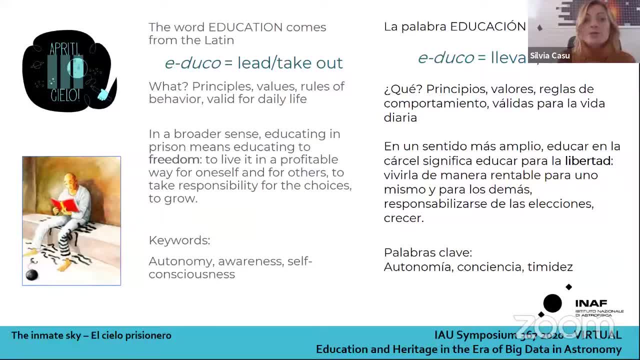 In a broader sense. so educating in prisons means educating to freedom, to live it in a profitable way for oneself and for the others, to take responsibility for their own choices and so definitely to grow And educating. Educating through astronomy means to- how can I say? 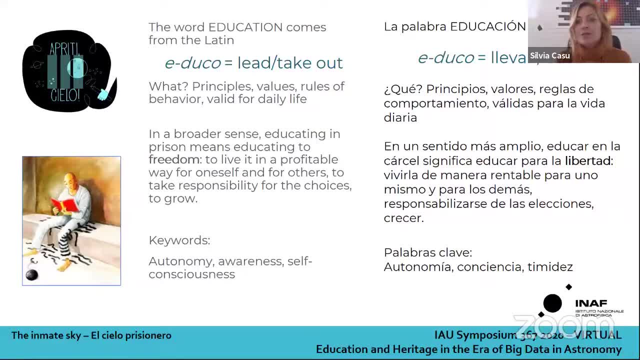 to bring back to elementary, to primary experience. for all Space skies often constitutes a place with which you have an affective relationship- And let's think about the moon, for example- And so it leads us, It leads us, It leads us to reflect on transversal themes. 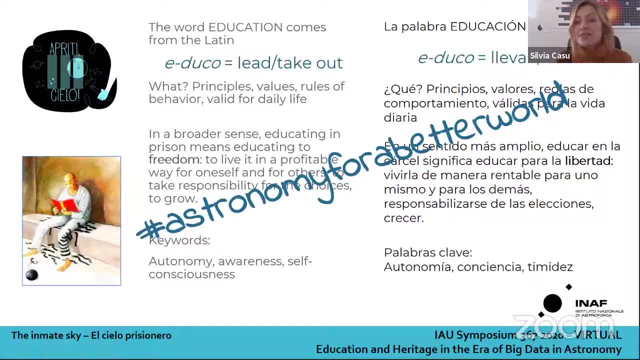 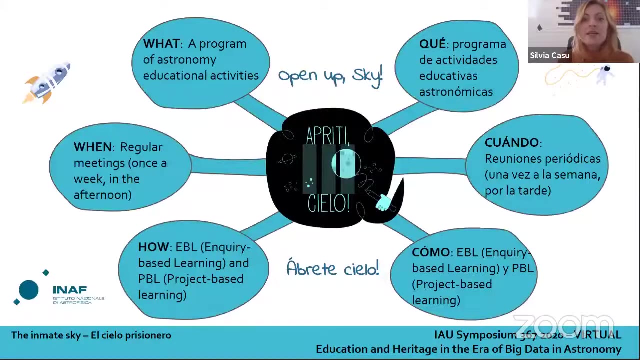 And this is exactly what we mean when we talk about astronomy for a better world, which is not only a powerful slogan, It's a lifestyle for me. So, following this main idea, in February 2020, we signate the formal agreement for the project. 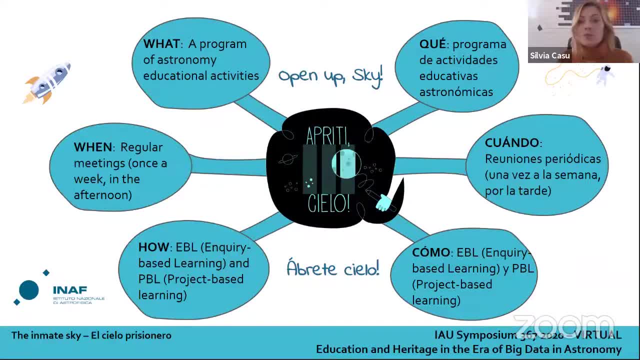 Open Up Priticello, Open Up Sky, Which is a program of astronomy educational activities for young men inside the juvenile detention institution. The project is based on activities. There's been a project called the many women in Vietnam as a team, And it's quite unique. 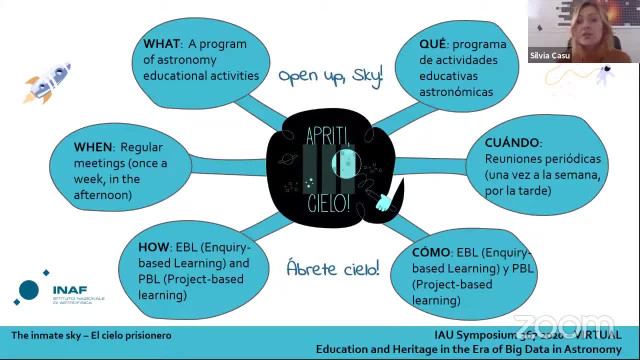 OK OK, whose methodologies have been agreed with the educational responsible of the institution and is based on a project-based learning approach centered around the learner, and attendance of meetings have been fixed once a week in the afternoon. The project was supposed to start in March 2020 but has been postponed due to the pandemic, and we discussed with 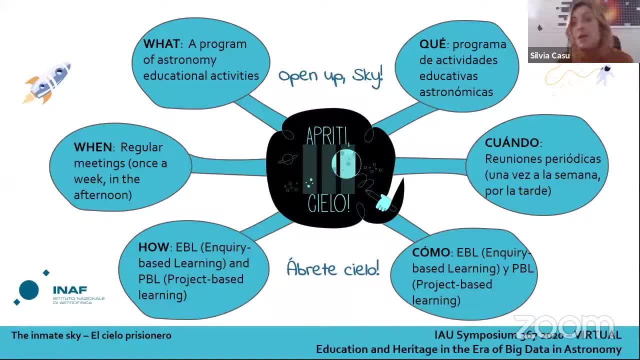 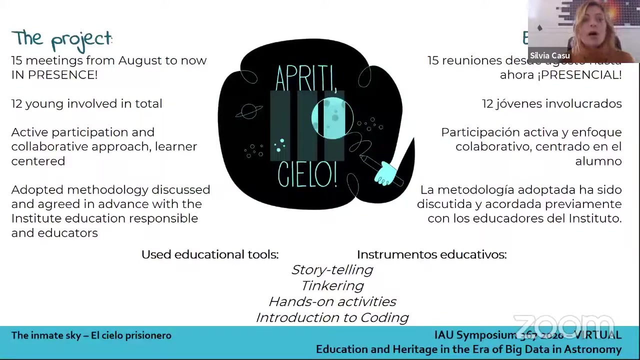 the responsible of the jail to start anyway in online modality, but we preferred not to alter the deadline, The nature of the project, because the presence was one of the very important part of it. So the project started in August 2020.. Until now, 15 meetings have been held in the presence, involving 12 young men in total. 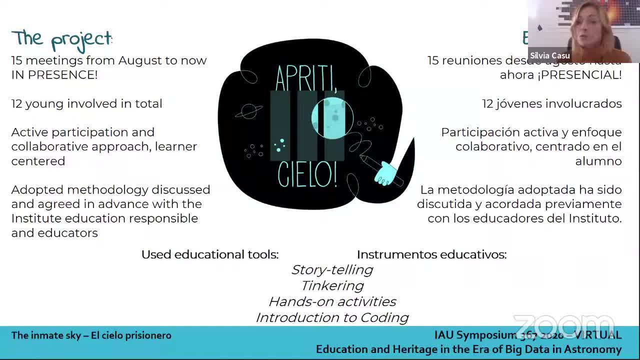 The project is still in progress. So many other, a lot of other meetings are scheduled once a week, so on a regular basis We adopt a constructivist and constructionism approach and principles: privileged learner center and collaborative approach with active participation by these young men. 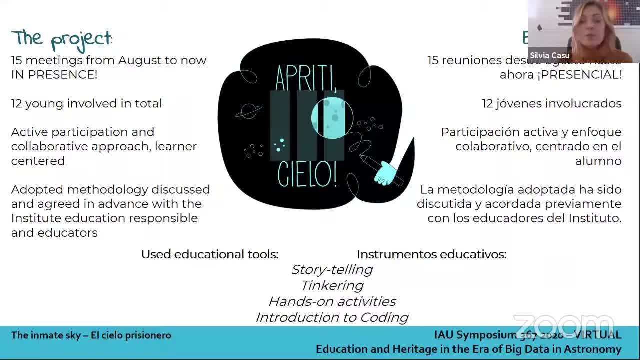 And during the project we use different educational tools. So we use storytelling contests describing scientists' biographies to be linked with the inmates' lives And experiences. We use thinking to introduce research methods and processes. We use hands-on activities to introduce astronomy objects and phenomena. 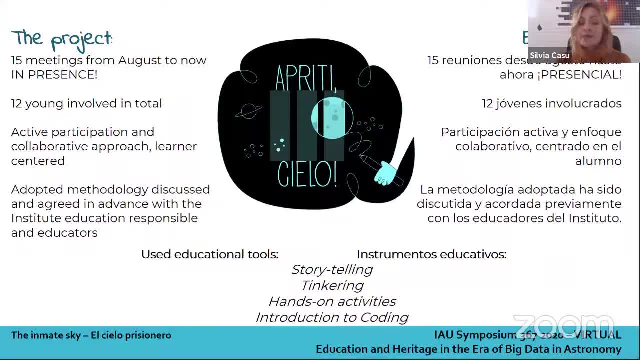 And we also introduce coding basis to promote the computational thinking. We also succeeded to organize a stargazing event. Of course it was a very interesting event. We also succeeded to organize a stargazing event. Of course it was a very interesting event. 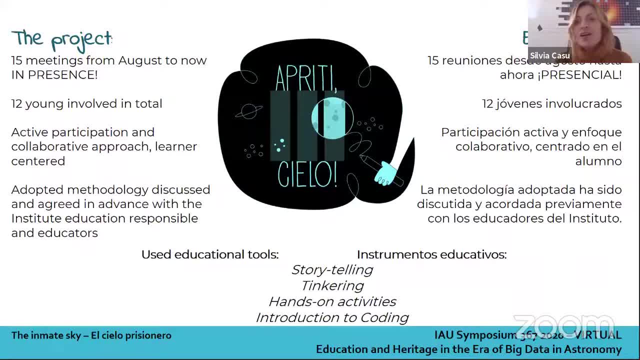 We also succeeded to organize a stargazing event. We also succeeded to organize a stargazing event. However, the kind of events that we visit inside the prison, with the natural limitations due to the artificial security. Unfortunately, as you can easily understand, we do not have pictures of the various activities. 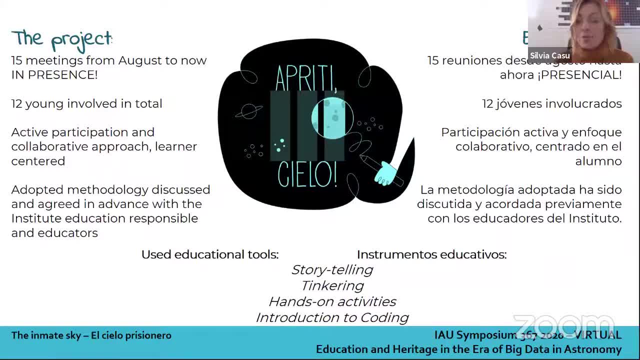 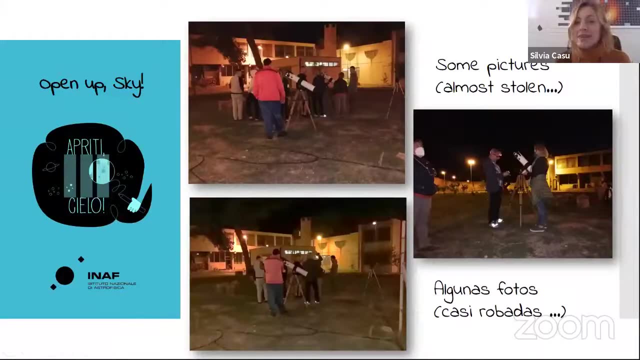 even if we obtain the same pictures in very particular moments, show you two of the most engaging activity. First of all, the stargazing event. For the inmates, it was the first time at all they approached to a real telescope And for most of them, the first time. 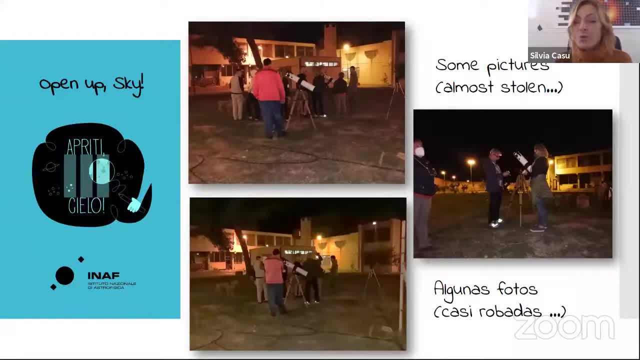 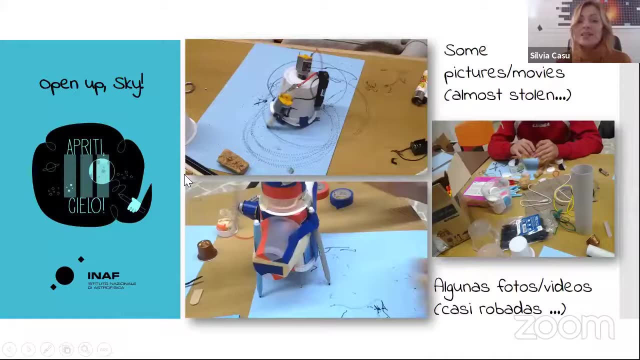 they really watched the sky, So they were completely excited. They were completely fascinated by this activity. It was a really big success. Another funny activity was the well-known tinkering activity Sylvia. two minutes, Yes, OK, Thank you, Sorry, sorry. 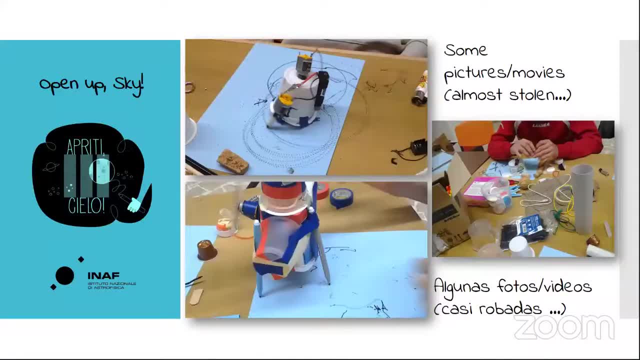 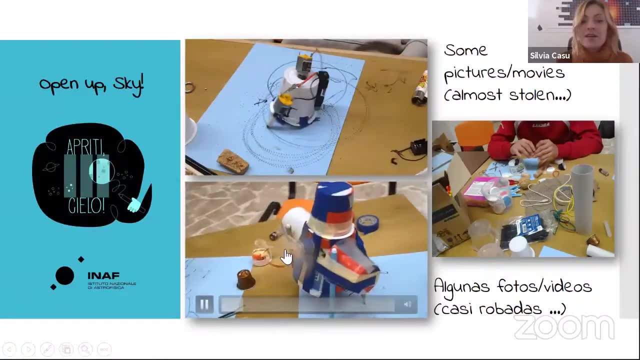 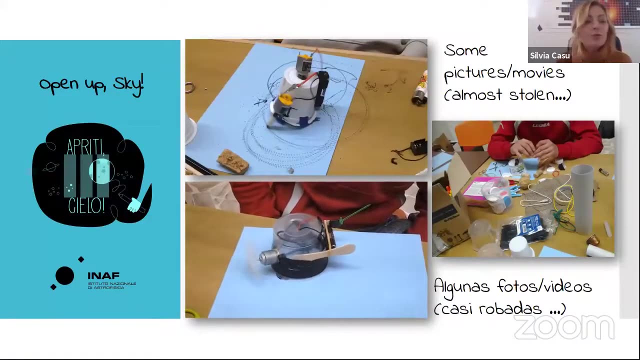 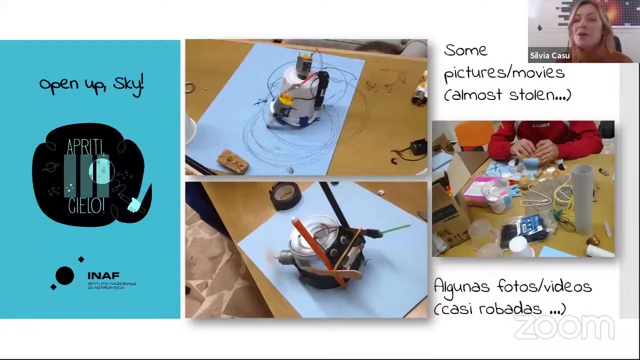 No, it's OK. They spent almost two hours committed to the activity And they had a lot of fun. I can show you just some of that. They are creations. I can't believe me. They created the wonderful objects, extremely different projects from one of the others. 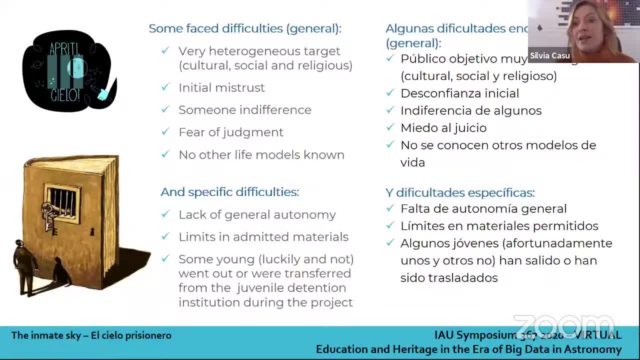 Of course, we faced some general and specific difficulties, because they are a very Thank you. Thank you, I hope you have enjoyed it. Thank you all for watching. It's been so good to have you on board And thank you for being here. 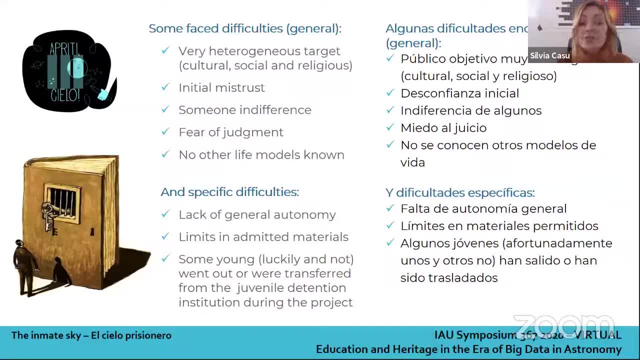 And please. I would also like to say a thank you to the team of the Holocaust Centre. Thank you. If you have any questions that you have, please feel free to put it in the chat. We will be getting some more questions from you. 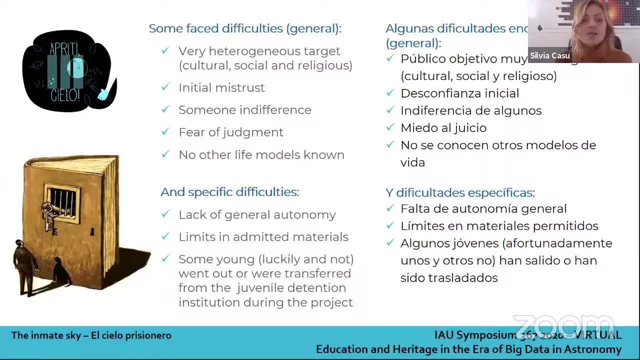 in case you have more. Thank you, Thank you for the good feedback And I would also like to say a very well done and a very nice presentation and special thank you to the entire research team of the Holocaust Centre, of the Holocaust Centre in Italy. 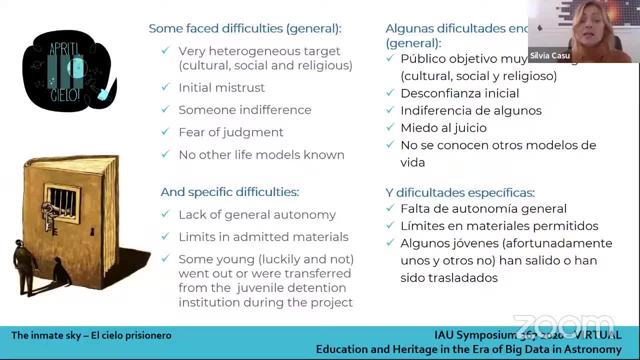 And I invite you all to join us. at the end We will be having a lot of other works available. They could be limited by the fear of judgment and by the lack of knowledge of different lifestyles. In addition, in jail there is a general lack of real autonomy. 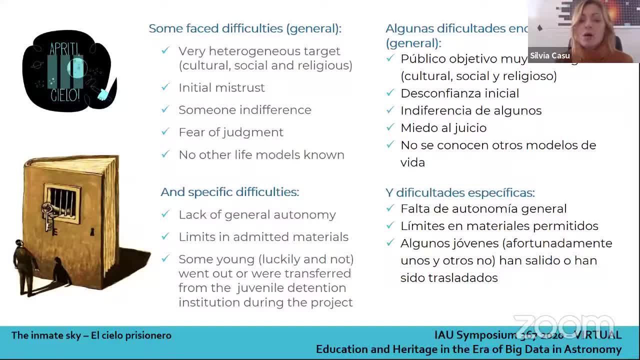 We cannot use really any kind of materials and tools for the end zone activity, for example. Last but not least, some young for different reasons. well, they exited or they have been transferred from prison during the project, So it took time to establish an emotional, educational relationship with them. 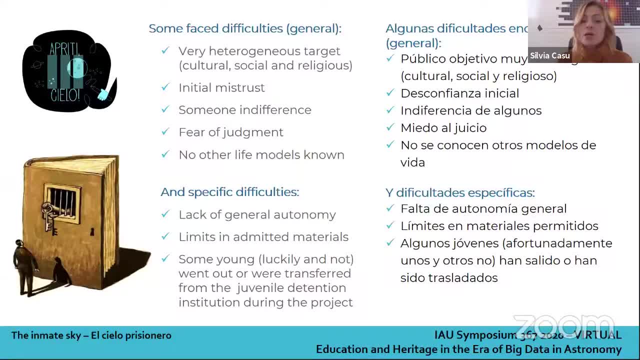 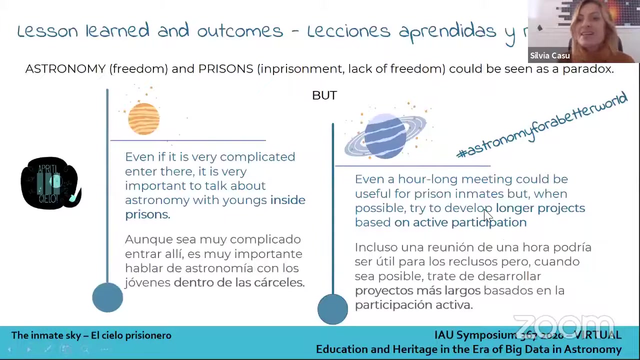 To face all these problems, we benefit of the professional advice of a therapist. We have a psychotherapist who is following us in all the steps of the project. Anyway, even if the project is not well completed, we can summarize some lessons learned and some outcomes of the project. 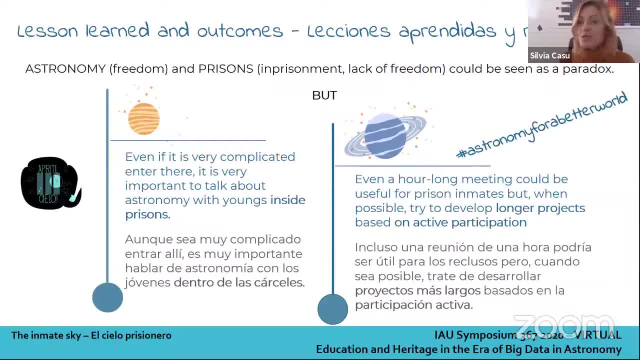 We promote the use of astronomy, astrophysics and space science to encourage and support the self-determination and self-expression of the individual, regardless of gender, social status, culture of origin and, of course, of committed crime. Even if it's very complicated to enter inside the jail, it is very important to talk about astronomy inside prisons. 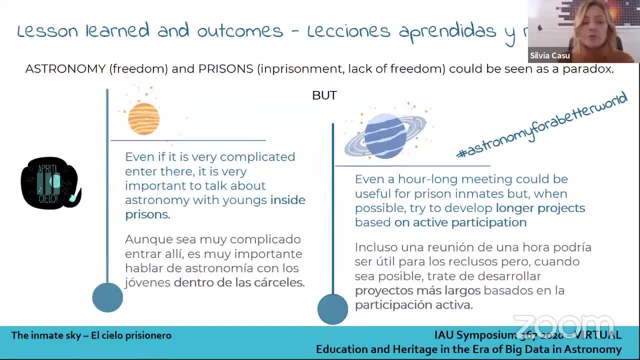 By providing the opportunity to talk about astronomy inside prisons, by providing the opportunity to talk about astronomy inside prisons, by providing a new point of view, new perspectives for involvement and participation in culture and knowledge formation processes, we aim to help people to find and maintain, of course, complete control over their own decisions, and definitely on their own lives. 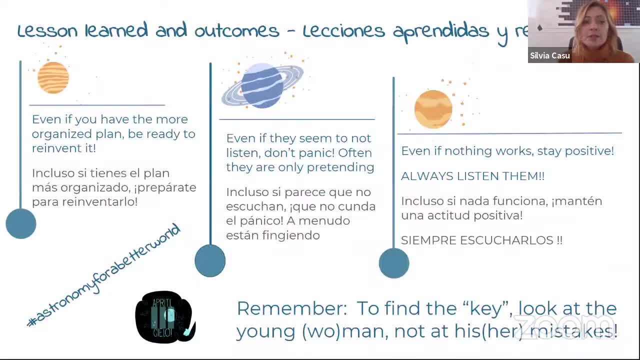 Again, it is important to be organized But flexible- Sorry, Silvia, time is- And to be able to follow the interest and change plans in the last moment And to be patient and to maintain, to keep a positive approach, positive in all the parts of the project. 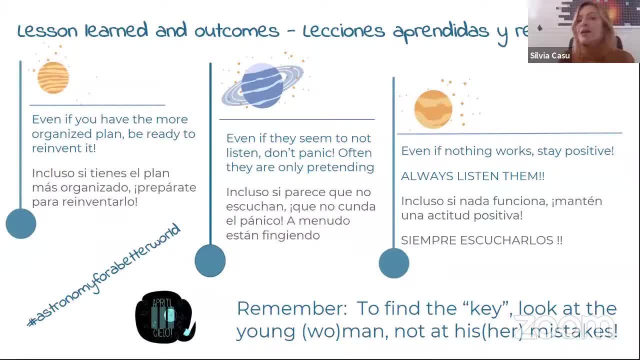 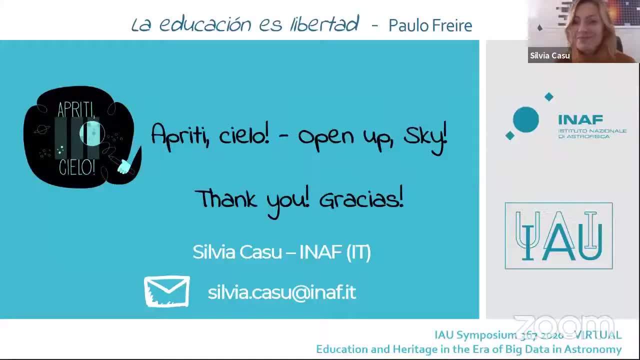 And remember: look at the young men, but not their mistakes, Thank you. Thank you so much, Silvia. This was quite, quite interesting And there's, I see already there's a lot of a few questions for you at the end of the session. 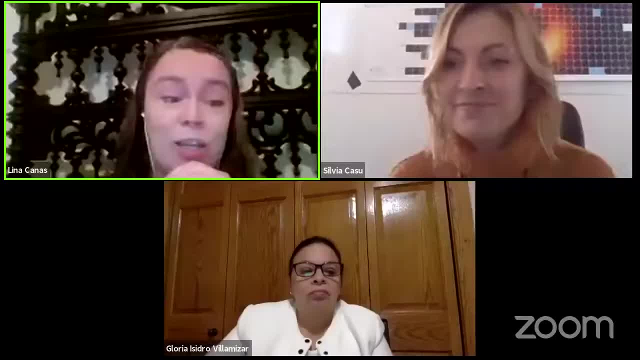 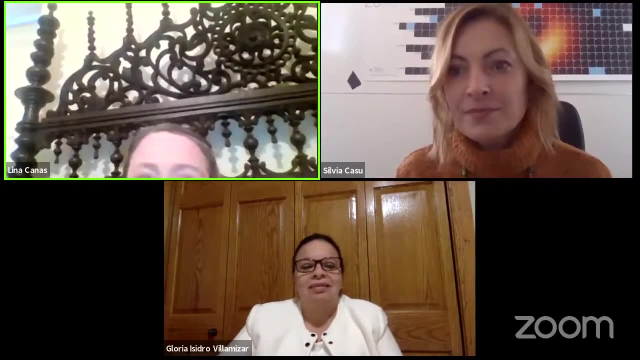 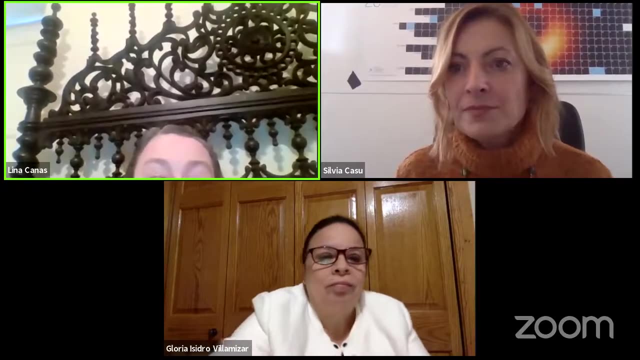 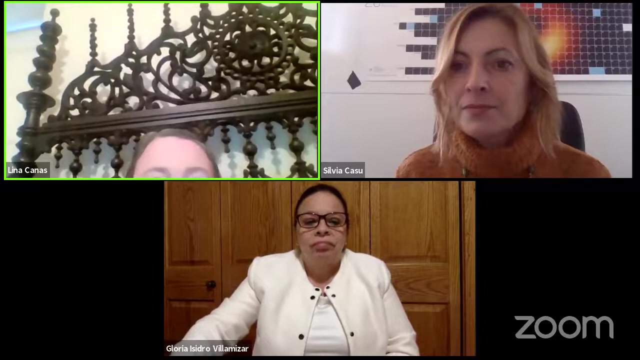 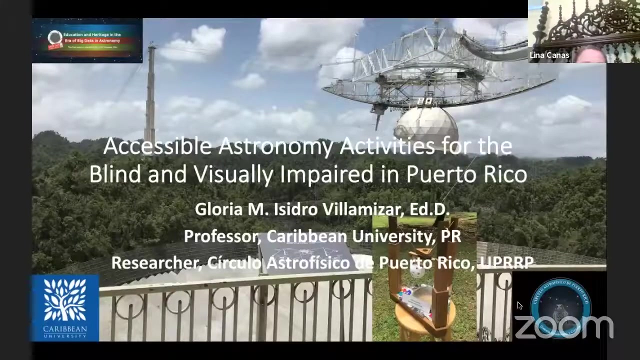 Now I would like to call Gloria Isidro Villamizar from the Caribbean University, Puerto Rico. Hi, Gloria. Thank you, Elena. Hello, Gloria will be giving her presentation in Spanish with the slides in English. In the true spirit of our inclusion session, we will be very diverse in the language in which we present this following presentation. 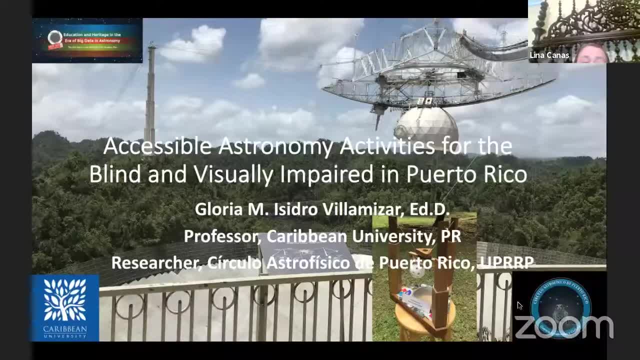 And Gloria will talk about the accessible astronomy activities for the blind and visually impaired in Puerto Rico. Gloria, Go ahead. Thank you. 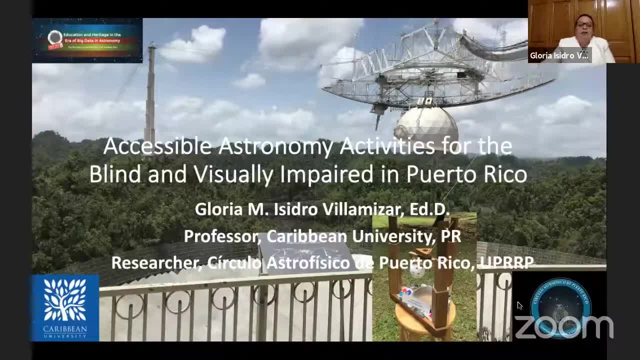 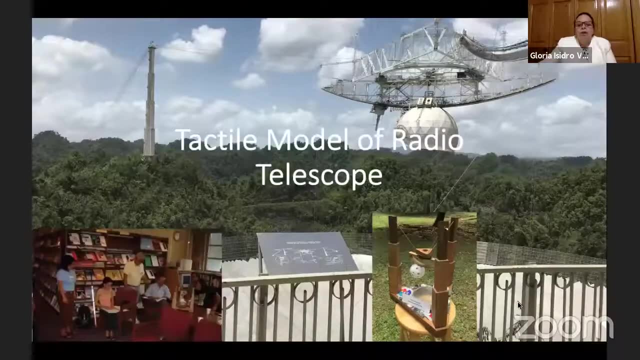 A blind person. what did that wow, that admiration mean to all the people who, from a balcony or a viewpoint, could be observed by the radio telescope? 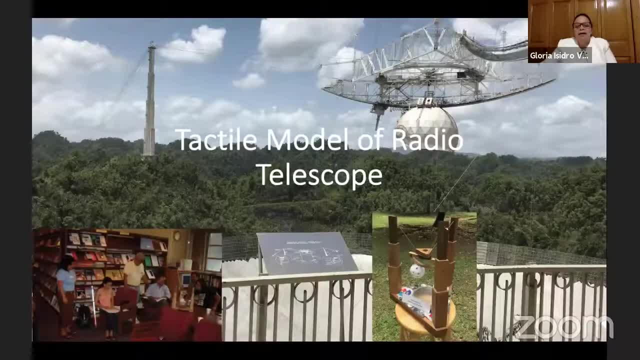 It was necessary, then, to make the Arecibo Observatory an accessible observatory for blind people. How did we do it? We did it by designing an unbreakable model of the Arecibo radio telescope, accompanied by a card that explains the parts of the radio telescope. 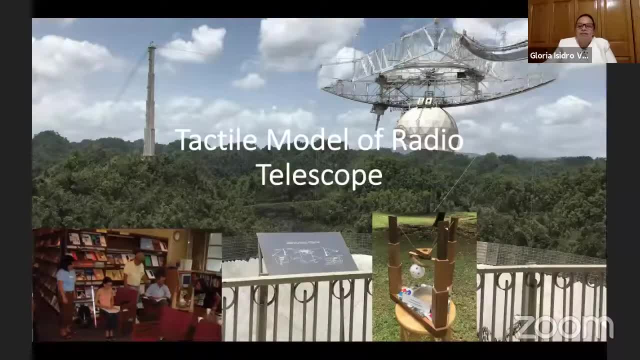 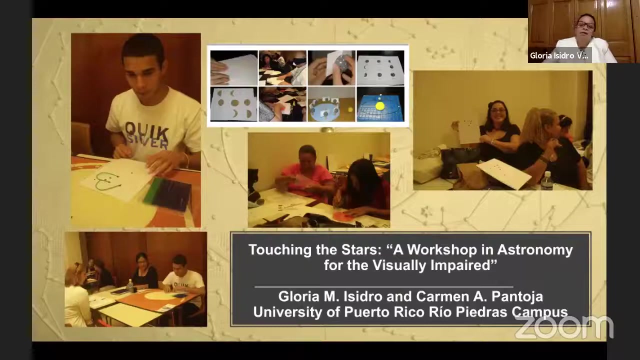 another card that explains the important definitions in astronomy and frequent questions. We designed it with the help of students from the University of Puerto Rico- blind students who helped us in the design, Also in the Arecibo Observatory in the following year, 2007,. 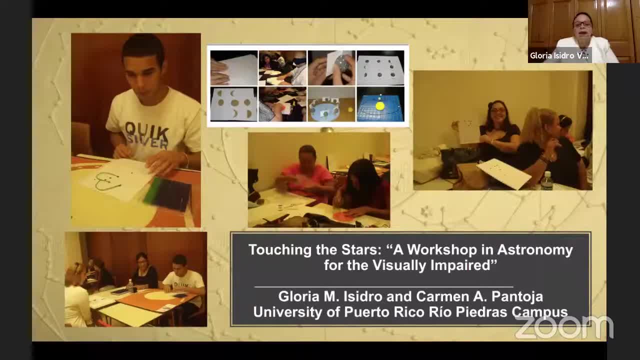 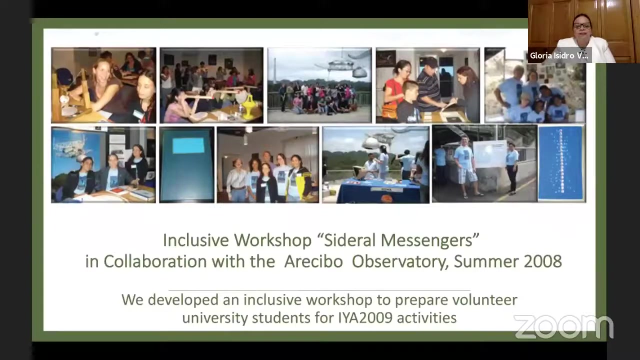 we were developing materials to do a workshop directed to astronomers and directed to higher education teachers in terms of how to teach a blind person the phases of the moon. Already in 2008,, we developed a workshop where we prepared university students, including two total blind students, who would be working as volunteers in all the activities of the year 2009.. 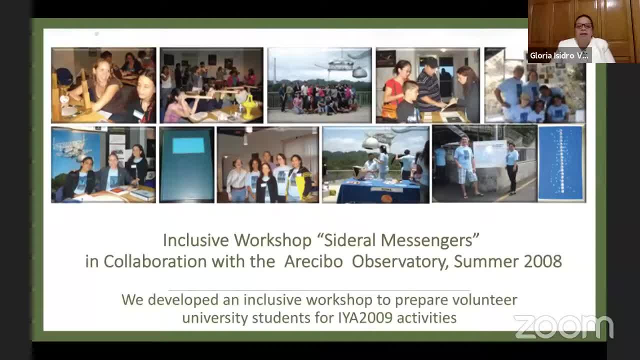 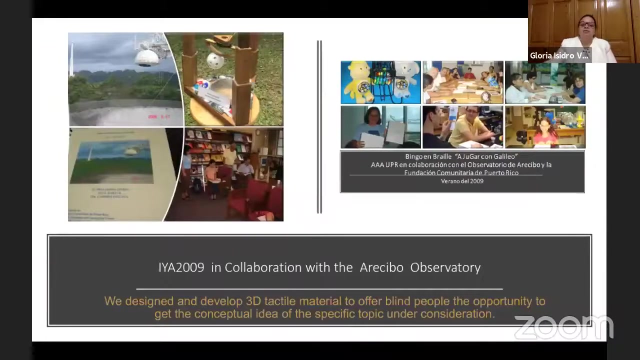 To develop this workshop, it was necessary to create tactile materials, to design three-dimensional materials so that our two total blind federal messengers could serve the public in general in our activities. Starting then in 2009,, we had in the Arecibo Observatory visitor center. 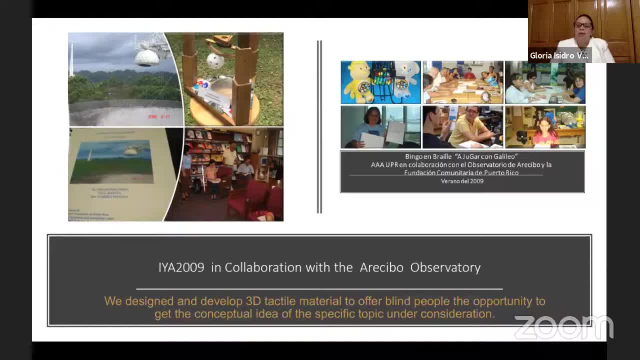 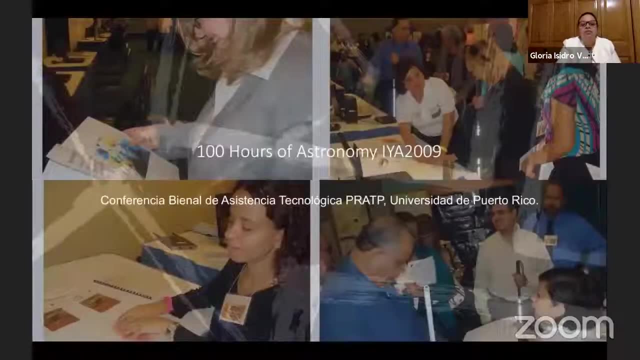 the bingo game Embray to play with Galileo, A bingo with cards. Embray with enlarged letters with texts about the solar system. We participated in the 100 hours of astronomy, where we had an assistance, a great assistance. 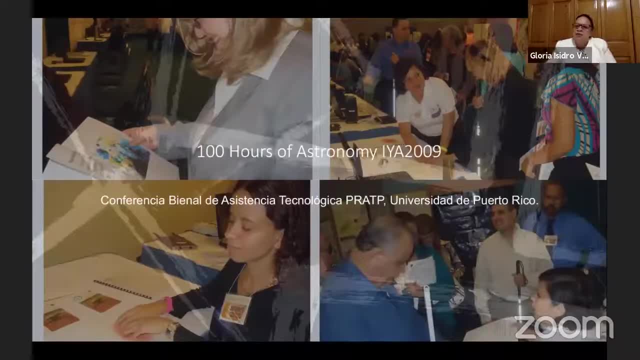 of a total of more or less 100 blind people from all over Puerto Rico who were present at the Bienal Conference of Technological Assistance of the University of Puerto Rico. There we presented images in relief. we presented the disassembled model of the Arecibo Observatory. 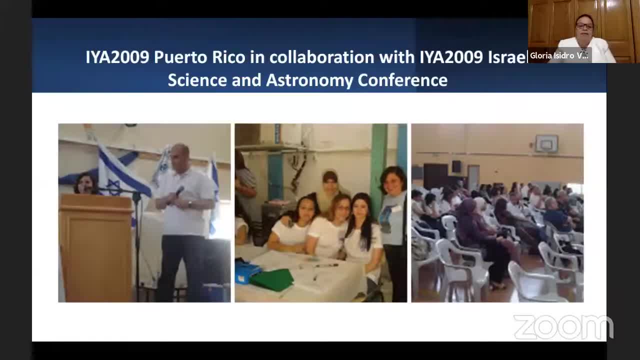 We were invited to be at the Science and Astronomy Conference in Israel at the opening of the International Year of Astronomy 2009 in Israel, And the next day we went to that was in Haifa, and the next day we traveled to Fula. 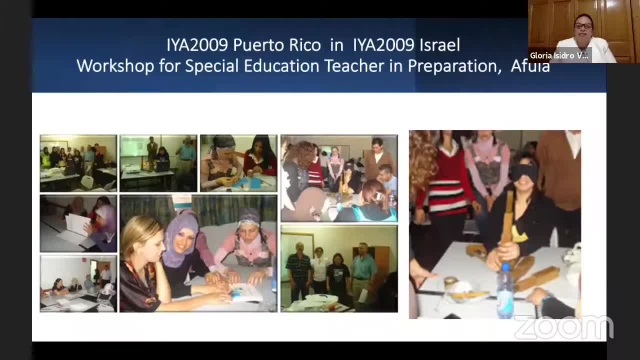 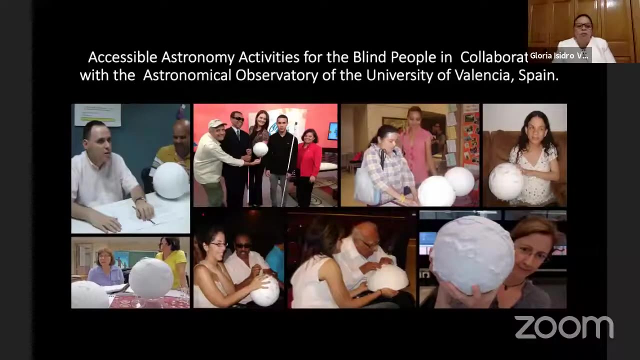 where we developed a workshop for students who were preparing to be special education teachers. The students were preparing materials for relief, the way we were doing it in Puerto Rico. The media in Puerto Rico, such as television and newspaper channels, published the activities that we were doing. 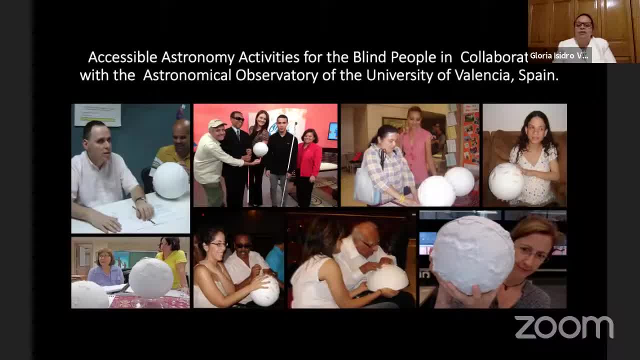 already in 2010,, in collaboration with the Astronomical Observatory of the University of Valencia, We evaluated the prototype of the tactical moon model, to then have the final model of the tactical moon, developed in Spain, a model that was evaluated with blind people. 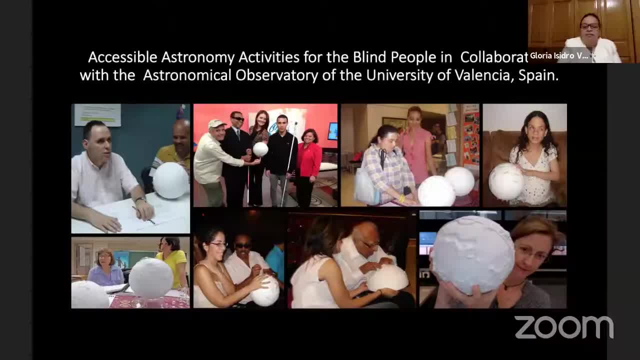 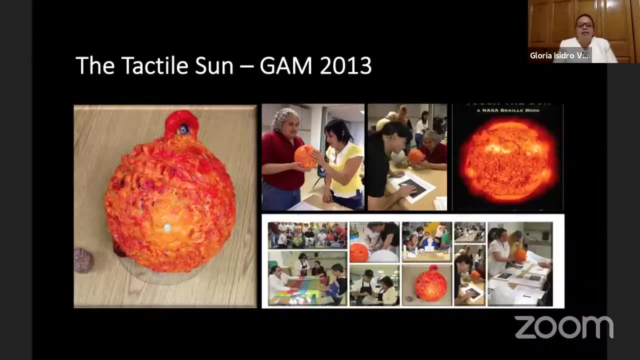 in 10 different countries. And after the moon came the sun, The sun. we were working on the tactical sun with the direction of the sculptor artist, the blind sculptor, Luis Felipe Pazalacua, who directed the sculpture workshop Manos que Miran. 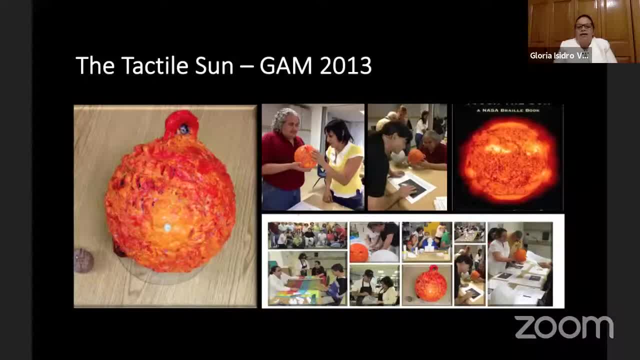 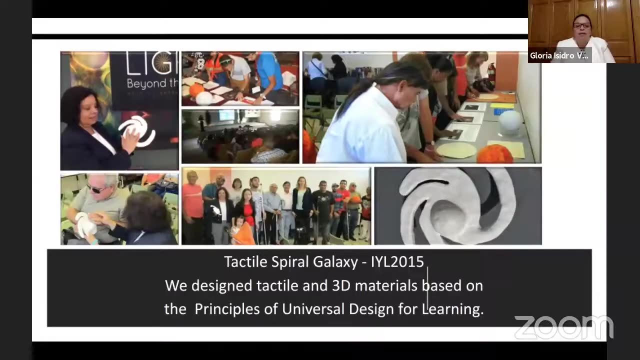 Working as a volunteer in that workshop, we were able to make the sun as a piece of sculpture. Continuing with our sculpture works for the International Year of Light, we developed the model of the galaxy, a tactical model. Every time we develop a model. 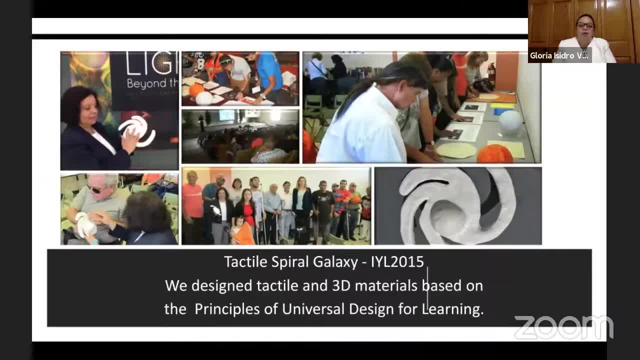 we hear the voice of our collaborators- blind people- and we take into account the principles of universal design for learning. In this specific case of the spiral galaxy model, we realized that the model could be taken with one hand and that the blind person with the next hand. 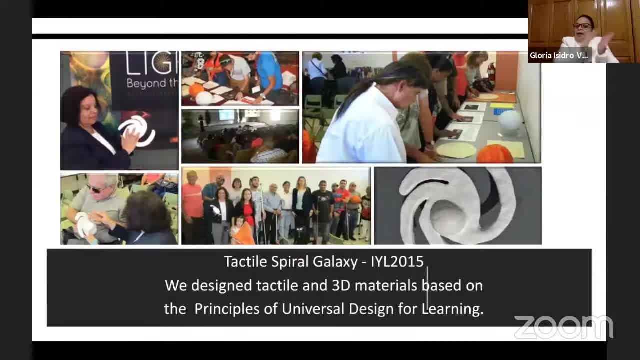 could feel, could find the nucleus of the galaxy and could find the phrases. The texture of the model of the galaxy is very smooth. It is important when we design materials for blind people, to take into account the texture that really causes them to touch. 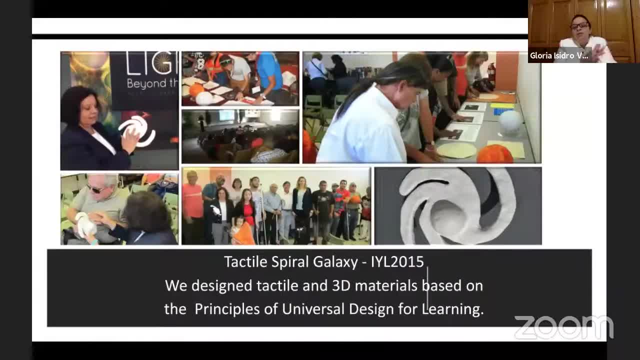 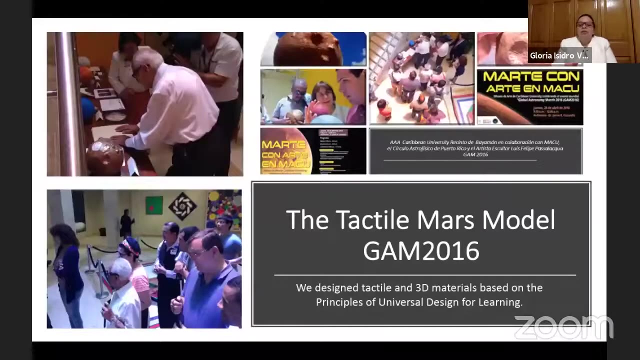 that the size is an adequate size, that the person next to the blind person also enjoys and appropriates that knowledge that we are explaining to them at that moment. After the International Year of Light in 2016,, we developed Marte con Arte. 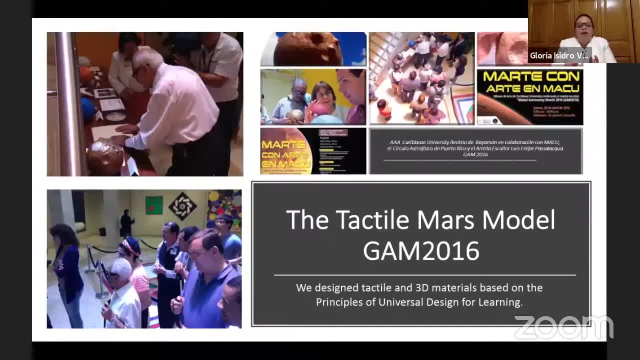 Marte con Arte is a piece of sculpture where, in an exaggerated way, the characteristics of the Martian surface are expressed. You can find Mount Olympus, the Tarsis mountain range, the Great Volcano, La Carita Feliz. This was a presentation. 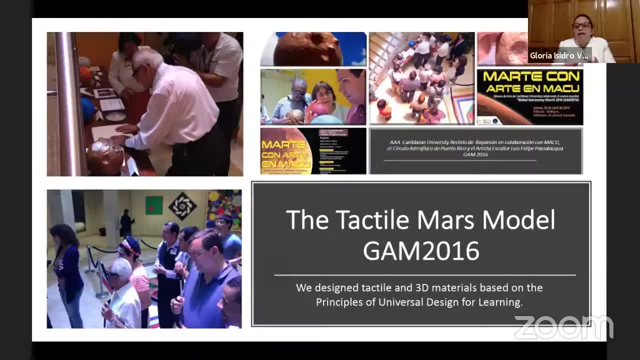 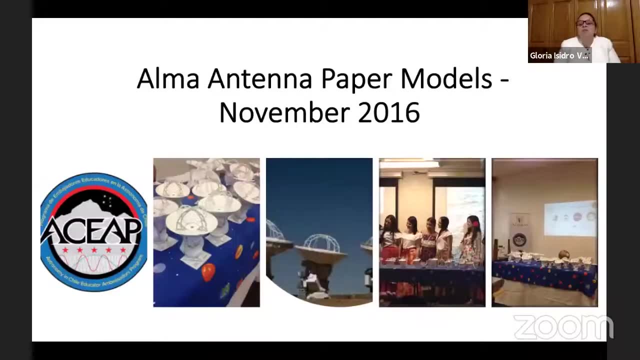 that we did in collaboration with the Caribbean University Art Museum and the different associations of blind people to whom we invite to Gloria, sorry, two minutes. Okay. We also developed the model of the antennas ALMA, a paper model. Sixty-six. 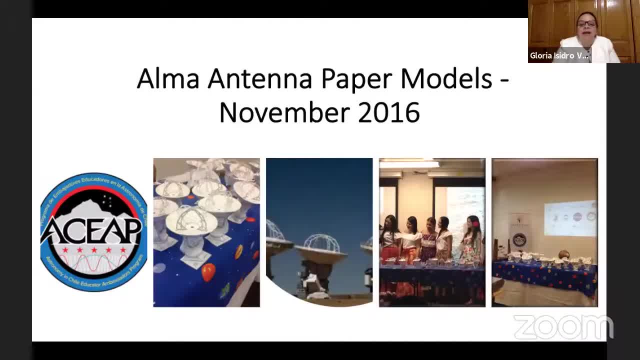 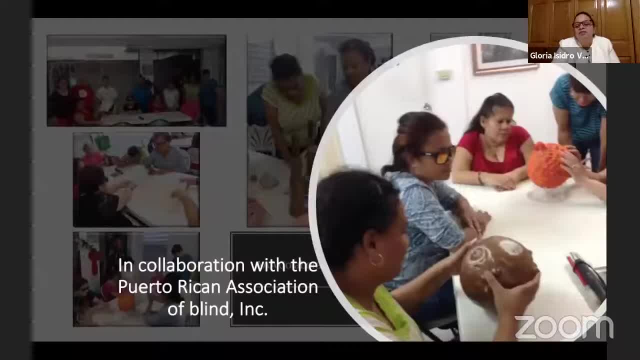 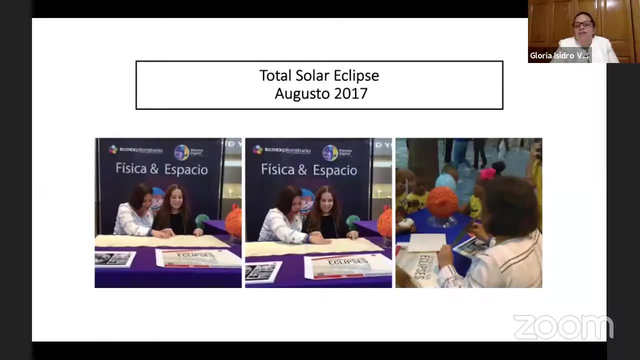 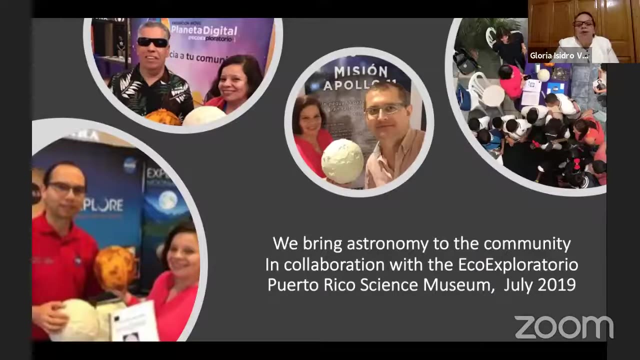 Sixty-six antennas made of paper were made in 2006,, 2016.. And we took them to blind associations. we divulged the solar eclipse. in 2017, with the book by NASA, we celebrated the 50th anniversary of the Moon. 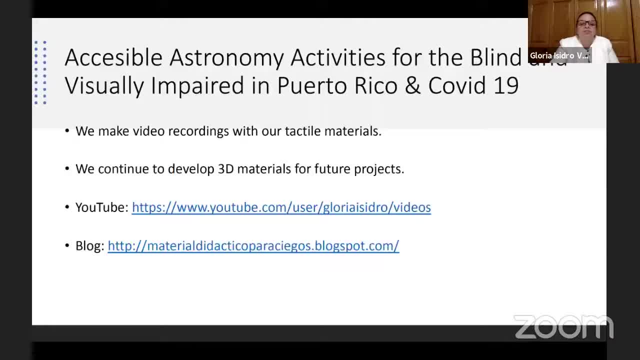 at the Science Museum of Puerto Rico. So what's going on with COVID now? Well, we can't do our activities so that those materials can be played. That's why we're making videos, so that all people can know about the activities that we develop. 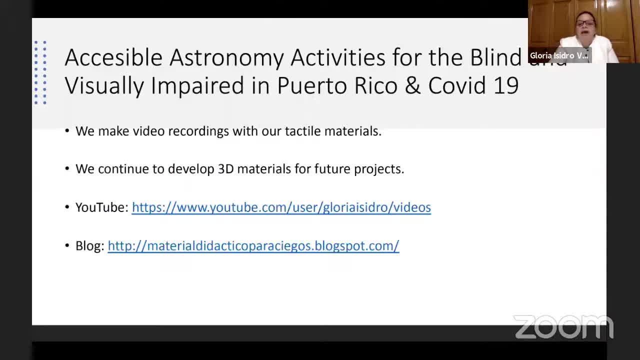 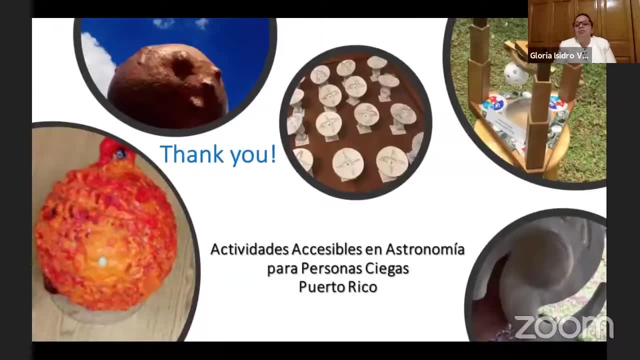 We also continue to develop three-dimensional materials for future projects. So thank you very much. Thank you so much, Gloria. It's always a pleasure and it's always amazing to see your history with inclusion and your activities, and that span over well over a decade. 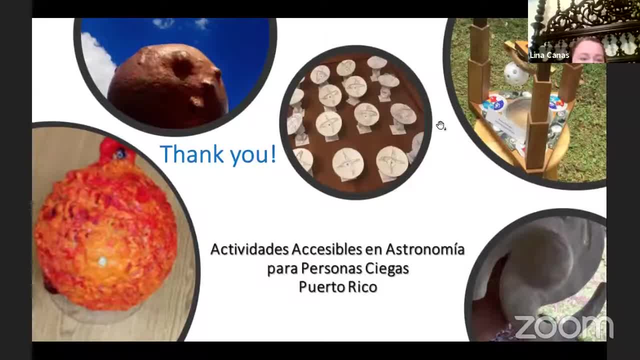 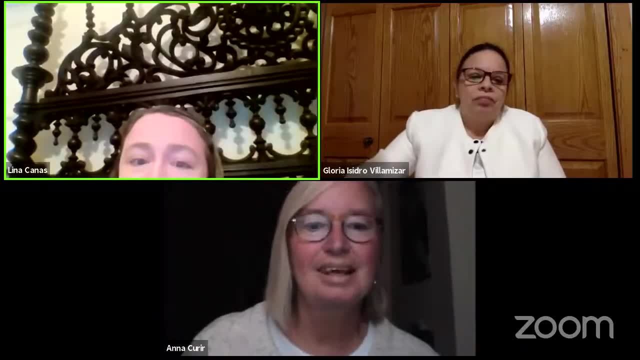 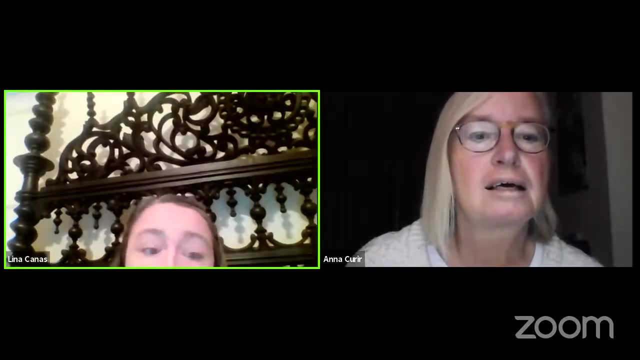 And thank you so much. It was fantastic. I would like to call now my colleague, Anna Curir, from INAF Observatorio Astrofísico di Torino, Italy. Hello, Hello Anna, Hello Nina. Anna will talk about women in astronomy. 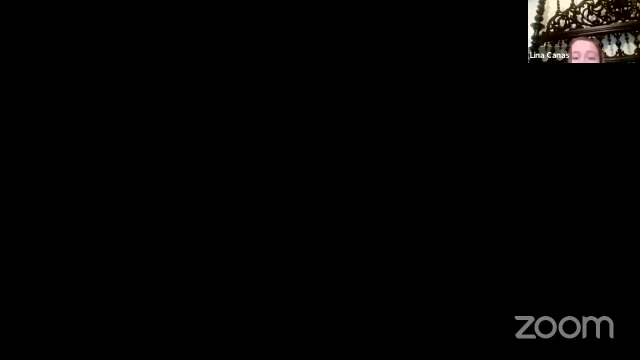 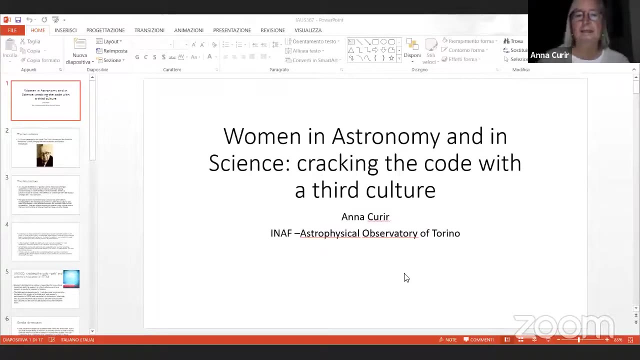 and in sciences, cracking the code with the third culture. Welcome, Anna, The floor is yours. Thank you, Thank you very much. Thank you very much to Beatrice and all the organizers for this beautiful and inspiring meeting. And do you see? 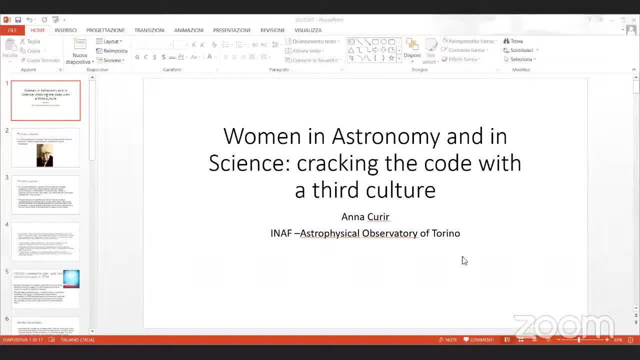 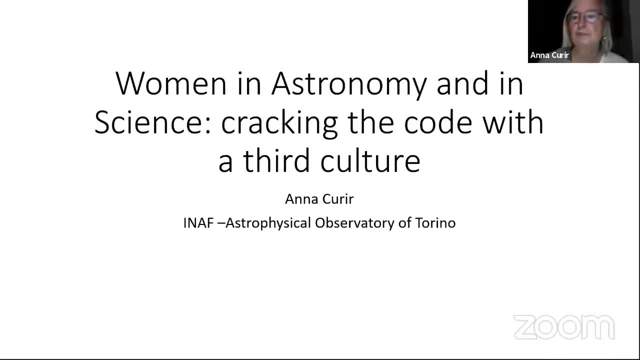 my presentation. Yes, Yes, You may go ahead. OK, So I would like to share with you and discuss with you a particular point of view about women in astronomy and in science, starting from the book that I think everybody knows by CP Snow. 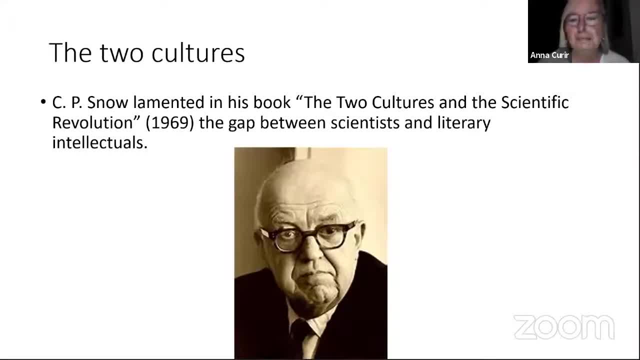 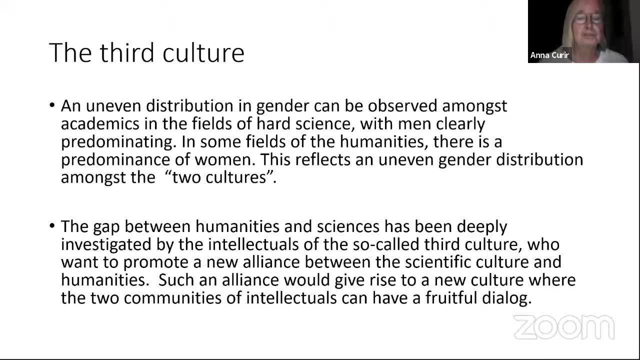 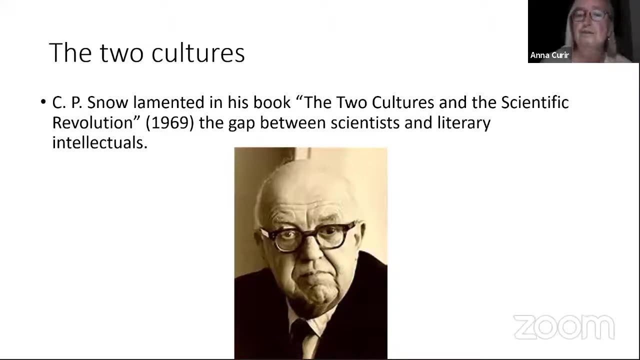 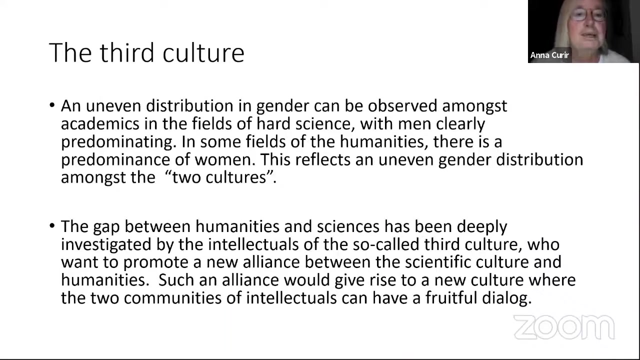 where he lamented the gap between scientists and literally intellectuals, And Snow was also proposing a third culture where the two communities have the possibility of speaking to each other. But we can also see an uneven distribution in gender amongst academics in the fields of science. 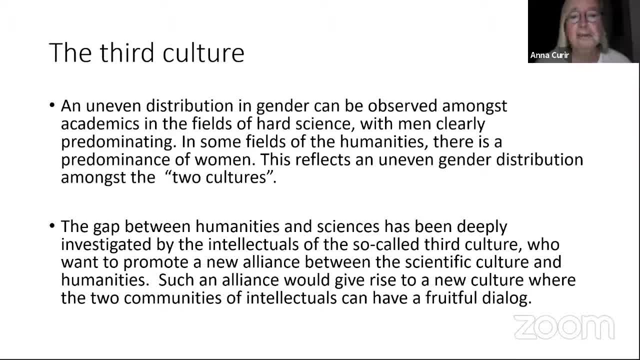 with men clearly predominating. In some fields of the humanities, there is a predominance of women, So there is an uneven gender distribution amongst the two cultures. The gap between humanities and science has been deeply investigated by the intellectuals of the so-called third culture. 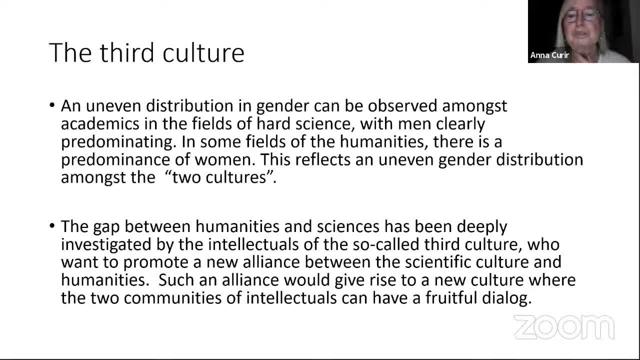 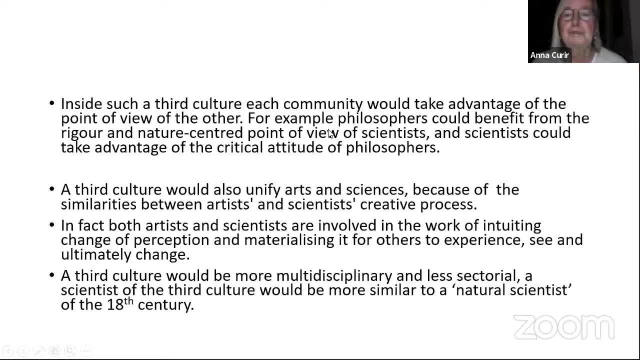 We want to promote a new alliance between the scientific culture and humanities. Such an alliance will give rise a new culture where the two communities of intellectuals can have a fruitful dialogue. Inside such a third culture, each community would take advantage of the point of view. 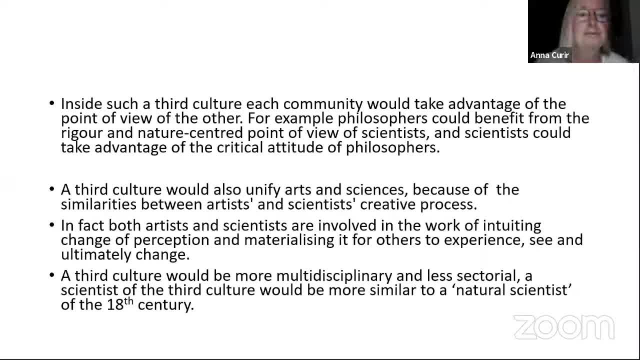 of the other. For example, philosophers could benefit of the rigor and nature centered point of view of scientists And scientists can take advantage of the critical attitude of philosophers. But a third culture would also unify arts and science, because the creative processes in arts and in science 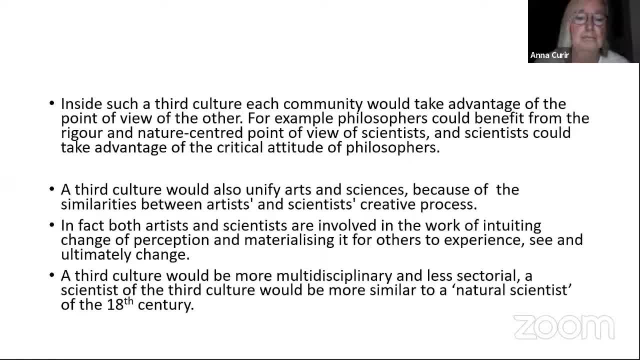 are basically the same because artists and scientists are involved in the work of intuiting change of perception and materializing it for others to experience, see and ultimately change. And a third culture would be more multidisciplinary and less sectorial, And in the document 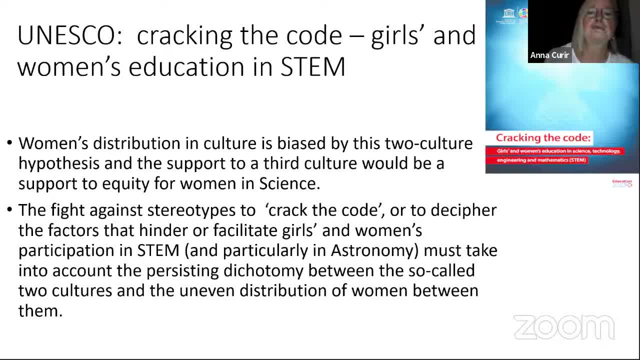 UNESCO document with the title Cracking the Code: Girls and Women's Education in STEM. it is a document that want to give the state of the art of the participation of women in STEM and promote action to improve the situation. And, as we said, 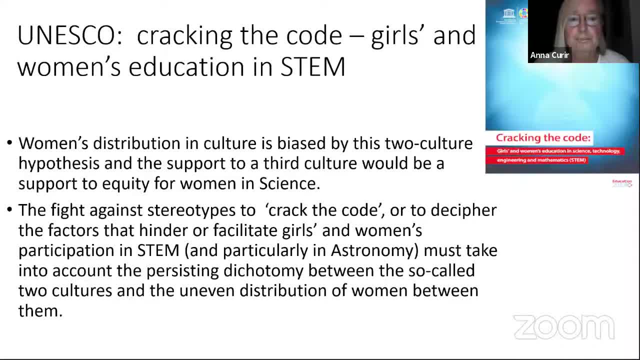 women's distribution is biased also by these two cultural hypotheses, And the support to a third culture would be a support to equity for women in science, The fight against stereotypes to crack the code or to decipher the factors that hinder or facilitate the girls' and women's 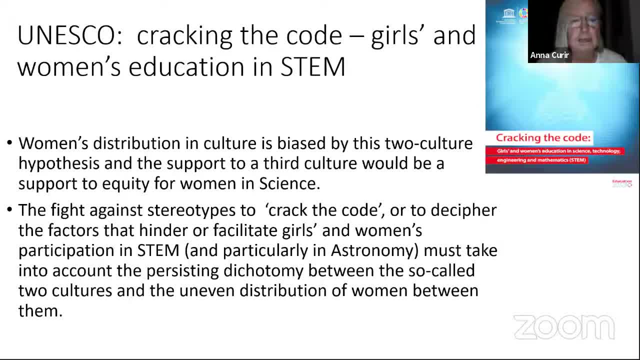 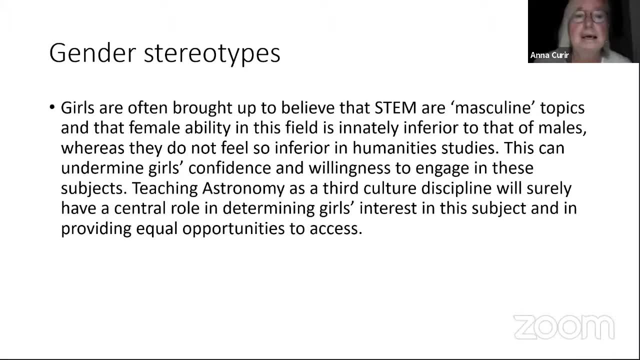 participation in STEM, and particularly in astronomy, must take into account the persistent dichotomy between the so-called two culture and the uneven distribution of women between them, Girls are often brought up to believe that STEM are masculine and that female ability in this field is innately inferior. 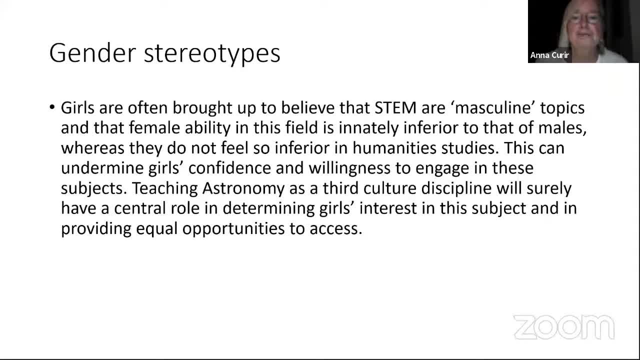 than that of men, Whereas they do not feel so inferior in humanities studies. This can undermine their confidence and willingness to engage in this subject. Teaching and structure of astronomy as a third culture discipline will have a central role in determining girls' interest in this subject. 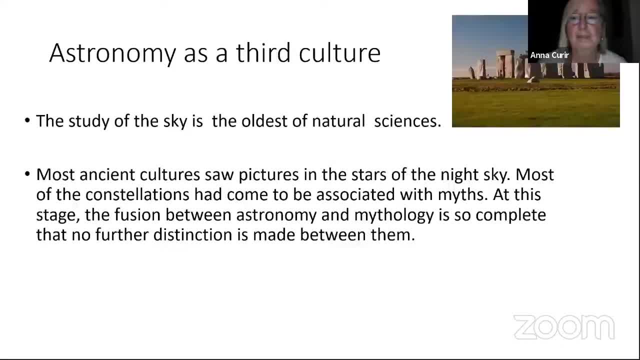 providing equal opportunities to access. But astronomy? if we think about astronomy, we can say that it is an old third culture, because in the ancient culture the fusion between astronomy and mythology is so complete that there is no distinction between them. So in ancient astronomy, 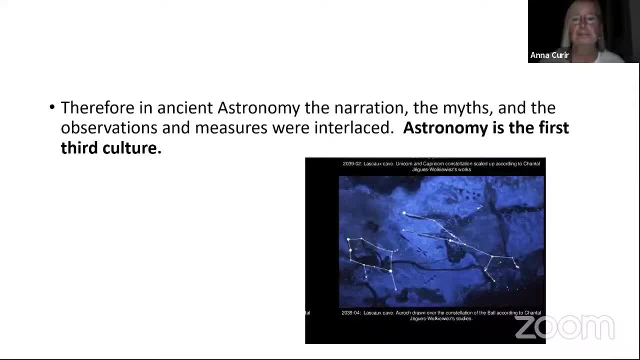 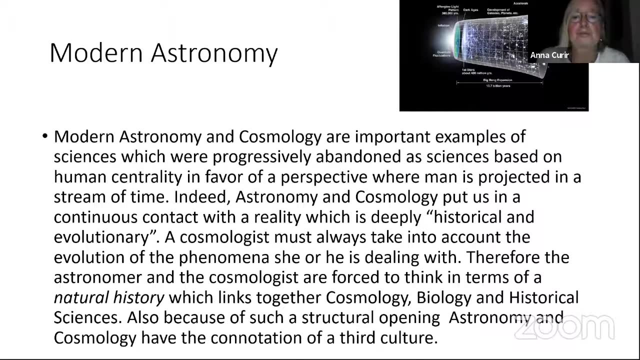 in a narration, the myth, and the observations and measures were interlaced. So we can really say that astronomy is the first third culture. But also modern astronomy and cosmology are important examples of sciences which were progressively abandoned as a science based on human centrality. 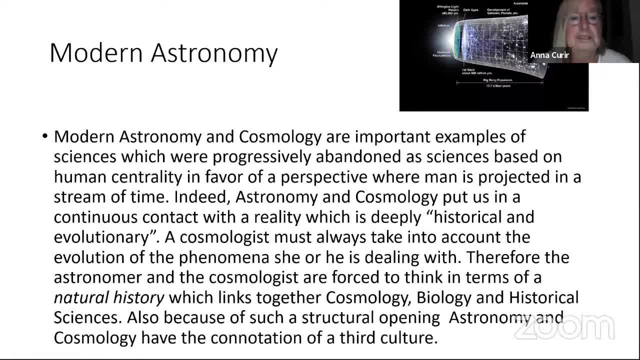 in favor of a perspective where the man is projected in a stream of time. Therefore, astronomers and cosmologists are forced to think in terms of natural history, which links together cosmology, biology, history and science, Also because of such a structural opening. 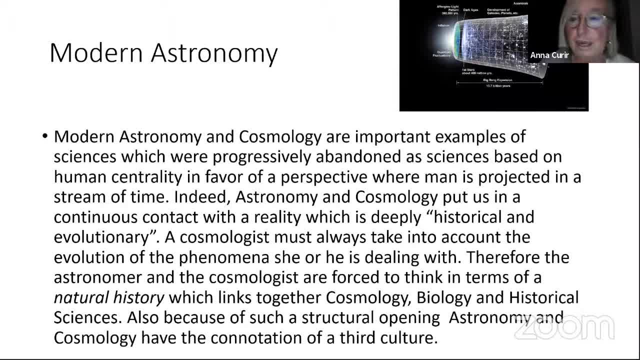 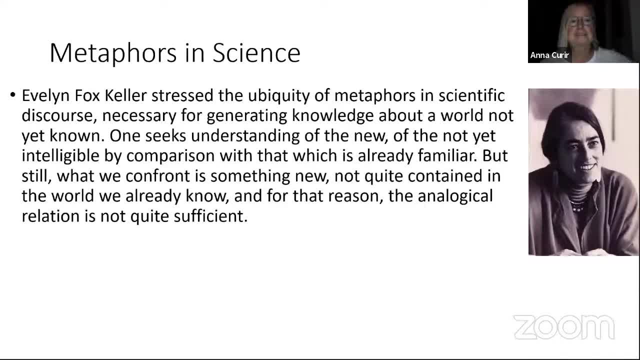 astronomy and cosmology have the connotation of a third culture. Eveline Fox Keller stressed the ubiquity of metaphors in scientific discourse necessary for generating knowledge about a world which is not yet known. One seeks understanding of the new by comparison with that which is already familiar. 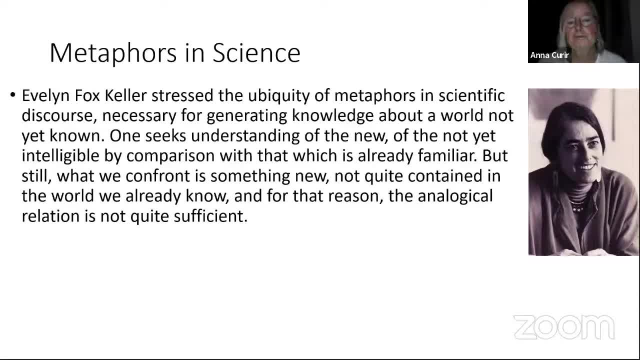 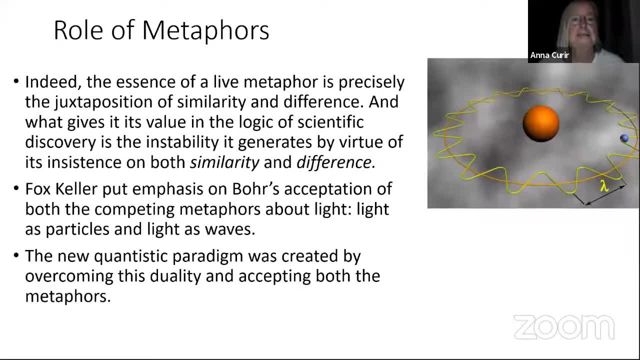 But still, what we confront is something new, not quite contained in the world we already know. Indeed, the idea of the essence of a life metaphor is precisely the juxtaposition of similarity and difference, And what gives its value in the logic of scientific discovery. 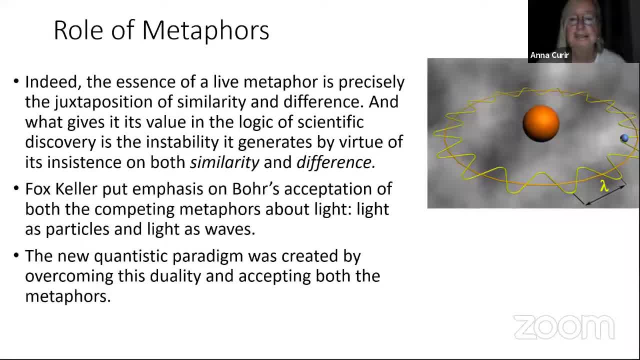 is precisely the instability it generates by virtue of its insistence of both: similarity, because we are in a world that we know, and the difference, because we are studying something new. Fox Keller put emphasis on more acceptation of both as a competing metaphors about light. 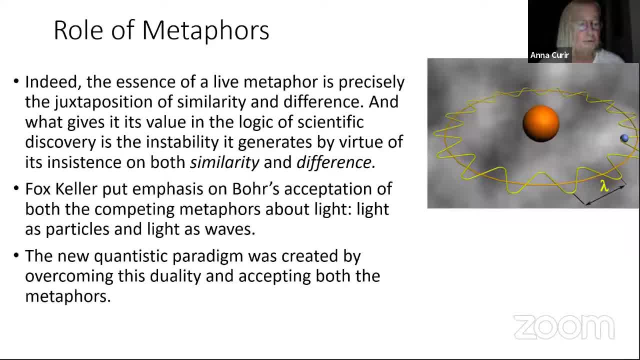 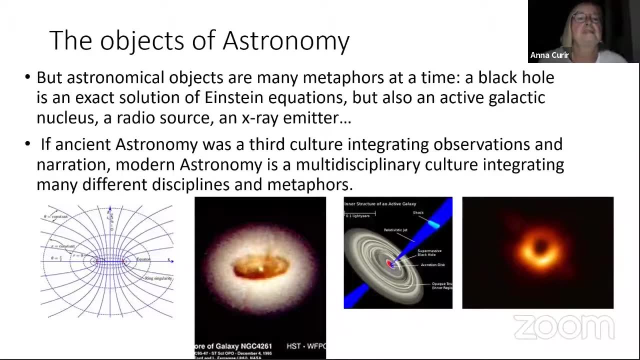 light as particles and light as waves, And the new quantistic paradigm was created by overcoming this duality and accepting both the metaphors. But the objects of astronomy are many metaphors at the time. A black hole, for example, is an exact solution. 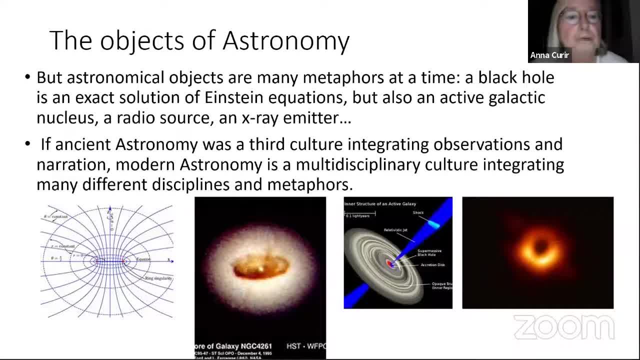 of Einstein's equation, but also an active galactic nucleus, a radio source, an x-ray emitter and a black hole, and so on. So if ancient astronomy was a third culture integrating observation and narration, modern astronomy is a multidisciplinary culture integrating. 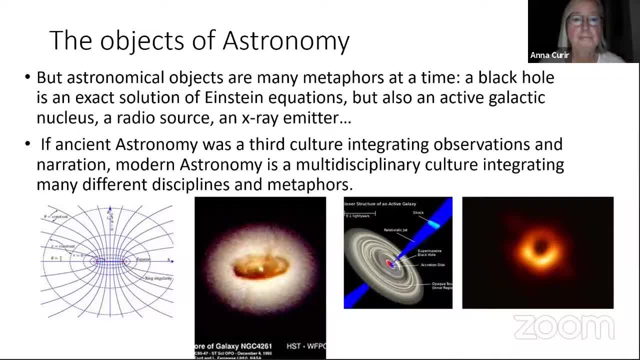 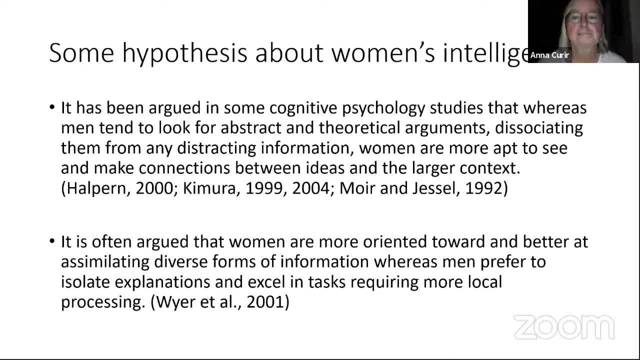 many different disciplines and metaphors. It has been argued in some cognitive psychological studies that, whereas men tend to look for abstract and theoretical argument, women are more apt to make a connection between ideas and larger context. It is often argued that women are more oriented. 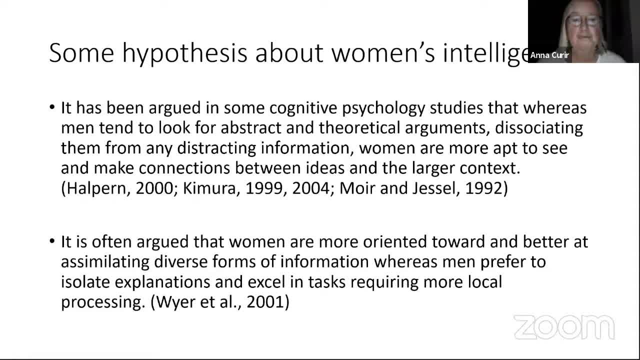 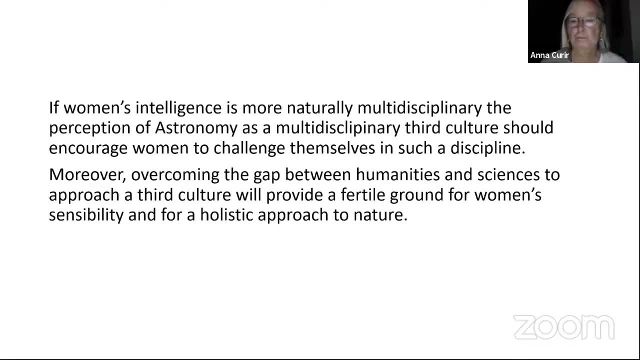 toward and better at assimilating diverse forms of information, whereas men prefer to isolate explanations and excel in tasks requiring more local processing. If women intelligence is more naturally important than information, then the perception of astronomy is a multidisciplinary culture. Third culture: 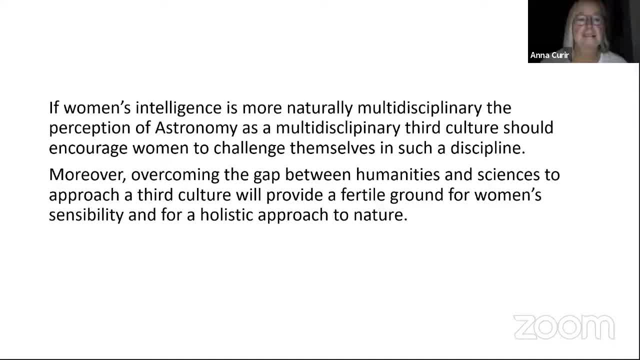 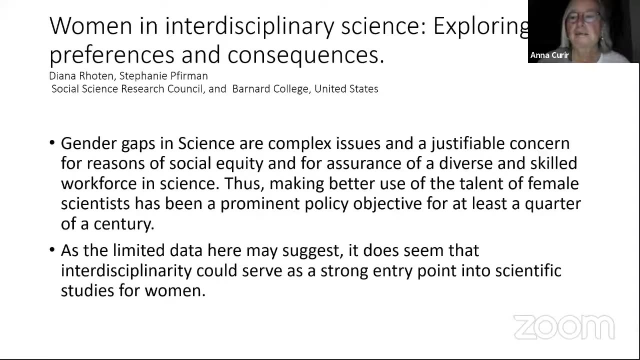 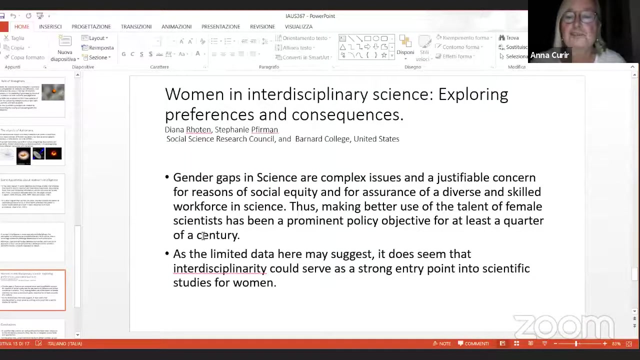 should encourage women to challenge themselves in such a discipline. Moreover, overcoming a gap between humanities and science- we approach a third culture- will provide a fertile ground for women in interdisciplinary science. They say at the end of the paper: gender gaps in science are complex. 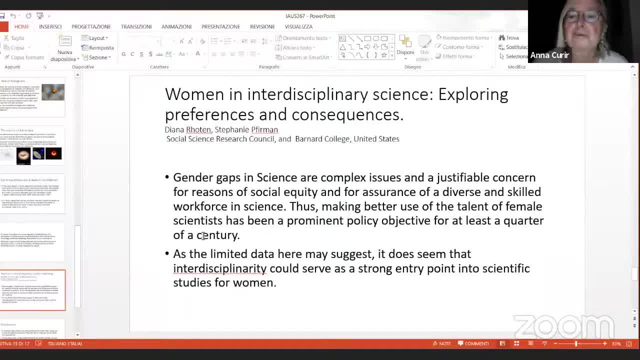 issues and justifiable concerns for the workforce in science. Thus making better use of the talent of female scientists, has been a prominent policy objective for at least a quarter of a century, As the limited data here may suggest. it does seem that interdisciplinarity 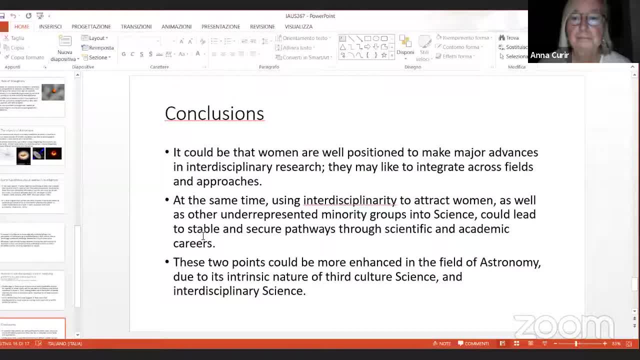 could serve as a strong entry point into scientific studies for women. So my conclusions are that women are well positioned to make major advances in interdisciplinary research. They may like to integrate across fields and approaches At the same time using interdisciplinary to attract women as well. 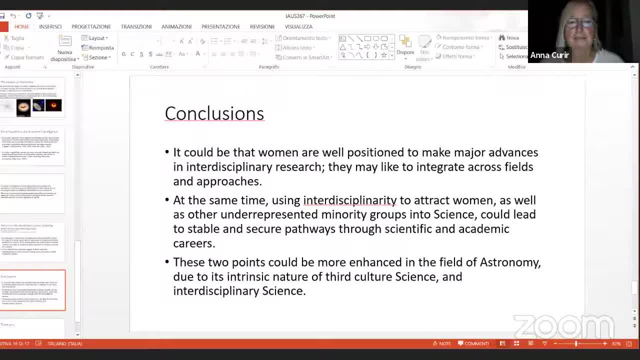 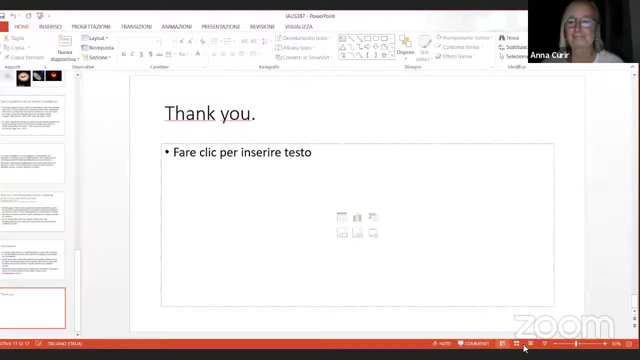 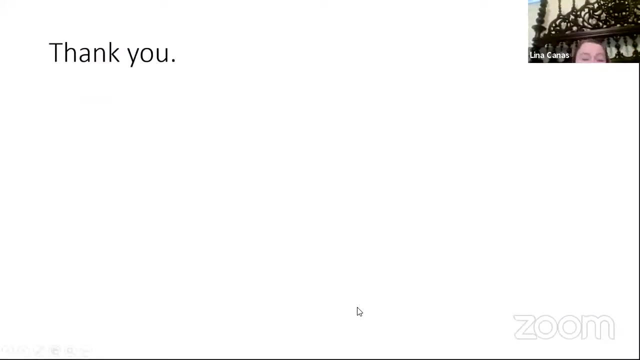 as other underrepresented minority groups into science, could lead to a stable and secure pathways through scientific and cultural science and interdisciplinary science. Thank you, Thank you so much, Ana, for the wonderful presentation And I apologize, We are really running out of time. 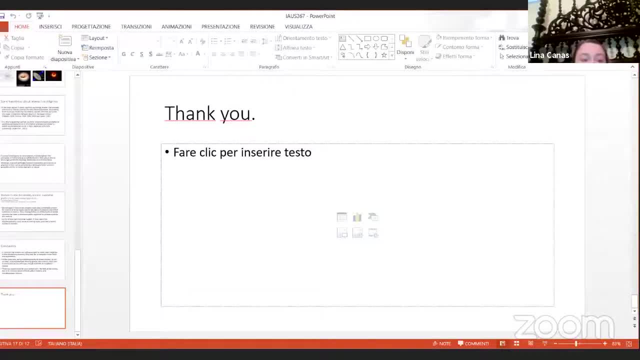 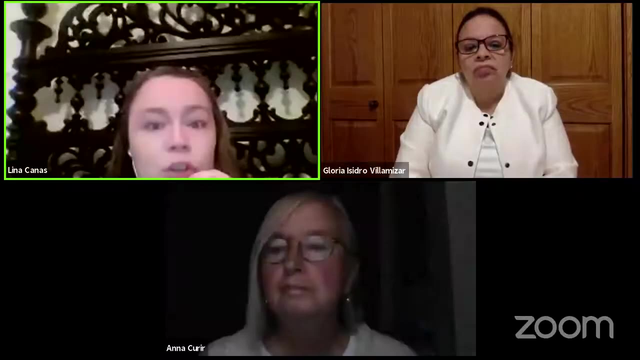 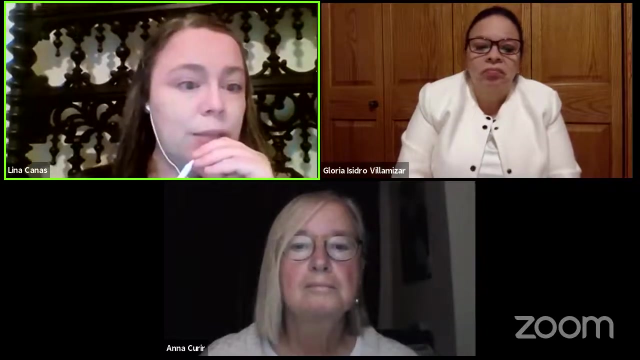 I want to thank all presenters for the wonderful presentations. We do have time to look into the chat and to try to answer as much or comment as much as you can. Here. we will have time for two questions, And the first one would go: 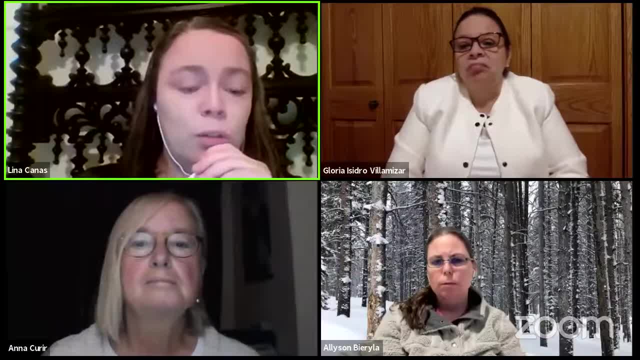 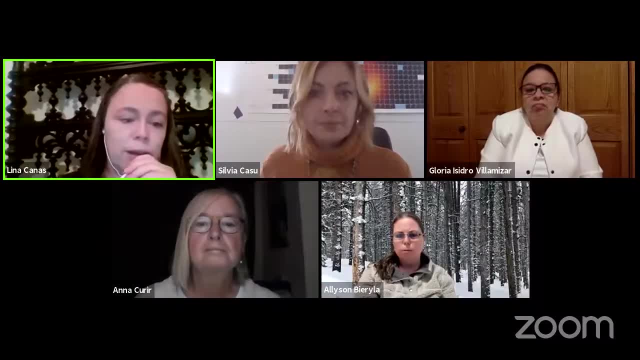 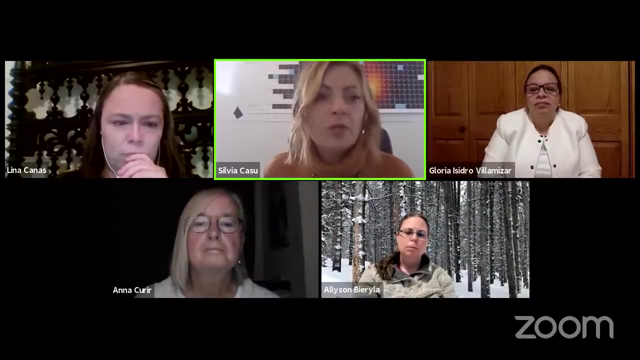 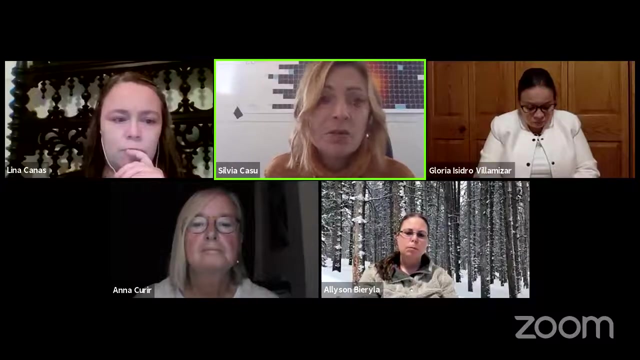 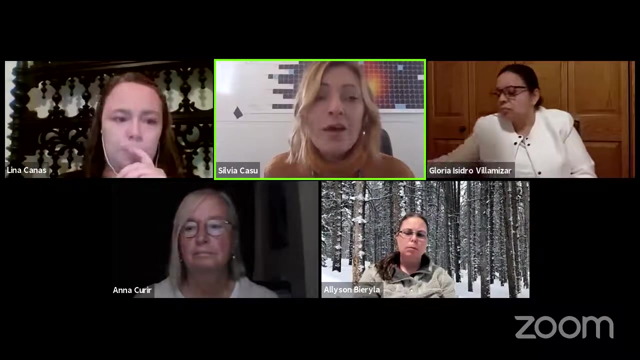 to my apologies, I'm just checking my notes. we have a question from Ugo that asks: what kind of inmates does the project work with? Well, we worked with 12 inmates, from 16 years old to 23 years old, So they. 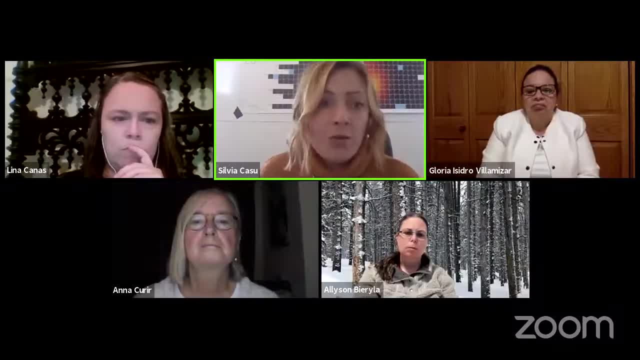 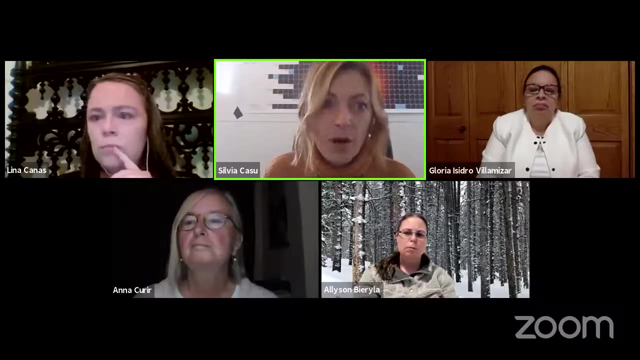 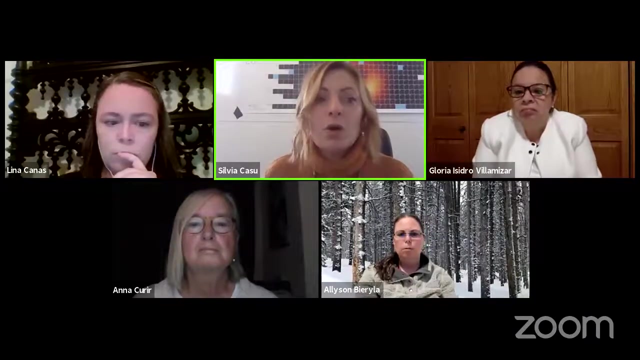 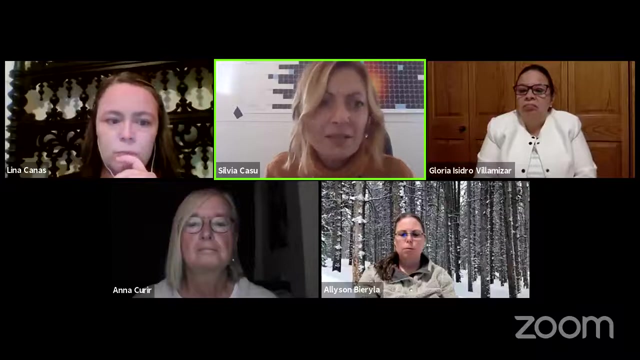 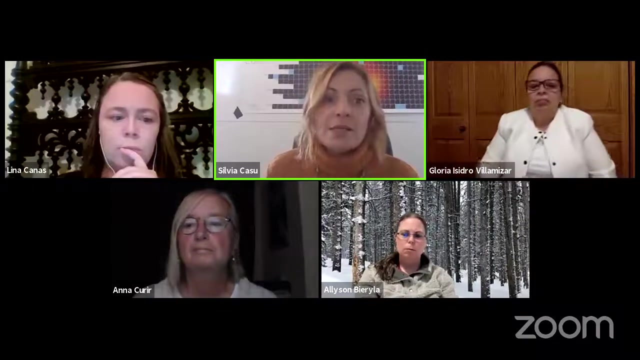 were very heterogeneous by age And they were very diverse from the age of 15 to the age of 30. And they were very diverse in terms of the age of the person. So this is a very different by their nation, one from Senegal. 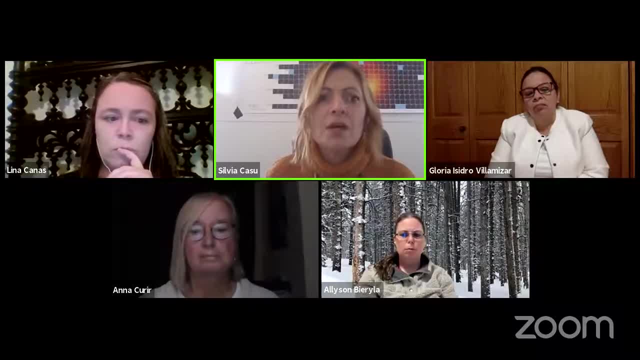 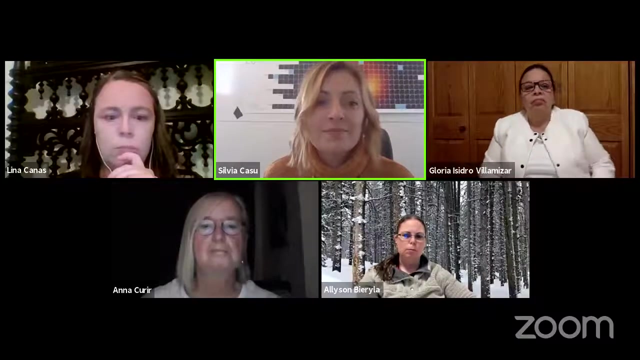 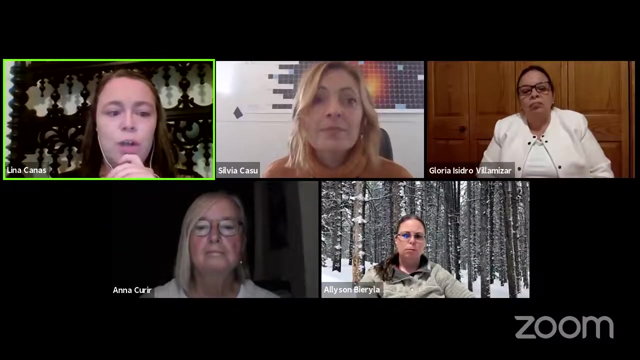 well, coming from Senegal, Egypt and Tunisia, Romania, Bosnia and all the other were from different parts of Italy, So they were very diverse in terms of the age of these people. Thank you, Silvia. And, as a follow-up: 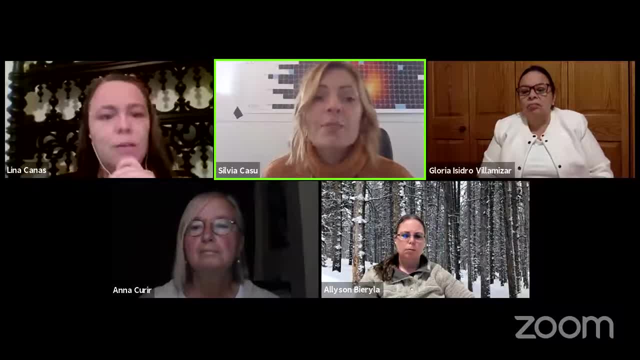 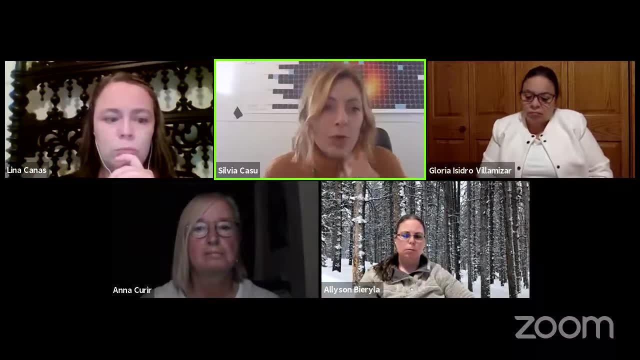 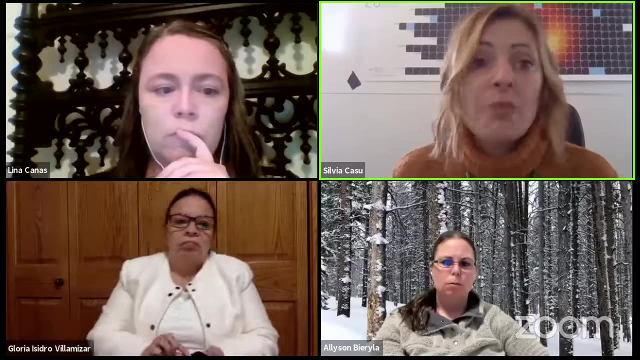 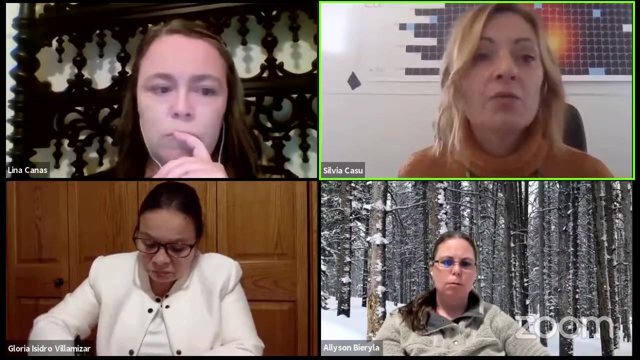 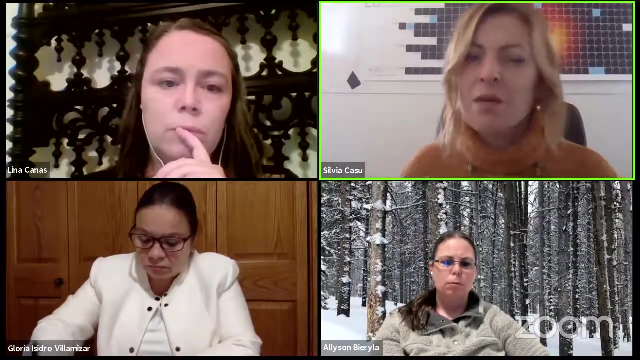 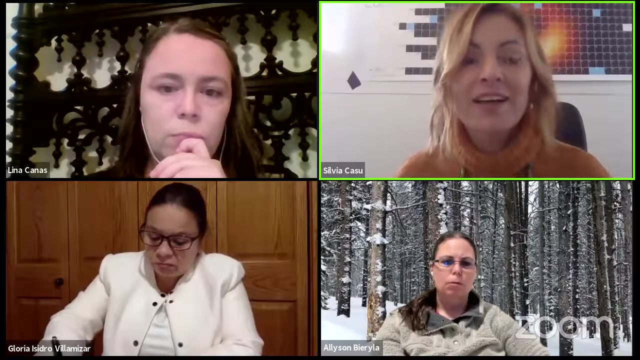 and I believe you already answered that. Jose Gomez asked what was the first thing you did to follow these activities. So at the very beginning they just stayed a couple of minutes and then just shake their shoulders and say hello, hi, and just. 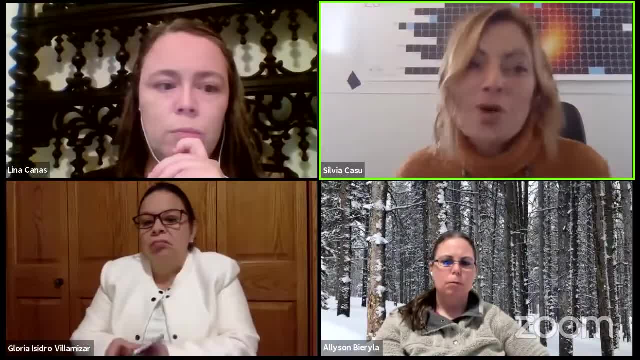 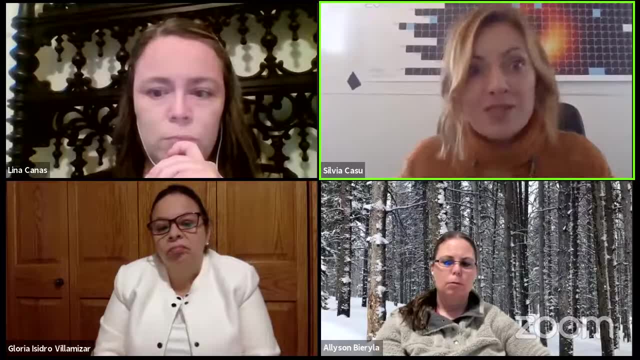 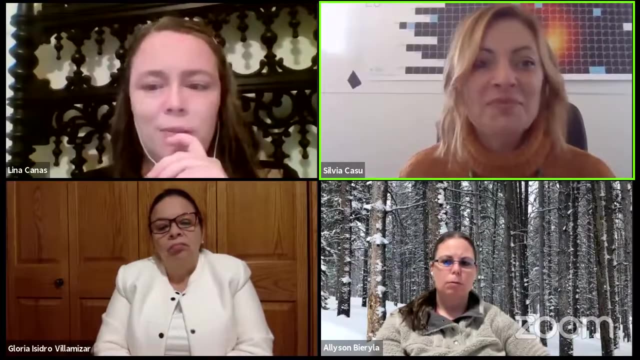 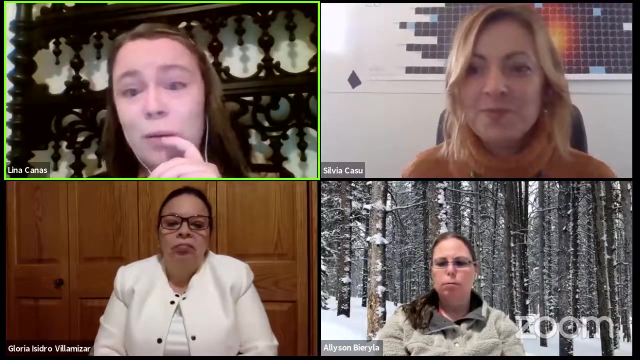 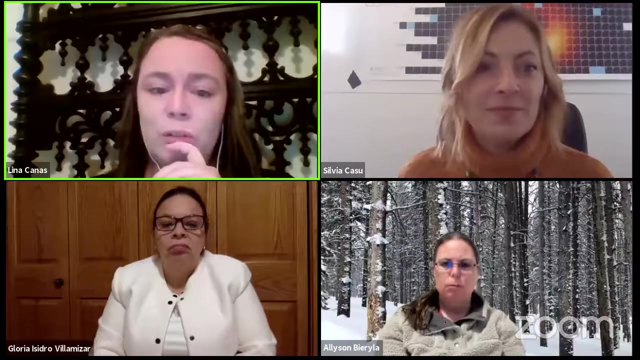 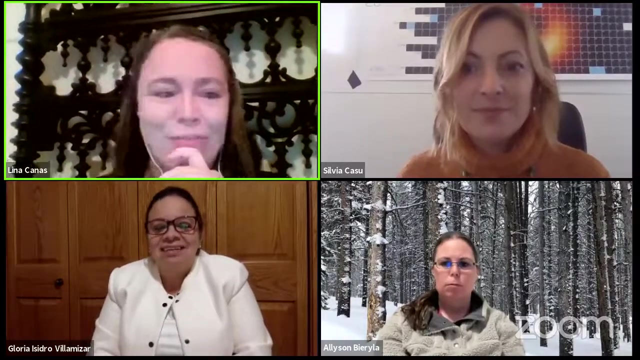 listen to them and wait and talk about all the things that I like to talk about. So transmit passion, transmit my feelings. Thank you, Silvia. Just for example, which spiral galaxy did you make the tactile model of? I believe you already. 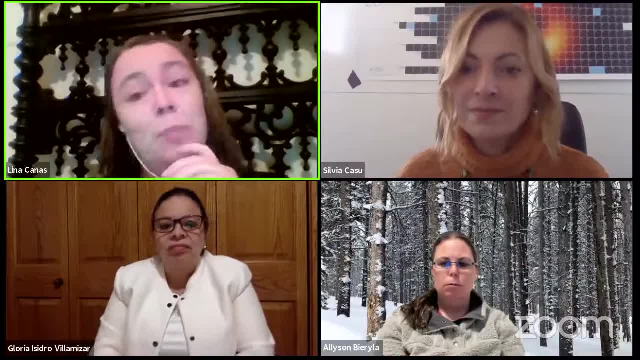 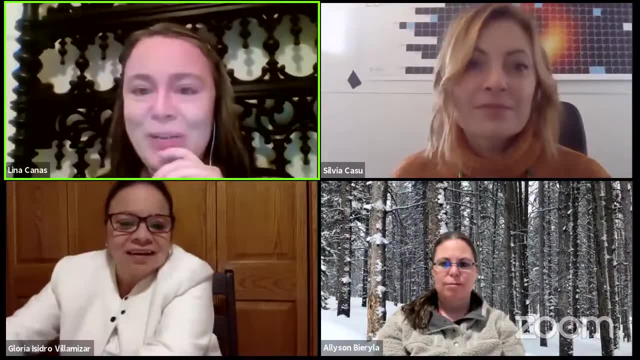 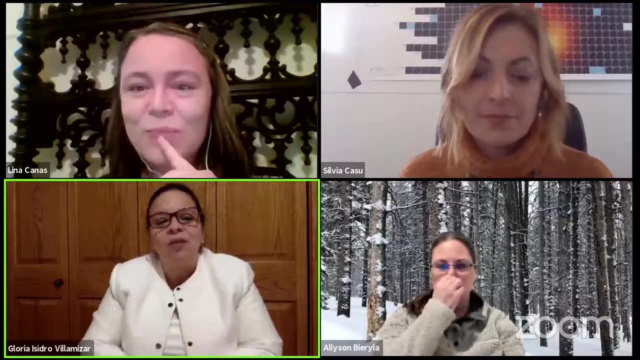 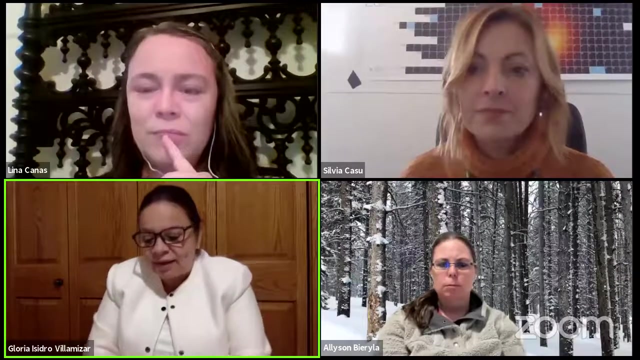 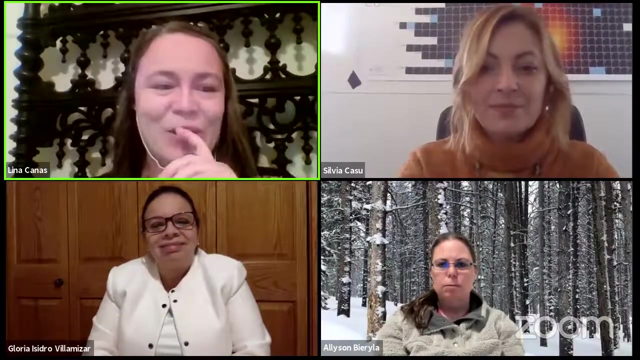 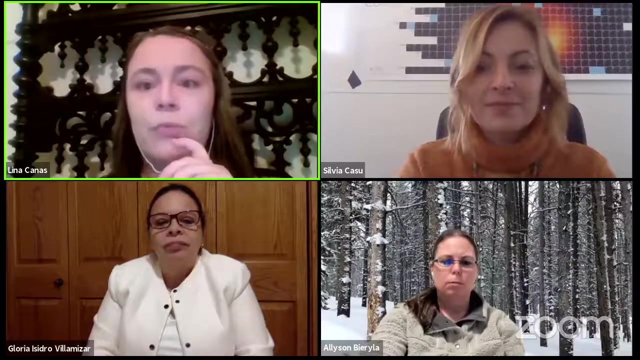 answered in the chat and I appreciate it. I just wanted to share a little bit with you about the images of NASA. For the spiral galaxy, we use the image of NASA, the NGC 1232.. Thank you, Gloria, For. 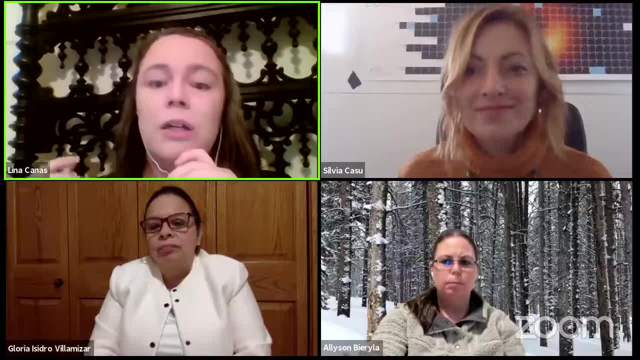 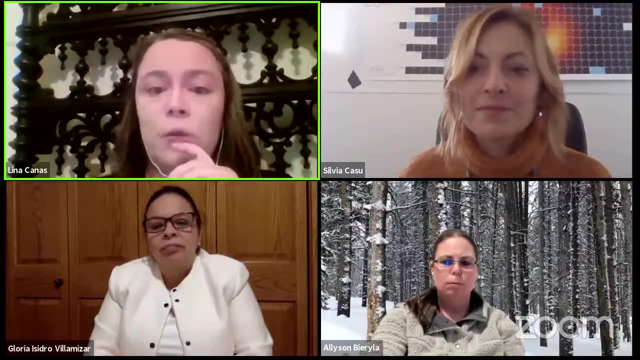 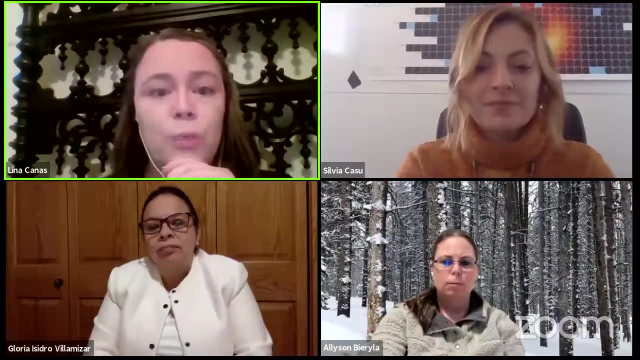 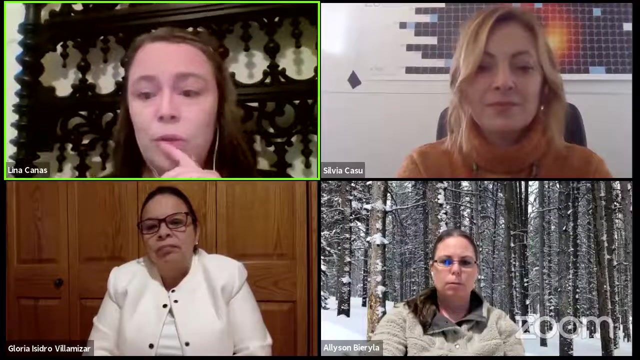 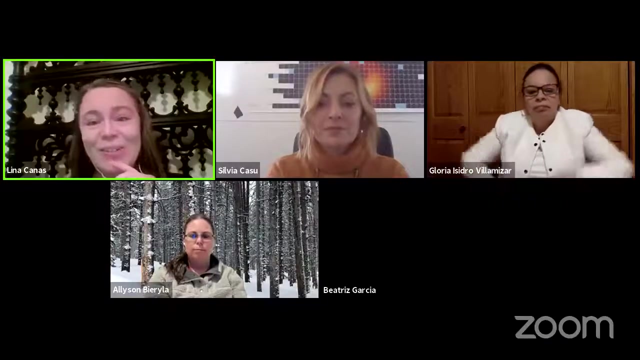 our colleague Alison. there's a lot of information in the chat. Where can we find further information? And also to Pauline, I apologize, There are these questions that Alison already answered. You can look into the chat for more information. Thank, 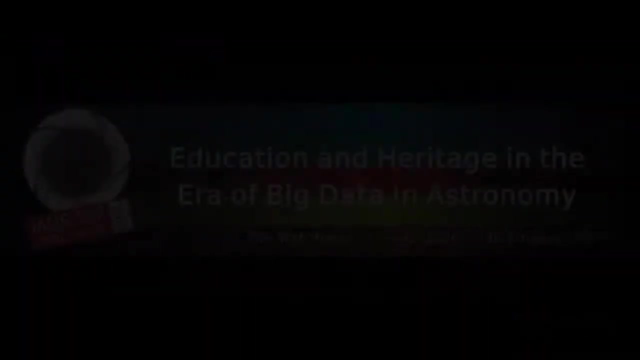 you so much. You are wonderful. The work you've been doing is very valuable.